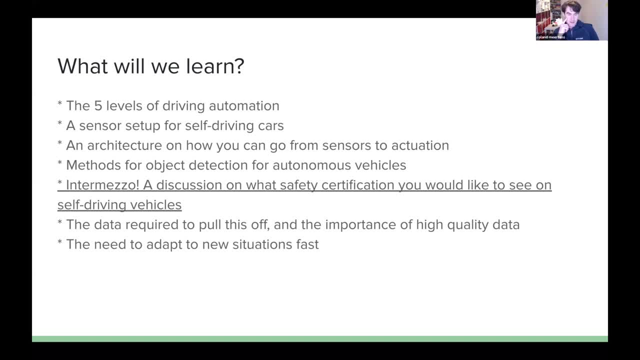 of autonomous vehicles. So that's five levels of driving automation: what kind of sensors are used for self-driving cars, What kind of the architectures are in terms of what components are there in the self-driving car stack, And then go over four really basic methods for object detection for autonomous. 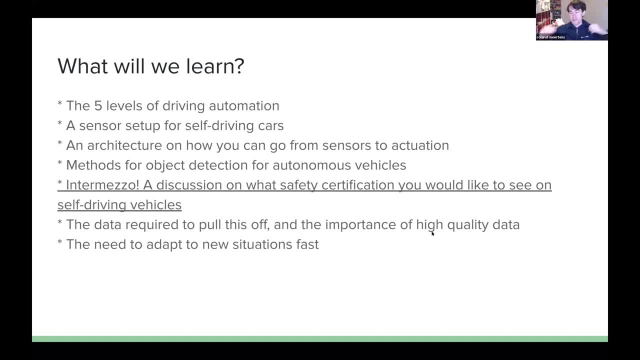 vehicles. And then I figured that we could do something interactive. So normally if you are doing a meetup it's just you listen to some guy talking and then, I don't know, after half an hour I start being distracted and start doing something else. So I figured 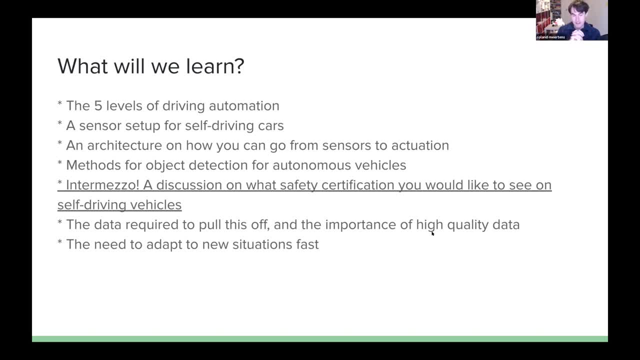 that after half an hour we can do like an intermezzo and can have a bit of a discussion on what you, as a participant in the meetup, think is important for the safety certification on self-driving vehicles. Right, So if you want to- I don't know- import a toy into the EU, you have to show that it's. 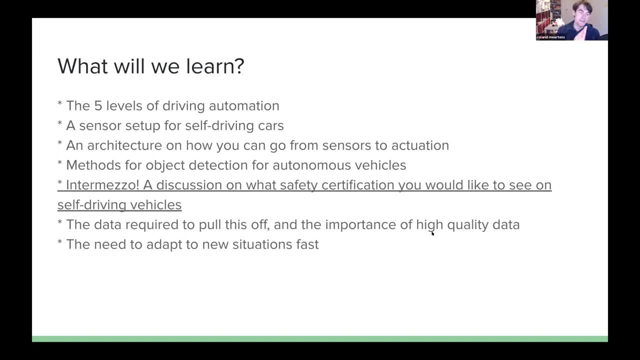 not poisonous for children. So if we have self-driving cars, whether you as a consumer or a person on the streets want to see has been certified about this car before we allow it on the street. So if you can already start thinking about that, that would be great, Or be prepared to turn. 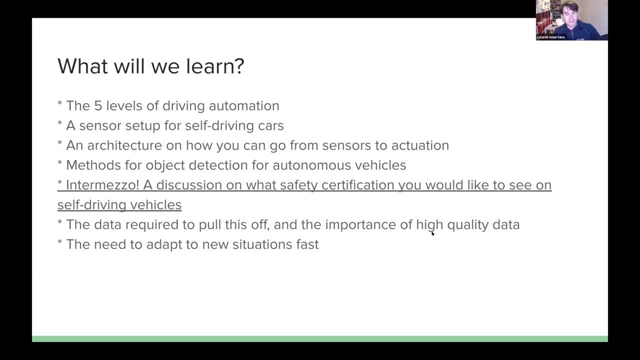 on your webcam and your microphone so we can have discussion. That would be nice And after we do that I will tell a bit more about kind of the data required to train self-driving cars and the importance of high quality data for training and validation. 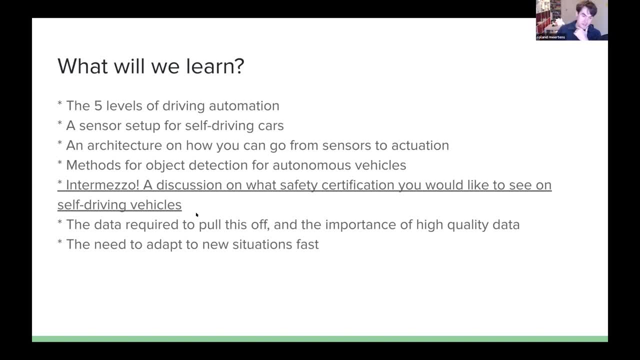 So we will come back there to proposals you made during this intermezzo, And then at the end I'll have a short talk about why self-driving cars need to be able to adapt to self-driving situations or to new situations. So the first thing is actually really exciting, because there's different types of self-driving. 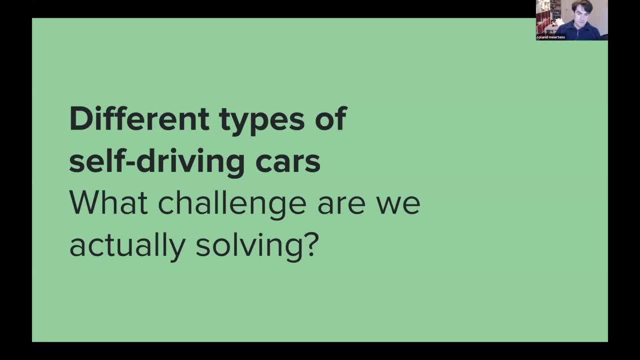 cars So often in media. everyone talks about self-driving cars, and it's one thing, but actually there's multiple types of self-driving cars, So I'm going to talk about that in a bit. So, first of all, self-driving cars are a very common challenge And this has been changed. 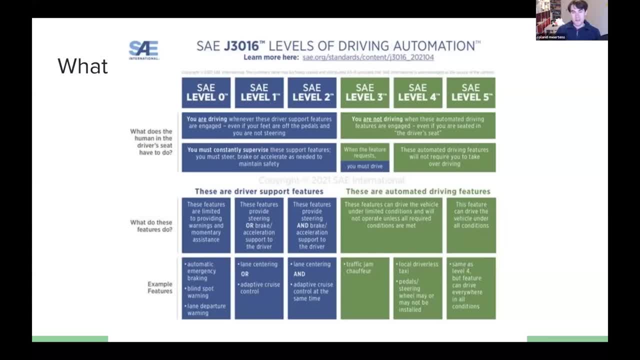 last week. So last week they defined the levels of self-driving vehicles a bit better. but there's a big difference between the self-driving level zero, which is no support at all for your self-driving, for your car, all the way to level five, which means you have a self-driving car which completely 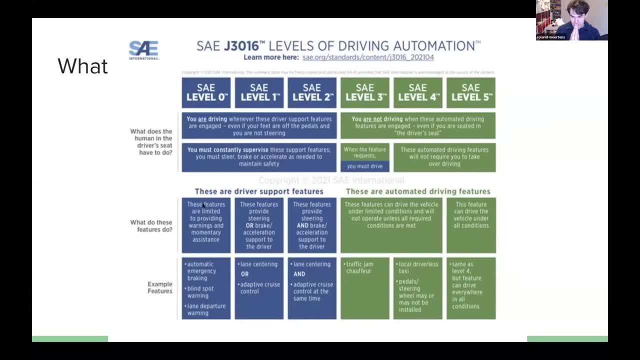 drives itself. You are not needed anymore And it can drive whenever and everywhere. And there's a big, maybe important, split here between level two, where there is support for steering and braking and acceleration, everything such as, for example, keeping the car, 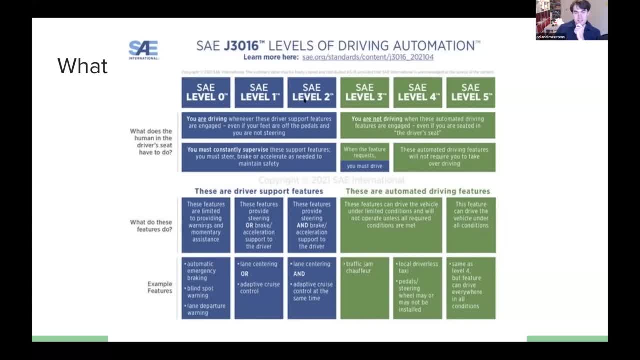 in the center of the lane or adaptive cruise control. But it's really important that in level two, you, as in, if you buy the car and you're driving this, you are still driving and you are still responsible and you are still 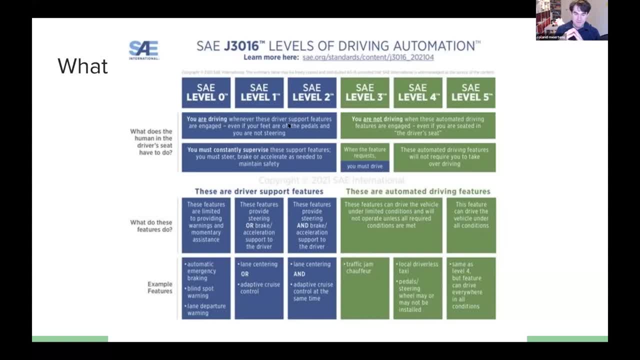 you still have to make sure that the car is safe. You must constantly kind of supervise it. You have to keep a look at, okay, what's what's the car doing. And then there's level three, from where you're not responsible anymore. You can go read a book, et cetera, et cetera. And 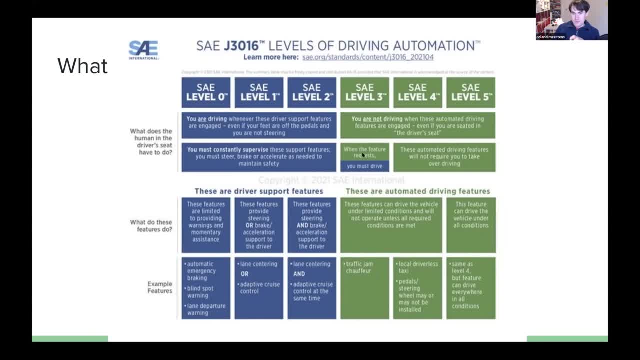 the difference between level three self-driving, where you're maybe not driving anymore, but sometimes the car might say, oh, I don't know what to do anymore, And then you must take over. So in level three and four there are basically limited conditions and limited circumstances. 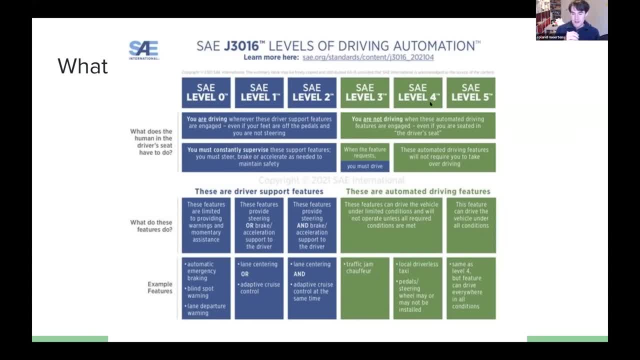 in which you can drive. So think about limited- limited to specific highways or limited to the traffic jam, for example. And in level four, there's already never any moment where you have to intervene with a car and get in the car or get behind the steering. 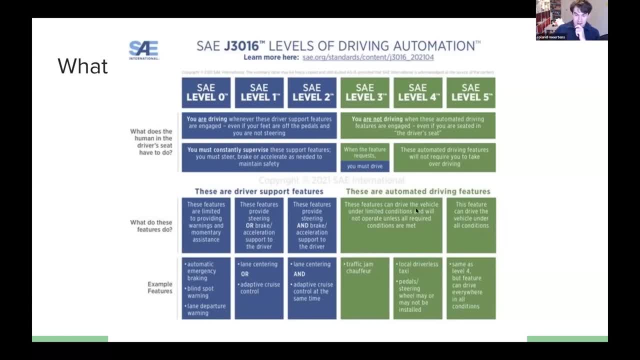 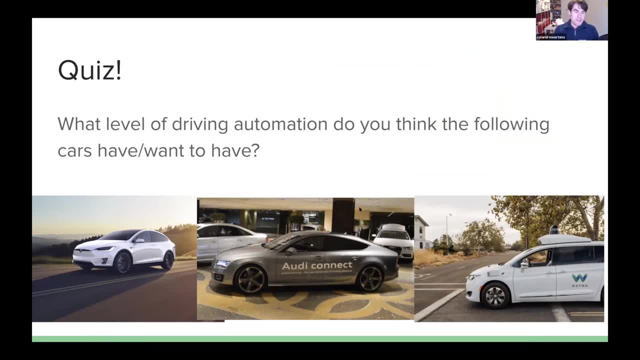 wheel to take over. So after we hear this, I've got a quiz. Yeah, Okay, I can't control my slides, It's good. So for the people who are listening, what level of driving automation do you think the following car following cars have or want to have? So let's first start with a Tesla. 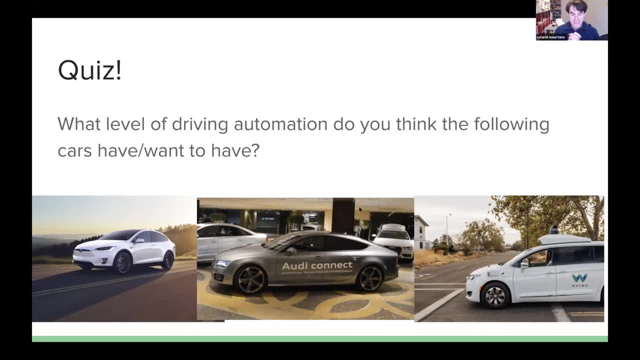 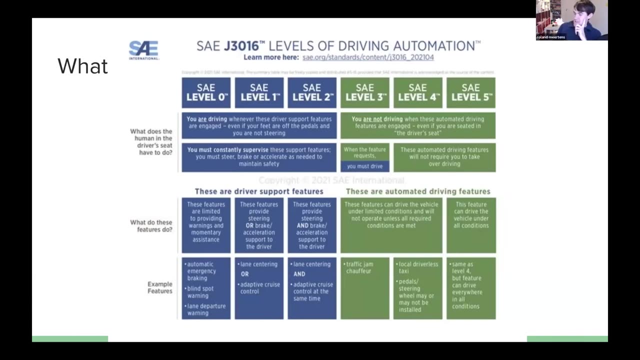 Elon Musk says: oh, it says full self-driving capabilities. That's what they sell in the media. What level do you think a Tesla has? Should we use chat for this, or do we want to? Oh, what we can do is, I don't know, do people mind turning the webcam on, or is that like super? 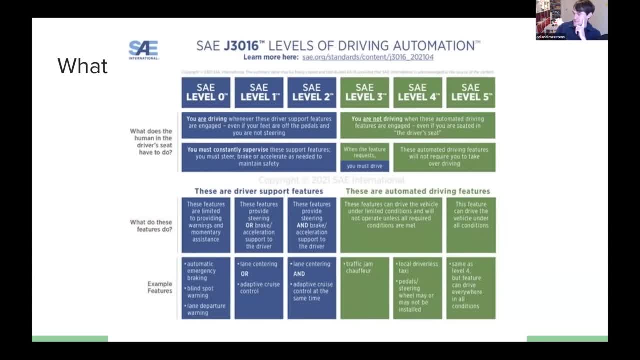 awkward now Are people like standing in their pajamas. I don't know. I can allow everybody to unmute themselves. if you want, It's up to you. Yeah, What we can do. it's also hard Like I'm trying to get a good view on everybody. 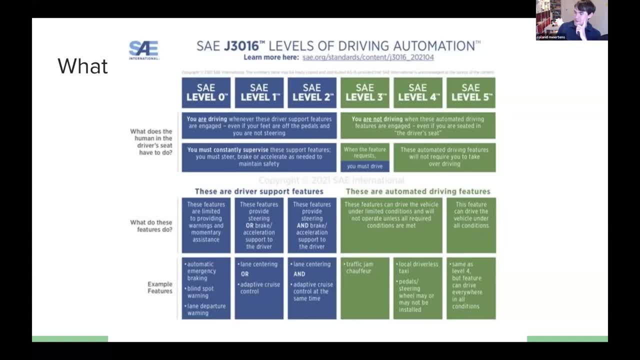 but I'm struggling with my window. Oh, now I got it, I can actually see people- Great. Also, my screen with people is on my right, my webcam, So I look like I'm looking away. So what we can do is do finger voting So people can just show. I mean, there's five levels, There's 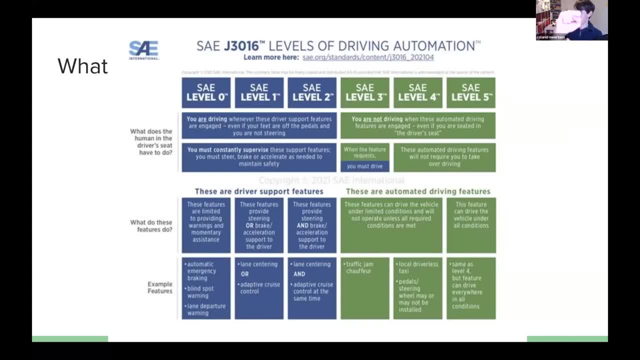 five fingers. It's easy, right? So people can just show their fist and then we just count down and three, two, one, And then you show what level you think a Tesla has. Three, two, one, I see. two times two, I see. 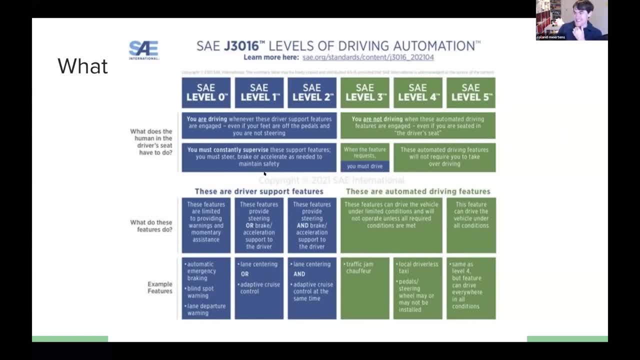 three, All right. So the right answer is indeed two. So the Tesla supports steering and braking and acceleration, But there's never a moment in a Tesla right now that you can look away or take your eyes off the road or start reading a book, So you always have to. 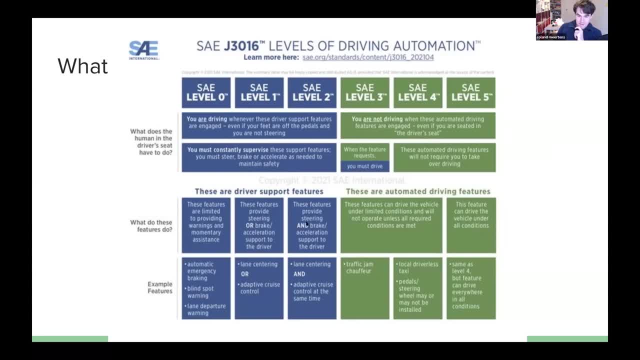 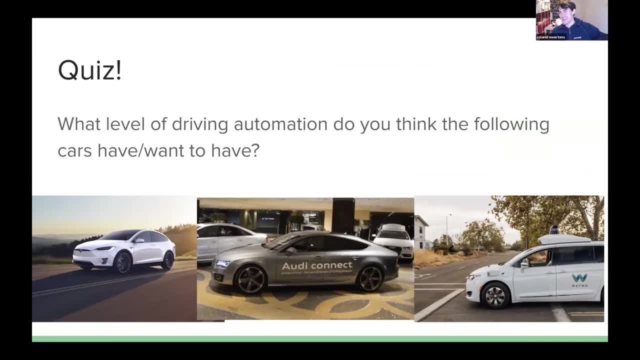 Be invested in driving. But if we go to the next car, there's the Audi A8. And the Audi A8, when it was released, they said this car will have a traffic jam pilot And if you get into a traffic jam, the car will steer itself and you can just relax. And as soon as you get out of the 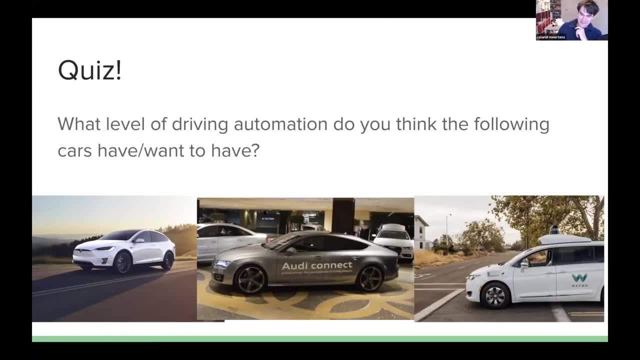 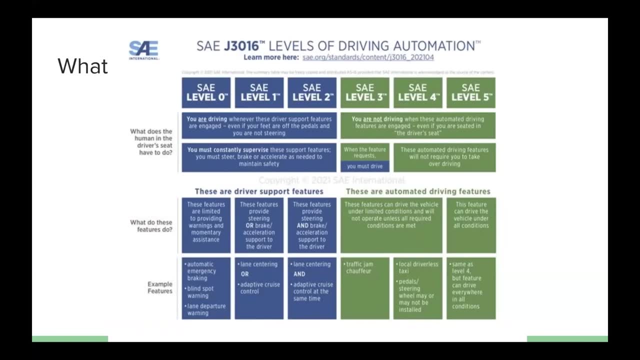 traffic jam, the car will beep and you have to take over again. What level do you think Let's do the same? Thumb finger hand voting again Three, two, one- I see one, two and two. Yeah, no, So actually. 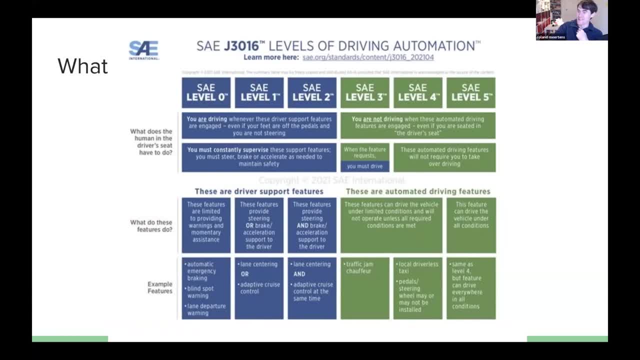 in this case it's a bit awkward for Audi because I think the feature never released, But the plan was. what they wanted to have was a level three system where you would really drive into the traffic jam and the control would start showing movies or something. You didn't have to pay any. 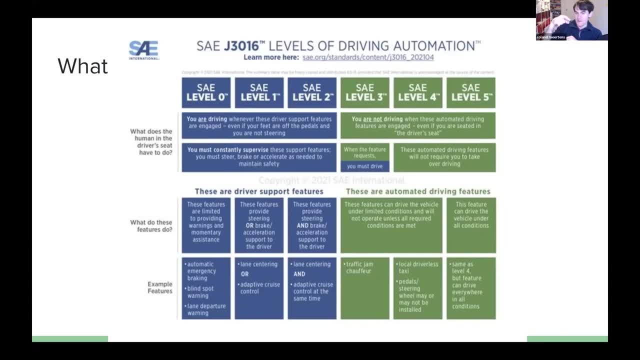 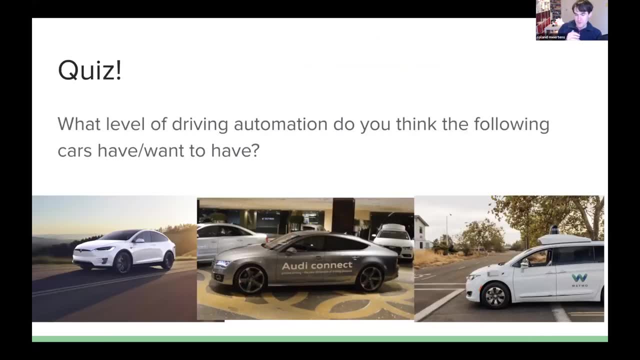 attention at all. But it's really this really local thing where, Where Audi would basically be responsible for any accident, The car would be responsible, And then we've got the Waymo vehicle. You'll already see there's no driver behind the steering wheel, So 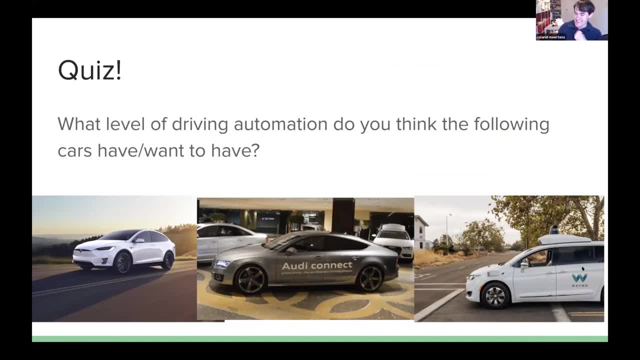 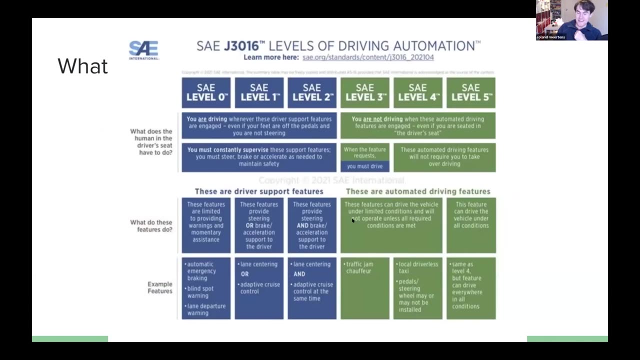 that's the hint. What level do you think the Waymo vehicles have? Let's count down again: Three, two, one. I see level three, three, three and four. So the right answer is that Waymo is level four. 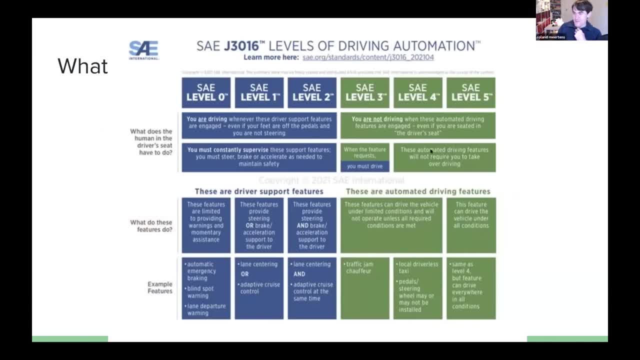 So Waymo is really going for a fully autonomous vehicle which is only at only like a local driverless taxi. I don't know if you can see my cursor, by the way. So it's only a local driverless taxi, But you, as a passenger, will never have to take over the steering wheel. The car should be. 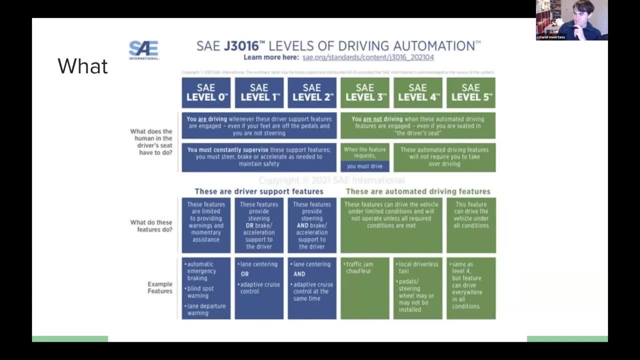 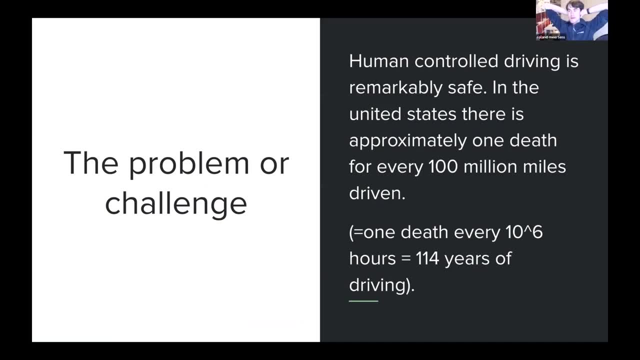 able to handle that all himself. So those are levels. So now the problem or the challenge with autonomous driving. So people always say, oh, there's so many accidents in traffic, which is true And it's really terrible, But it's a really hard problem. 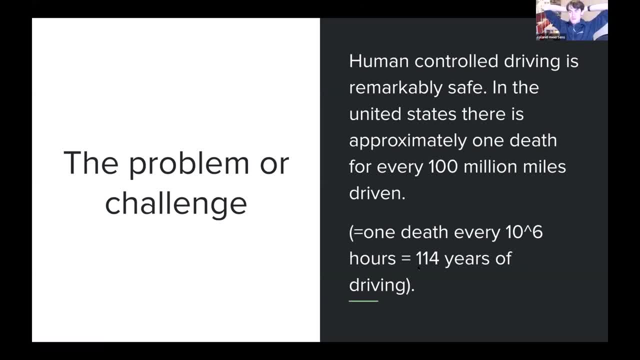 to automate. even though humans are not amazing at driving, Human controlled driving is really big, Maybe mute again. by the way, I'm hearing some rustling. So in the United States there's maybe one death for every 100 million miles driven. 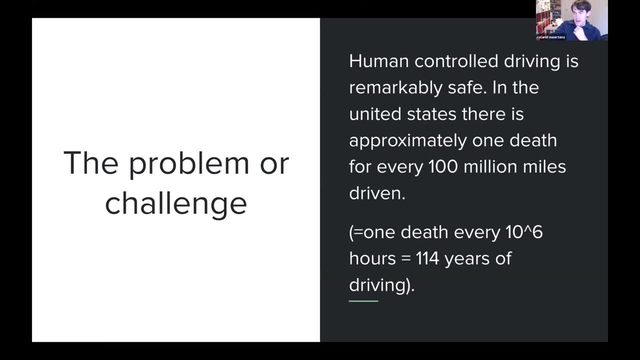 That means that there's one accident or one accident with a death ending every 114 years of driving, or every 10 to the power six hours. Fun fact, by the way, If you guys are able to fly a plane again, a plane is a thousand times more kind of like safe against wings falling off. So 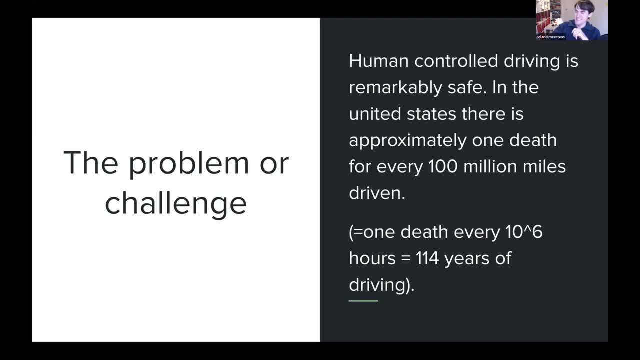 So every 114,000 years of flying, a plane loses its wings spontaneously. But this is kind of the safety we are looking at for transport, which is really safe. If you look back at programs you've written yourself, it happens pretty. yeah, like this is kind of safety you really have to get to. 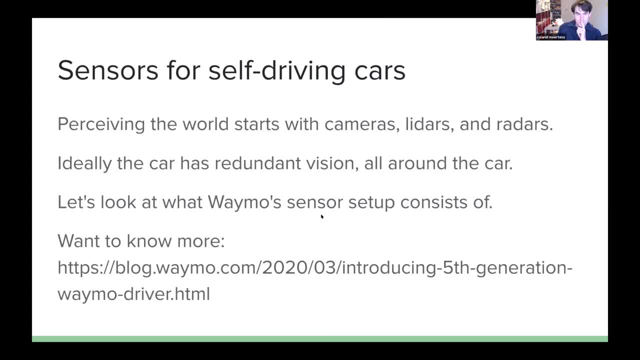 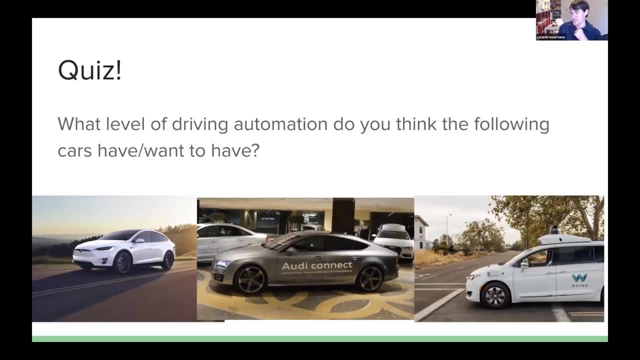 So for the sensors self-driving cars, have I already showed you the Waymo vehicle here. So the sensors of self-driving cars have to determine where can I drive, what decisions can I make. Those are lidars, which you can see here, cameras which are all around the vehicle, and radars. 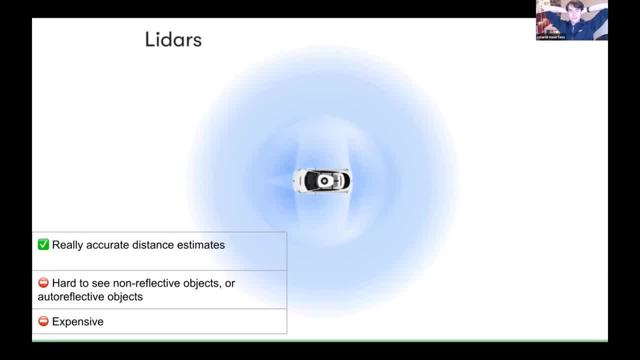 So I want to quickly go over. especially nowadays, People are saying, oh, Elon Musk is saying, oh, there's no need for a lidar, or there's no need for radar. Every one of these sensors actually has big merits and reasons. you want to use them. 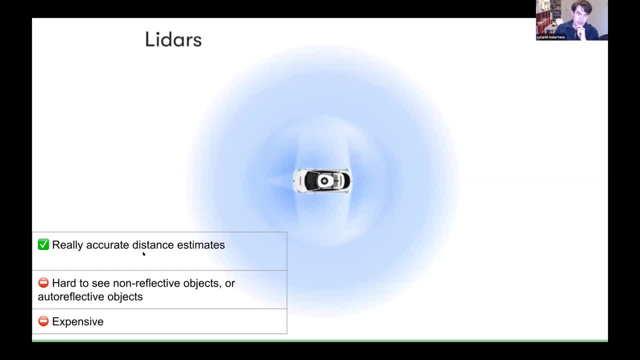 So lidars are really great because they have really accurate distance estimates. So those are centimeter accurate. You know exactly where objects are around you. It's a really nice sensor for that, But there's also a downside. So, for example, if you have non-reflective objects, 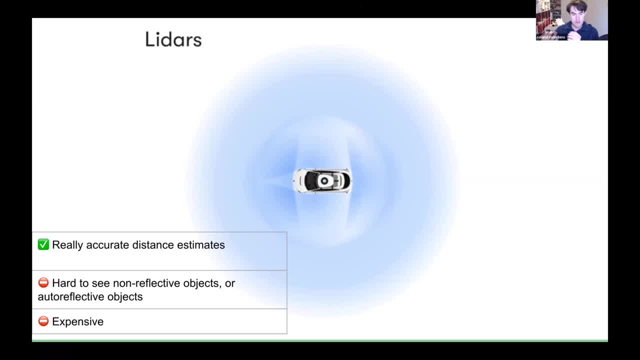 Like really black cars or outer reflective objects like traffic signs. they tend to cause a bit of blooming- or non-reflective objects don't return any lidar information. So then you don't see your specific object anymore And lidars are also currently expensive. but you can see that Waymo likes lidar so much that they've put one big spinning one for long range lidar in the middle. 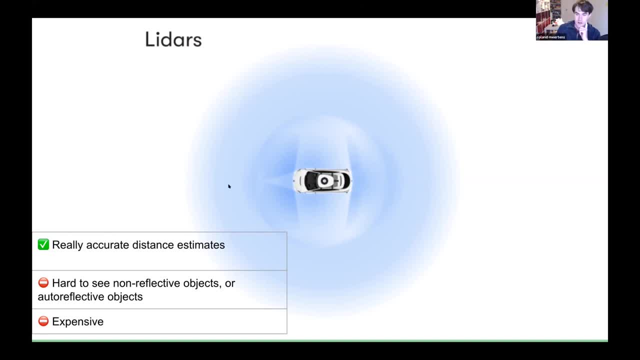 So this was sent up to 200 or 250 meters away And they also added one, two, three, four. And they also added one, two, three, four lidars on the sides to catch any pedestrians or any small things which are closer to the car. 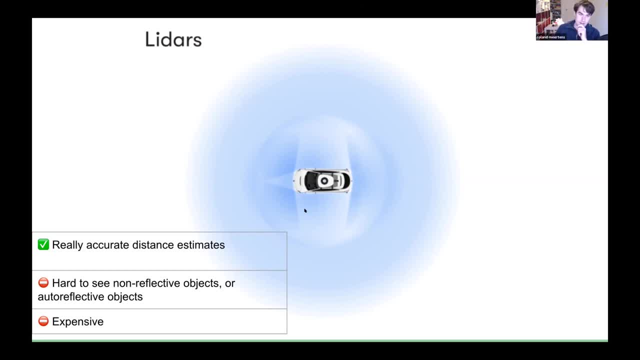 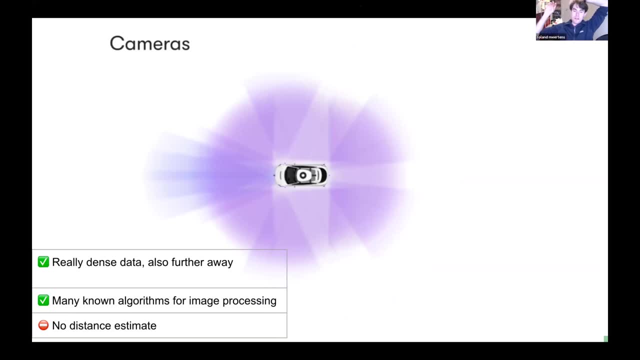 So they have complete 360 degree coverage of their car. They've also got radar sorry cameras. So if you look at a laser scanner, like with lidars, they're always spinning right. So that means that you only shoot a laser beam every X angle. 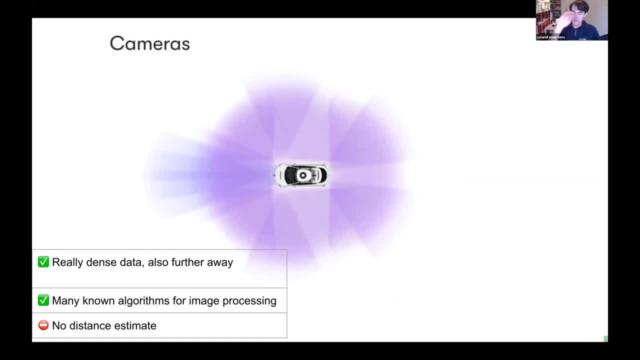 But it means that farther away you don't have that many lidar returns anymore for objects. So if you have an object which is maybe 200 or 150 meters away, there's maybe- I don't know- eight or five or 10 lidar points. you get back from the object and you don't really know what it is. 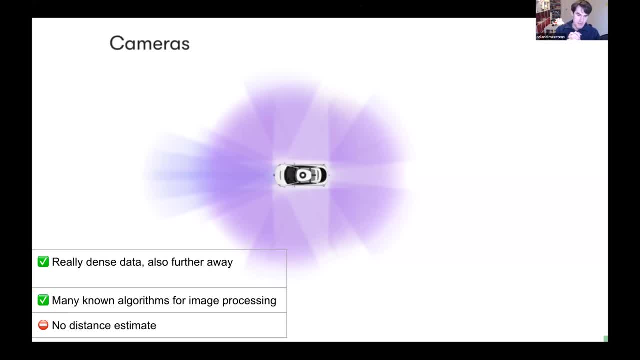 So cameras are really useful because you get really dense data also further away. You can see that Waymo here has two far range cameras in front of a vehicle, So that's really useful. There's also many known algorithms for image processing. Those images are laid out really nice and convolutional deep learning algorithms can handle them very well. 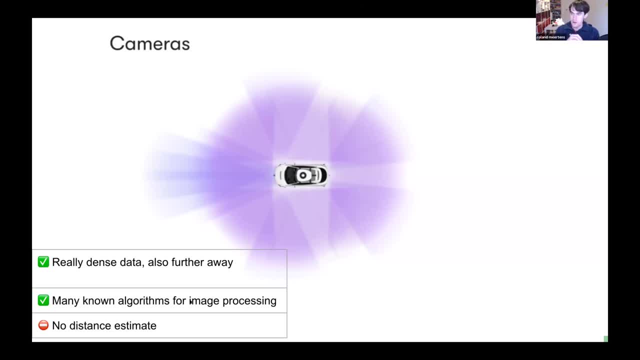 There's tons of research which we're self driving cars are currently benefiting from, which are not in the domain of self driving at all or robotics at all, But because people are solving the image net challenge, for example, we get way better ideas of what to do for objects. 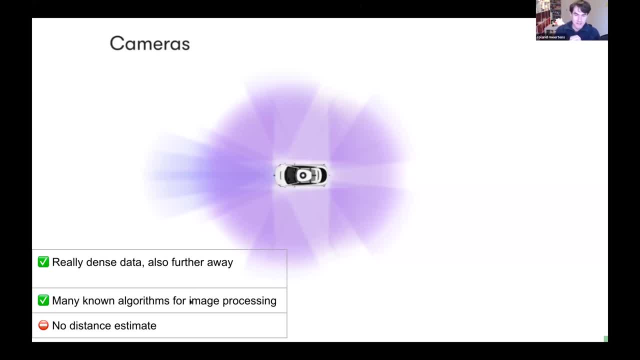 So that's really useful. There are должfront Итак. in my opinion, that's a big benefit of плоmm working robots and robotics projects, So that's a big benefit of Kamra. And then the big problem with cameras is that there's no accurate distance estimate. 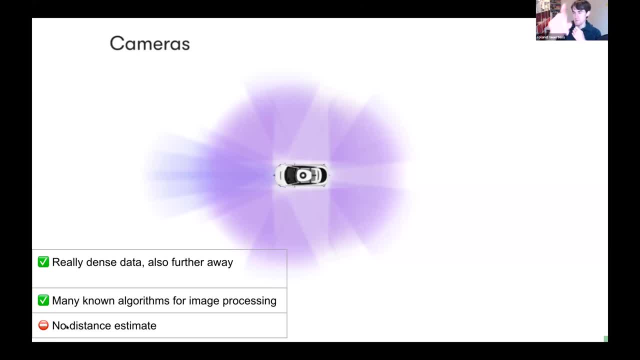 Of course we as humans can said: oh, this is probably farther away than that, but it's not a measurement, It keeps being estimates. And then there, areaki kasugrai lives in Japan, So that's hard. If you want to have information, you really can accelerate your robots or which are self driving car. 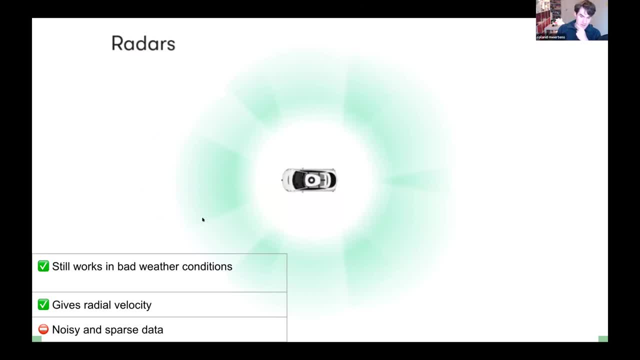 There's a few Area brains, as usual, and we don't really have, But at the moment they're data and robots and I think that there's a lot of data on there. thank you, is the radar? uh, so you can imagine that if there is uh snow or if it is raining very hard, or if it. 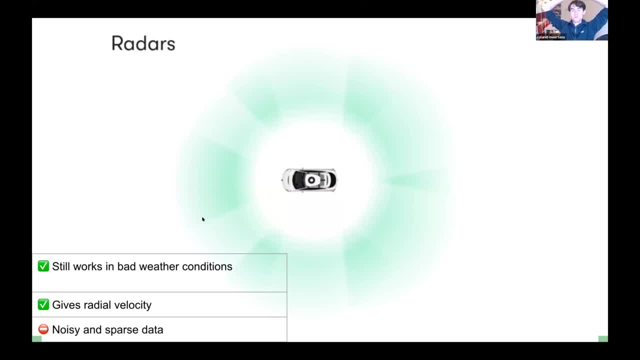 is uh foggy, then you can't like there's no light penetrating through the fog. or rain, right, uh, or maybe not a lot. so in these cases lighter has some troubles, or reflects of, like small wet surfaces, um, and for example lidar can't go through fog and of course cameras also can't go through. 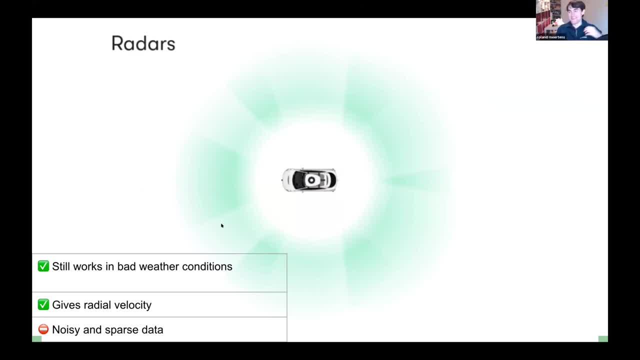 fog, but radars they can. so if you have better circumstances, your radar still works in better weather conditions. it also gives you something really cool, which is radio velocity, so velocity of other participants in the direction of vehicle. but the data itself is kind of sparse. so there's. 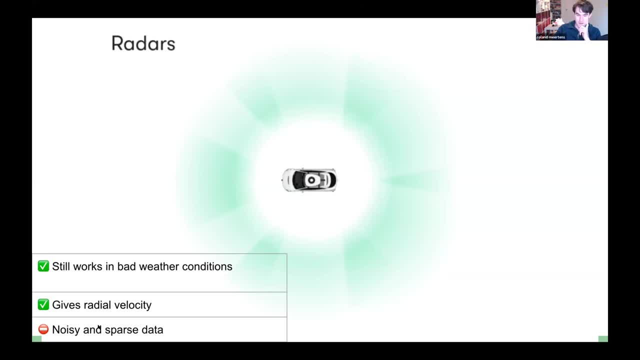 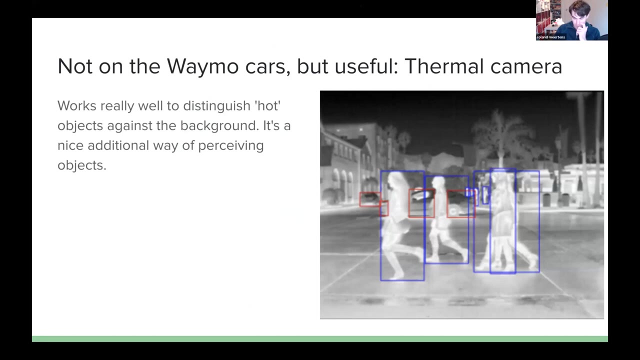 not that many radar returns and there's a bit of noisy data, uh, so in that sense it's less useful. but yeah, you can see that all these centers all together give a big um like give a big, good 360 degree view of what's going on in the world. um, and one other camera which is 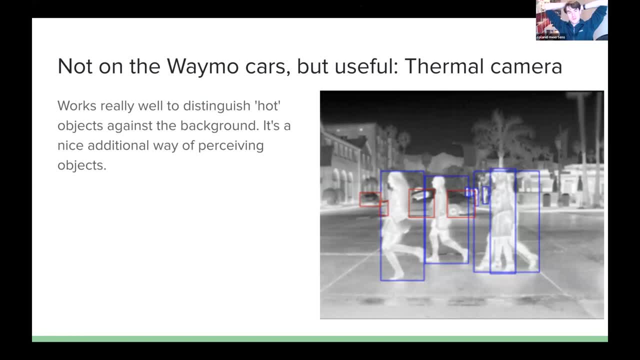 pretty cool for for robotics, which is not on the waymo cars, but i figured that you guys might like. it is a thermal camera, so thermal cameras really give you a estimate of the temperature of objects and you can imagine that if you have a robot deployed, for example, in a dark environment with normal cameras, that might be. 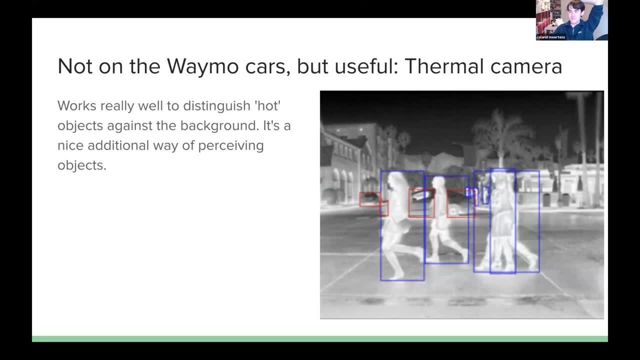 a problem, but humans are always roughly the same temperature, so they always stand out against a specific background. so if you're ever building a robot which also has to maybe drive at night or detect pedestrians at night, um, maybe think about a thermal camera, because it's a nice. 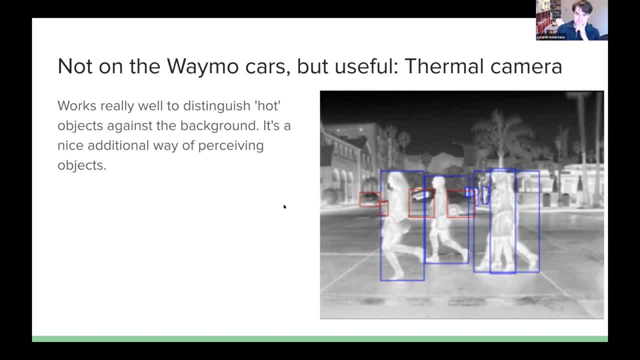 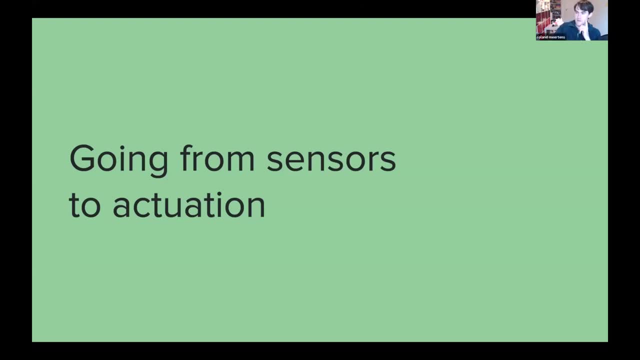 additional way of perceiving objects. um so if we now look at, uh, how we so, we now know kind of what center data we're getting into a self-driving car or robot right. so now the question is: how do you go from these sensors to actuation? 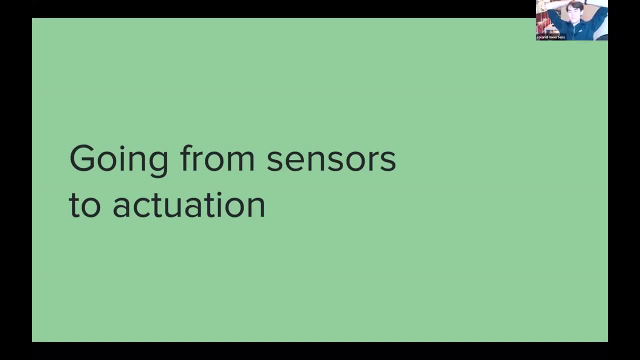 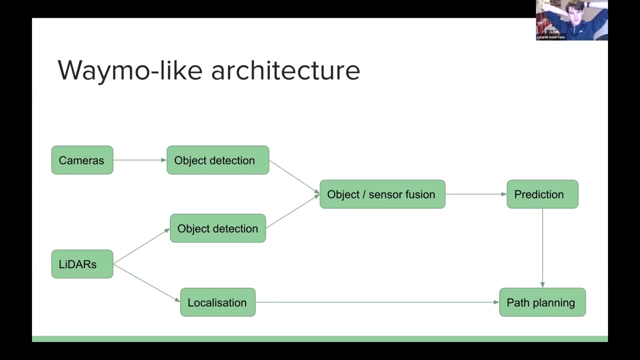 and i want to here again kind of highlight a bit of a difference between the level 4 robotaxis and the level 2 tesla and maybe comma ai, where you see that a lot of those robo taxi companies have a certain architecture which is really modular. 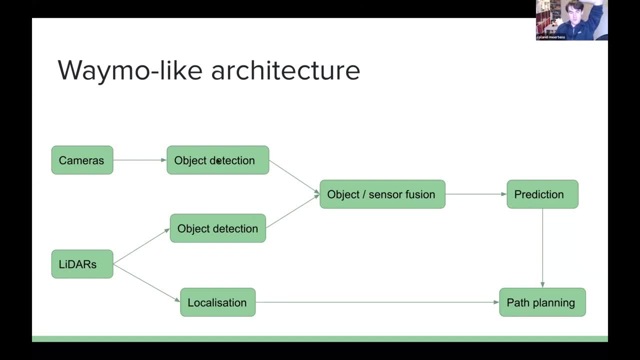 there's a lot of high-end software and stuff like that. there's a lot of stuff for picture detection, um, and there's lots of other things like x-ray sensors, uh. but the reason i'm showing you here are some things that are actually pretty specific. so the first thing that is: 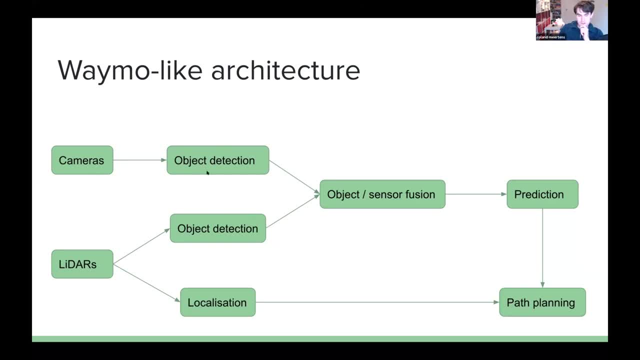 a lot of people don't have any idea about right now. um is. you can have a lot of things like three cameras and leders, and then there's often components for doing object detection based on camera data, and then there's a component which does object detection based on lidar data and 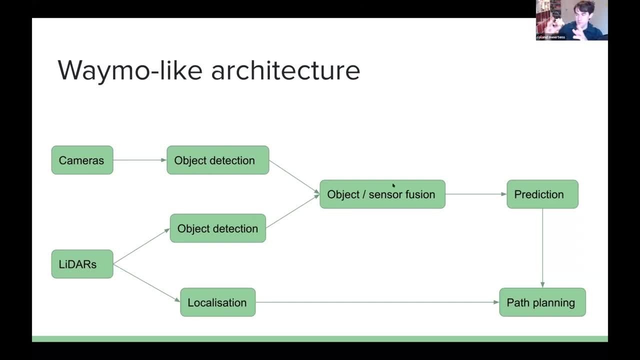 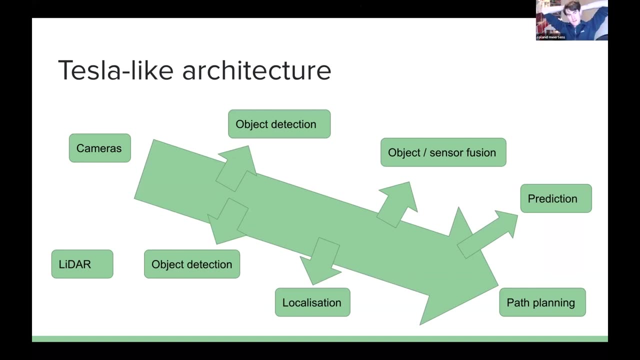 you've got your localization algorithm, which takes lidar and maybe gps inputs, and all this information is then passed through a path planning component. um, that's really like a way more like architecture, and then people always talk about a yeah, like a tesla, uh, like architecture. it's really easy to get started with and to end learning nowadays. 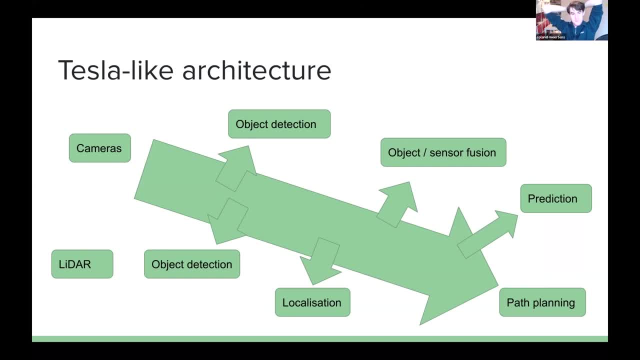 so many people, uh are thinking: oh, why don't i just take my camera data and pass that directly to a path planning uh component with a neural network, uh and also um, that's as i was talking about their hydra nets. so they have um as inputs or cameras and then they have all kinds of outputs. 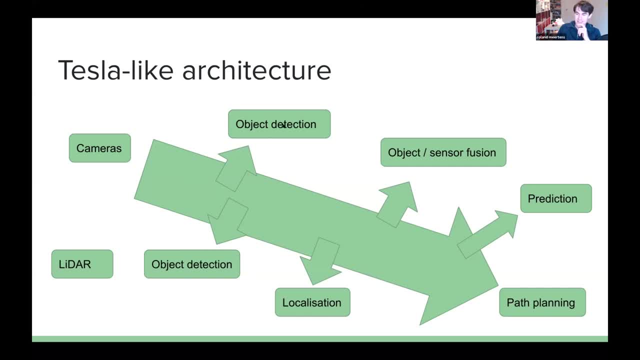 they can use as like proxies, so they have object detection- uh, they're training that. and to get on the same neural network backbone, they also do object detection, or, sorry, uh, the localization, um, with respect to lanes. and then also in the plug-in on the same latent neural space, they can do maybe center fusion, where they fuse all camera. 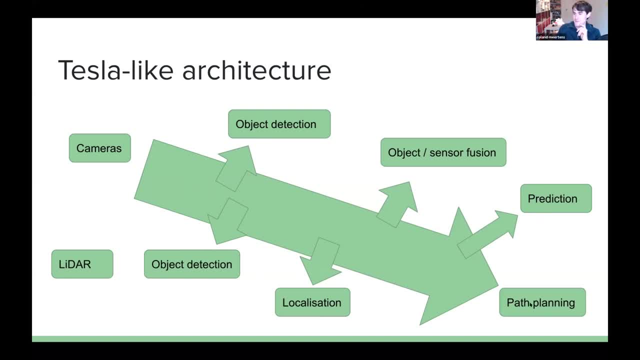 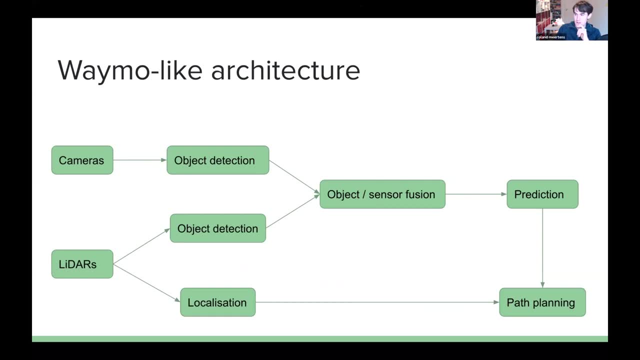 information. they also do a prediction and they kind of directly do the path planning based on the same information, and that's that's a big difference between end-to-end learning and, and this, all kind of modular approach. so, yeah, what i want to do is go over, uh, four challenges of self-driving, which 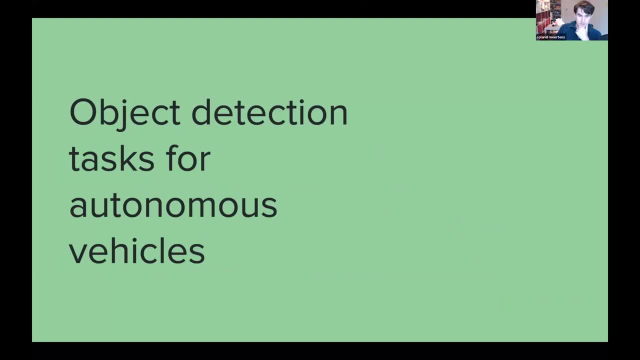 you are seeing often um. so there's a couple of tasks which people are trying to solve. there's many competitions for this, so if you are interested, download the data set, get started. it's loads of fun. one of them, which is very well known nowadays, is bounding box detection, where 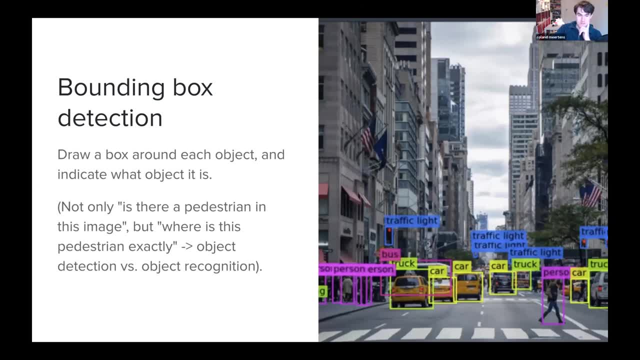 people draw a box around each object and indicate what object is um. so you're not only doing a classification task, like is there a predation in this image, but you're also doing a classification, a uh, saying okay, where exactly is this pedestrian, how big is it, how wide is it? so you can imagine. 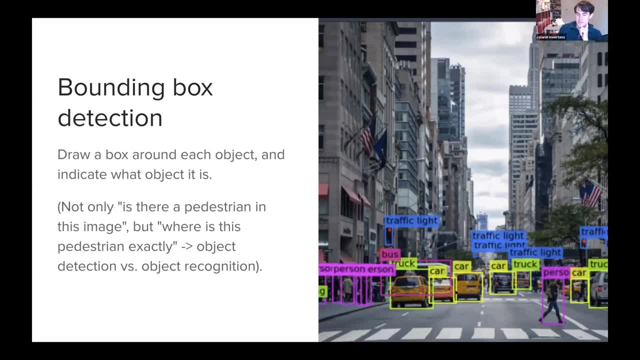 that if you have a car or a robot and you have this information, you can already kind of try to navigate between the bounding boxes. uh, it's, uh, it's still a bit hard, uh, because if you know where something is, you don't know, or you don't know what order thing which doesn't have a bounding box is. 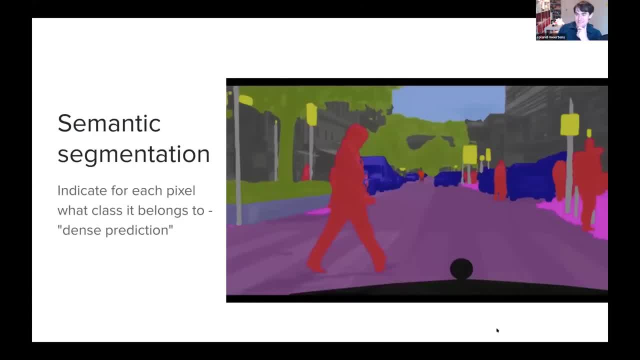 uh, but there's a task for that which is called semantic segmentation, and that's already more interesting, because then the neural network or whatever algorithm you have has to indicate for each pixel what class it belongs to. so then you're already doing a very dense prediction, uh. so if you have your input image, you're really saying, okay, this pixel, this is a pedestrian, uh. 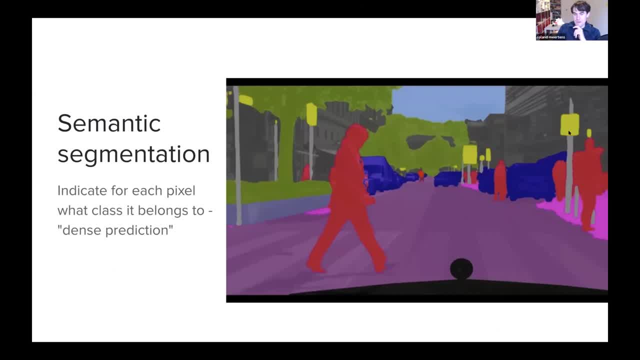 this pixel, this is the road. this pixel, this is a uh lamppost, for example. or this pixel, this is a building, um, i can already imagine that this way easier to navigate through, where you can at least have a feeling for, uh, that you're trying to keep being on the road, um, and then there's a task for 3d bounding box detection. 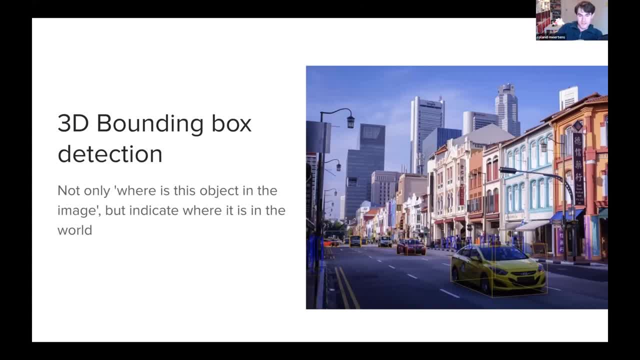 so then you're not only saying, okay, where is this object in the image, but you really say, okay, where is this in the world? uh, give me the 3d coordinates. uh. so this is normally where people start using lidar, because it gives you a way more accurate, uh, prediction of where an object is. 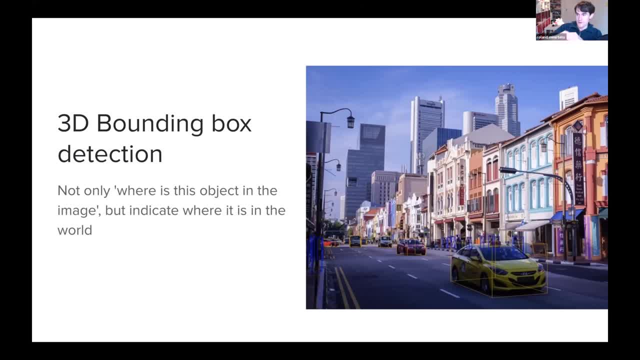 you, um, and often you're also trying to estimate the angle the object has and maybe the direction the object has, so that you have an idea for where the car might go. so that's important for your prediction component. uh, you're trying to estimate the size and, yeah, self-driving car algorithm of 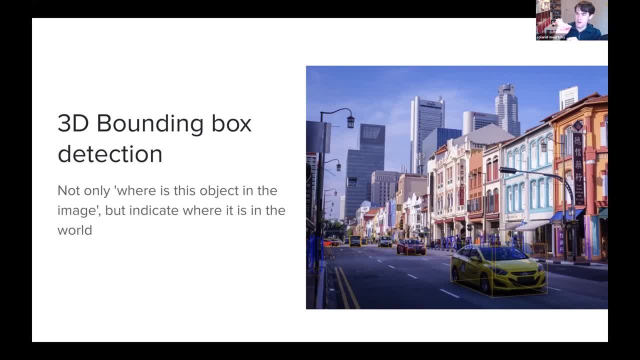 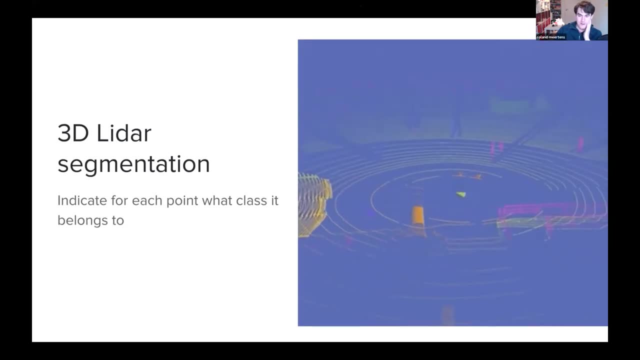 course needs this information, because then it can predict where objects are, where they are going. you can uh, you can track them. um. so this is a really important and difficult task, uh, where lidar starts being the main uh input for your algorithm and then there's another really cool uh algorithm. i hope you can see this. 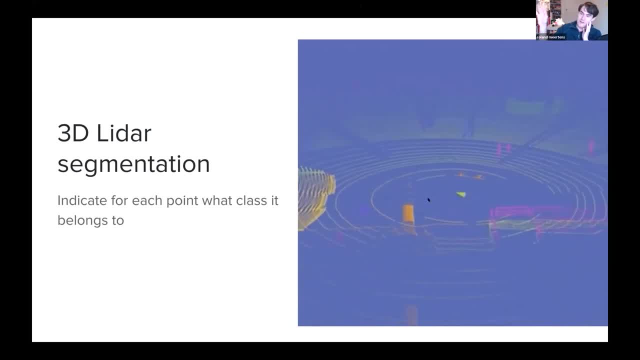 but that's the 3d lidar segmentation. so if you have a lidar, you got all your points in your point cloud for your laser distance returns. um, the challenge for your algorithm is really indicate for each point what class it belongs to, so you can see that here in this case. uh, the challenge is okay. 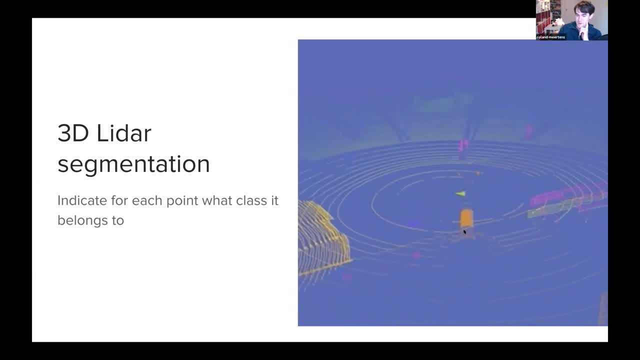 well this: these points here belong to a pedestrian, these points here belong to a tree. all these points here belong to the road, and then you can see that these points here belong to the road, and then you can see that these points here belong to the road, and then you can see that these points here belong to the road. 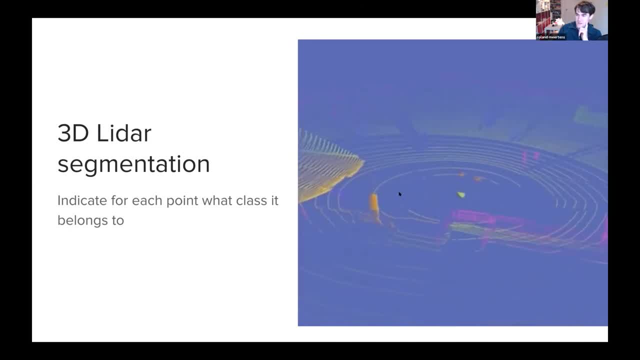 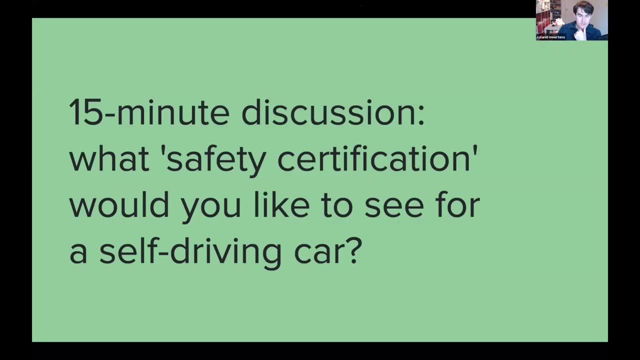 here's where the sidewalk starts. uh, so it's an even harder task, uh, but it's kind of kind of new like people started doing this since a couple of years. um, i think there's still a lot of growth possibility to improve these algorithms here. um, so now that we know what kind of uh tasks they are and what kind of levels they are, 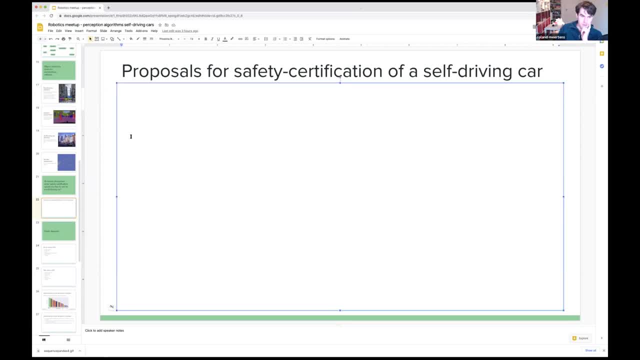 i figured that, um, you, as robotics experts might have a good idea for what you would like to see for the safety certification of a self-driving car, and i figured we could maybe have a couple of proposals. i'll write them down on the slides and then at the end we have a couple of nice. 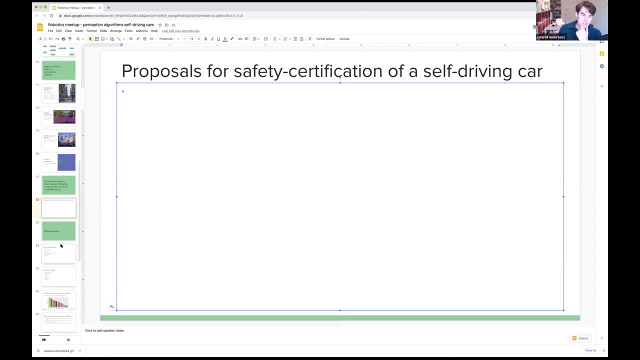 interesting proposals, we can have a bit of discussion, and after we do that, later i will tell a bit more about some aspects of the data which might be interesting there. so don't be shy. do people have any proposals or ideas for how you would safety certify a car? 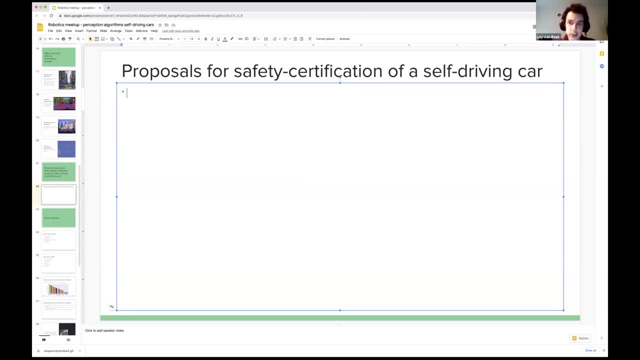 so so, um, i think there's two approaches you can take in general to this. so one is just um having a drive, uh, ex having a drive for basically the statistical way, just um having a drive a really long distance and have cover lots of different um roads and some situations. but the other one, the other one is analyzing this and uh covering. 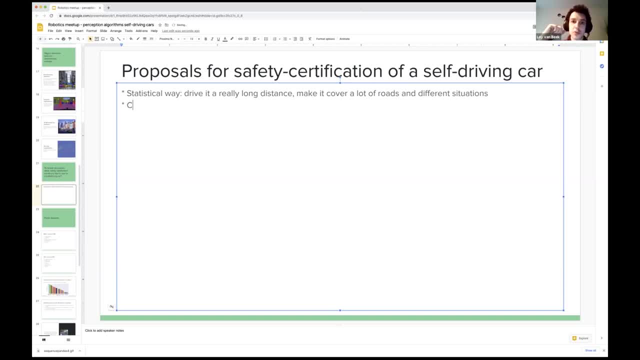 more on the software side? what types of stuff can more? it's not really formal methods, but can you prove that it handles these needs in these cases, which are two completely different ways, but i'm not sure which i'll which, uh, which i would prefer before i step into a car like that? 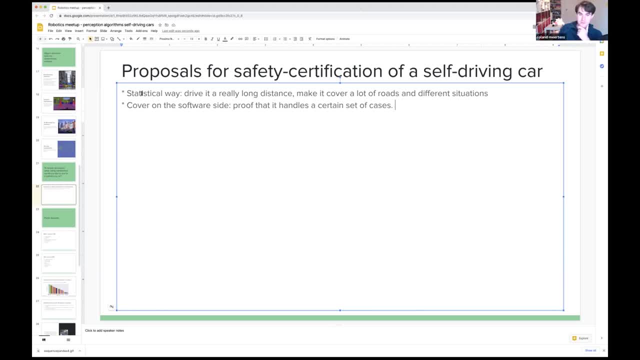 yeah, yeah, okay. so what i'm hearing here is that you say, okay, well, one way is that we can have a fleet and we drive it a really long distance and we make it cover loads of roads and kind of make sure it gets into different situations, and the other way is: okay, maybe we can. 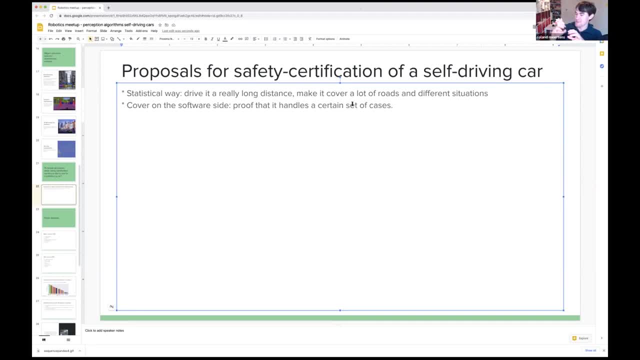 have a certain set of like test cases and we just replay them, or would you? would you, how would you prove that it handles a certain set of cases? how would you do that? um, no idea really. um no, i, i really wouldn't know. so that's, that's the problem there, and there's always, uh, there's always. 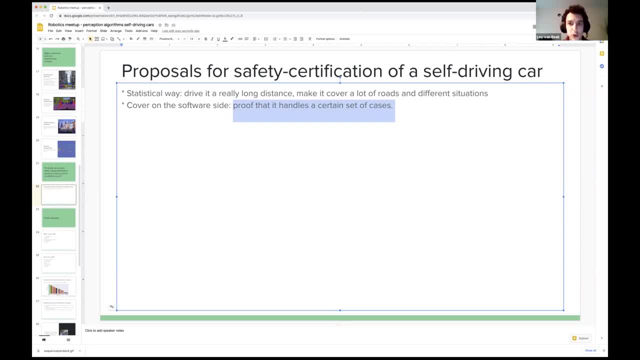 more cases that you didn't think about, and that goes for both situations, for for both these types of certifications, you can and and you could have buy them or get them. no matter how hasty plug you going, it depends totally on every person's umşallah. umth start to destroy your heart. i have a really 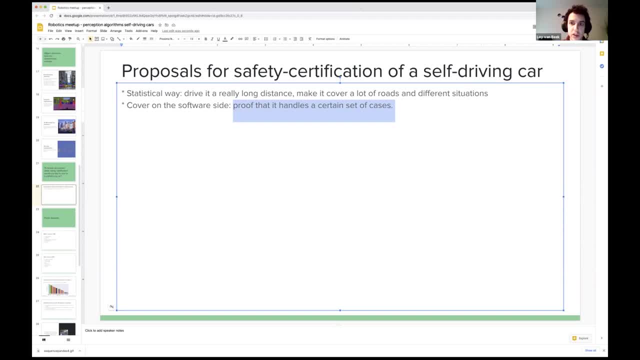 struggle with. i can't wash them, i can't give myself after they coolest felt over happened, not doing even a. I mean, you cannot drive it in every situation, every road, and you also cannot make a unit test, for example, for every case. 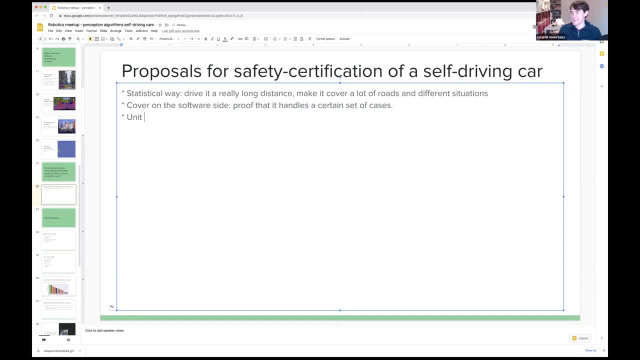 It's quite impossible. We'll just write down a unit test for a fixed set of cases and then we at least got those covered right, But it's not going to be enough. Also, it's the same for integration tests. It's there's. so yeah, you're dealing with human lives here. 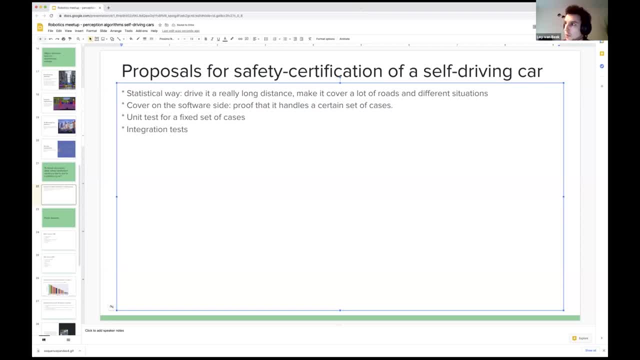 So I'm also not sure how, for example, airplanes software for airplanes is certified, or same for medical devices, But then I'm not even sure how that type of certification actually works. Do you have any idea, or maybe any ideas of things which you are doing? 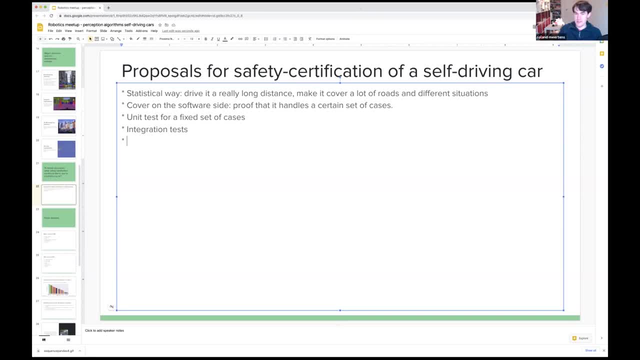 in the In the airplane and spaceflight industry, which at least help make an airplane safer. Yeah, there's well, there's different standards. you have to buy to like the automotive. there's MISCA-C, I think. There's automotive coding standards. 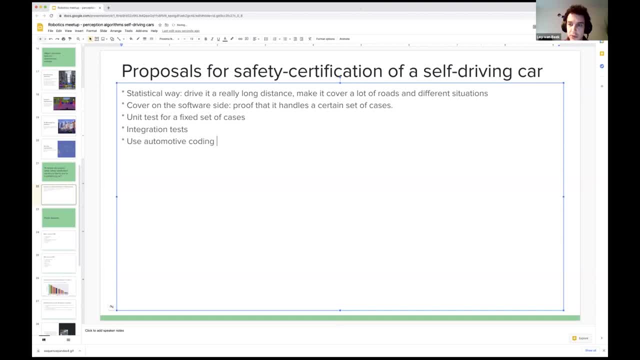 So that's one thing. I know NASA has extensive code reviews and architecture that kind of stuff. I think even in NASA there's like two teams: one team actually implementing stuff and the other team trying to break it. So there's, but that's like just general code review and QA testing. 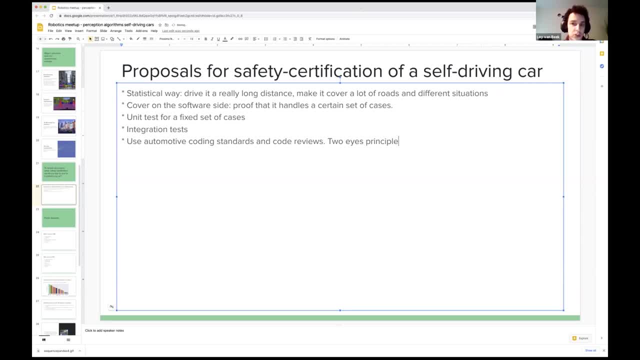 But yeah, But for stuff like computer vision and neural nets that's almost impossible to have it adhere to any form of method. So there you get to the statistics. Yeah, So that's not so sure, I don't know. It's difficult, that's for sure. 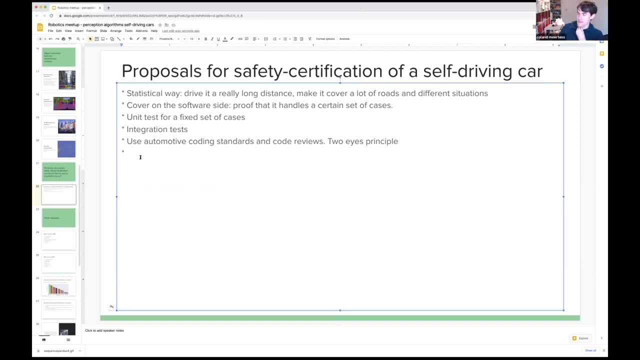 Maybe anyone else has any things they know about the airplane and rocket industry where they- which they do- use to make sure that rockets and airplanes are safe. I don't have extensive knowledge but I know that you have some guarantees on some sensors. 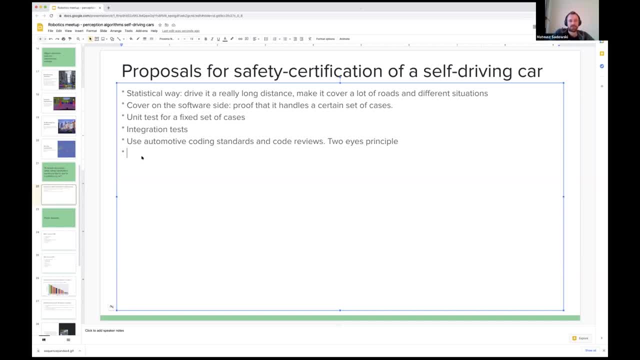 So you have guarantees- Yeah, Both on sensors and some on the hardware and software execution, So you can have hard deadlines that you need to meet at all, yeah, at all times. And also, I would add redundancy as well, So you can have redundancy both in software and hardware. 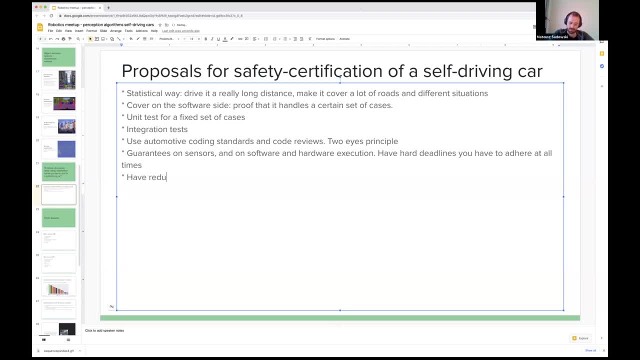 So yeah, And I think the redundancy is an interesting, interesting thing, right? So I know that rockets often have multiple flight computers where you see: okay, well, do they agree with each other? to also see, in automotive driving there are some companies. 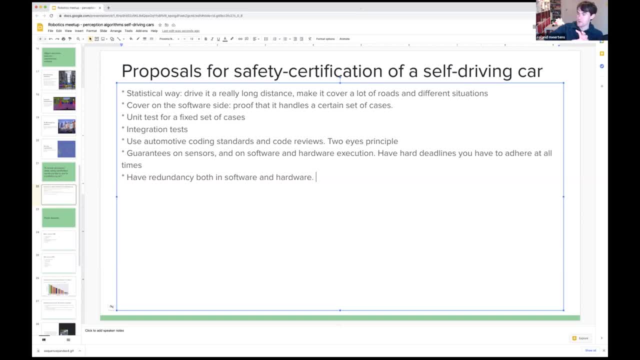 who have two computers And, for example, Auto-X Chinese company. they have two self-driving stacks which run exactly the same software And as long as that like agrees with each other, they think okay, well then, at least we nothing in our software in one of the computers just is suddenly corrupt. 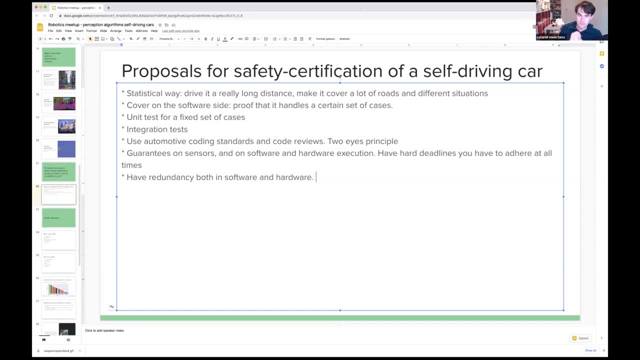 But there's also companies which have, for example, two self-driving stacks and one is using traditional methods And uh, and the other is then maybe using like deep neural networks, And then, as long as they agree with each other, they know okay. well, I guess this path is safe and good. 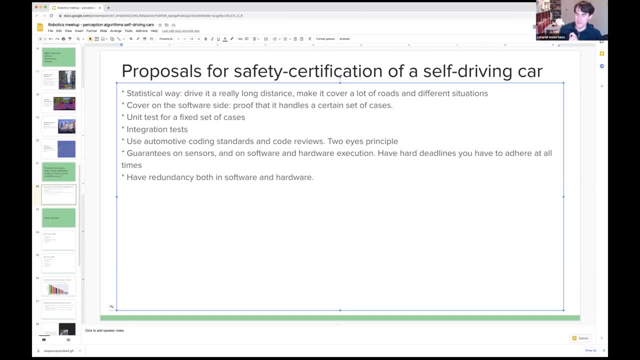 Uh, but yeah, as soon as they start disagreeing, you, uh, you have to think about: okay, well, what's what's uh? what's uh software is probably right, Or what's software is probably doing, uh, making good decision. 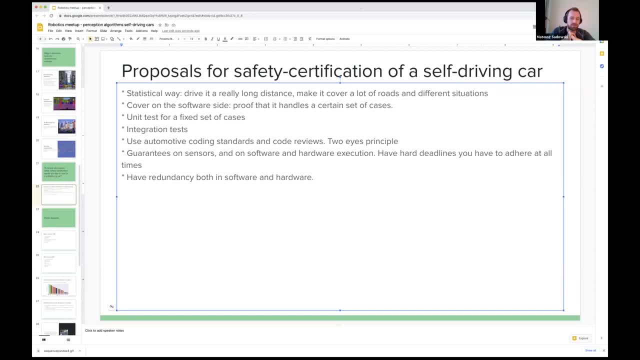 Um, I think the comments in the chat, Sorry. Yeah, Go online. Yeah, Just just want to. it's also hard in some cases, of course, to even define what is the right way to solve some, some, some situation. not killing people and being safe is most obvious, but, um, it's uh. so there's, of course, the, the, the, the trolley problem. 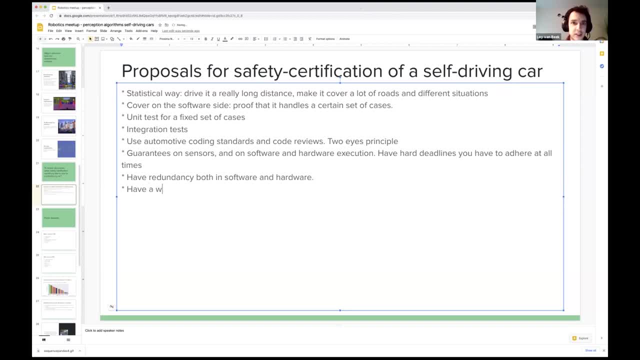 It doesn't really apply. Is that something that's actually considered this type of thong is? or should it just slam on the brakes and Make it a good um? try to avoid any issue whatsoever. And then I mean, is it, is it even a thing that is being uh, is it still relevant? 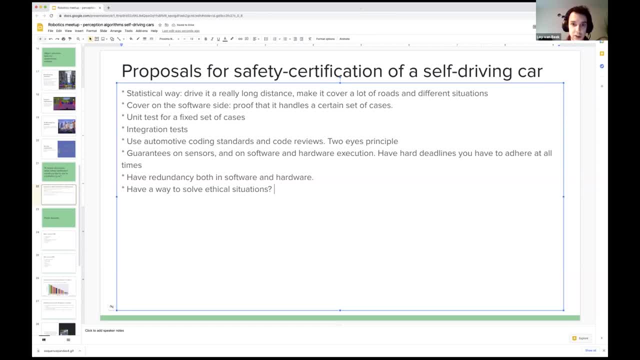 This kind of uh situations or questions is: are they being considered or is it? I'm just blabbering? Yeah, I think it's an interesting, uh interesting thing. So actually I was asking this yesterday um to a couple of people at uh, at uh university. 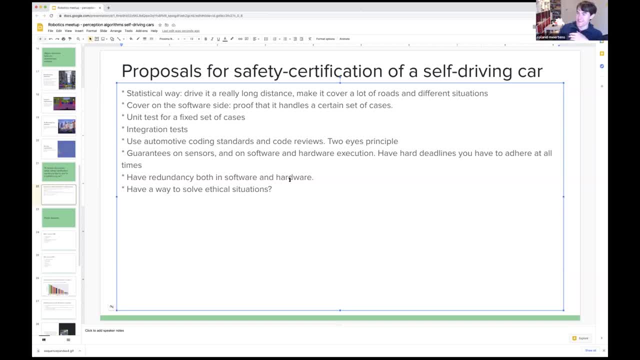 Um, and they are. someone Just said: okay, well, let's uh appoint someone in the. in the country I have a committee that says: okay, if the car sees this, you have to respond in it in this way. 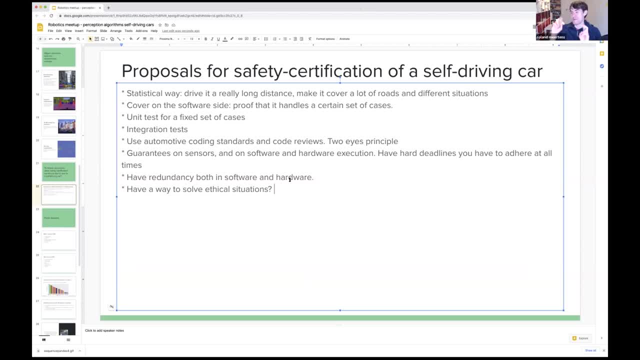 Uh. so basically he said: okay, well, let's solve the trolley problem by just appointing someone who is in responsible for, uh, for solving it, Uh. and then you have a set of test cases where the car has to make the right ethical decision or has to make the right decision. 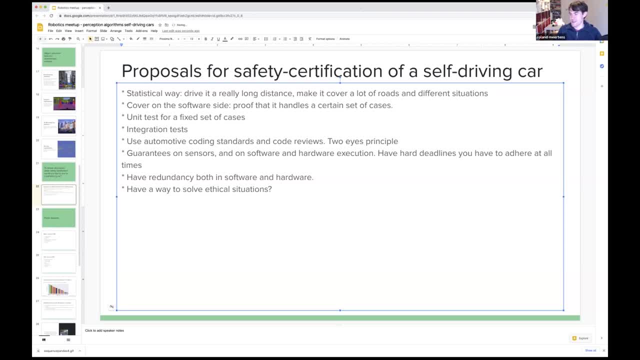 Uh, but yeah, I'll edit here: Uh, I don't know how much of a I think this. so the problem is that, uh, normally you try to keep the car safe in all situations, right? So you don't uh hope that you're ending up in one of these situations. but if you, for example, there are situations where it's really hard for the car to um to really not get into an accident because if it's gets surrounded by four cars, yeah, 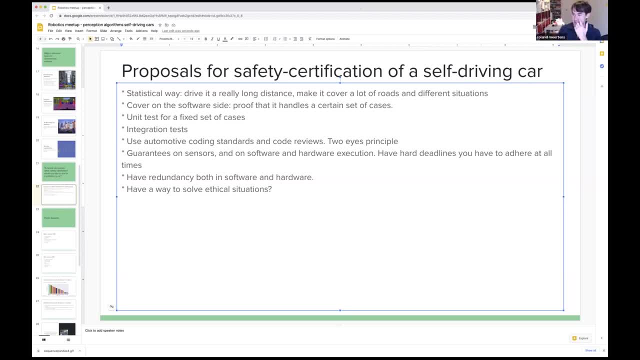 Then you are driving, then you can't go anywhere without hitting a car And in front of cars breaks you. you can't make a, make a, You can only like, take the path of the least damage, but not not in a part of no damage. 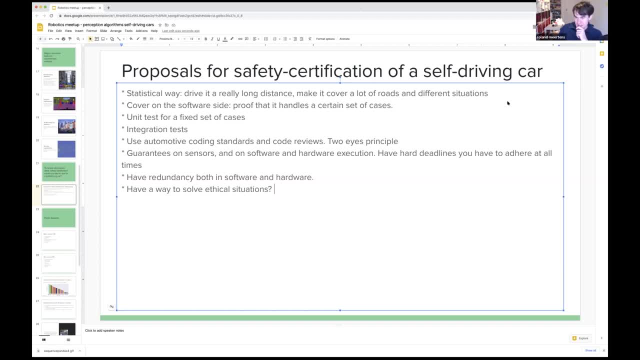 Um, yeah, I see, by the way, a couple of uh comments in the chat. uh, maybe do you, can you uh, or can someone summarize them? or Uh, I can add a comment about the uh, the paper that I linked. 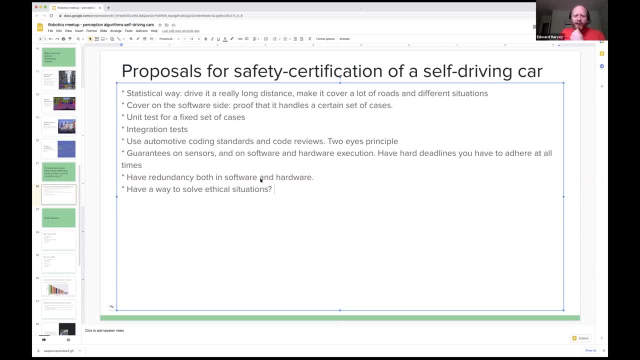 Um, so I I definitely don't know much of anything about certifiability, but I do know that, uh, uh. so Luca Carlone is the- uh, the author on the paper that I linked, And, Uh so he's a professor at MIT. 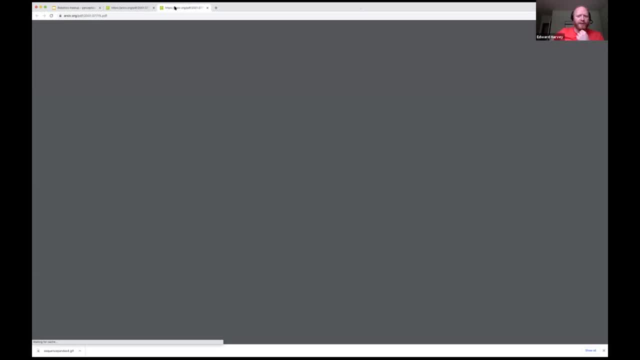 Um, I've seen him, uh, give a presentation on some subject that was closely related to this one, And, uh, and so he's always talking about certifiability, and this is something that they're very clearly working on. Um, so, as soon as you mentioned it, that was the first place where my, where my- mind went. 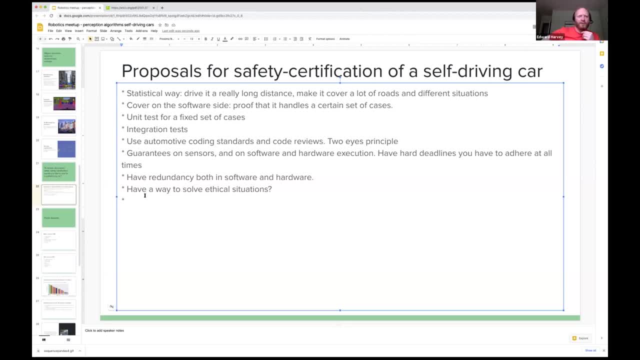 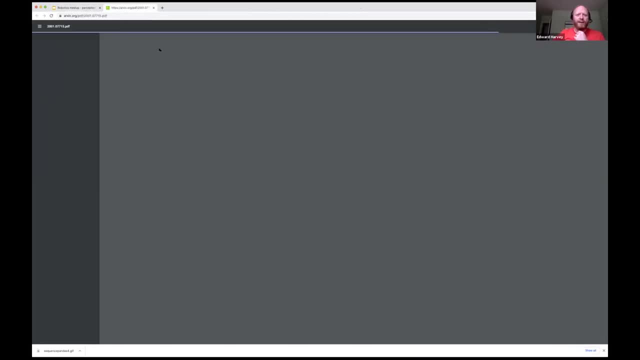 And um so, just while we were sitting here, I quickly searched through my archive of his papers and found one of the ones that uh makes certifiability uh explicit point, And so that was the one that I linked here. 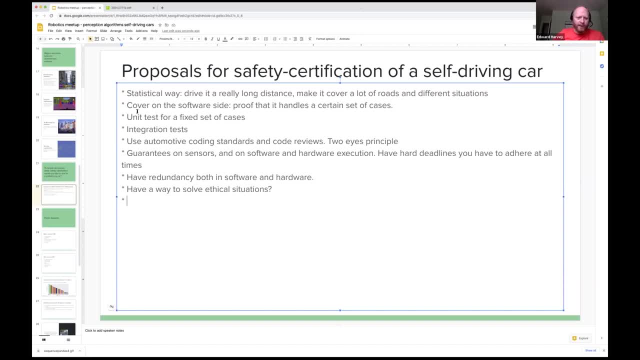 Um, uh, so in that paper, uh- I have this up on my screen right now- Uh, appendix a on page 21,. um is where they go into uh, defining, uh what they consider to be the criteria for um, for certifiability, and the justifications and the ref references that they have of, uh, you know, prior work and so on in this area. 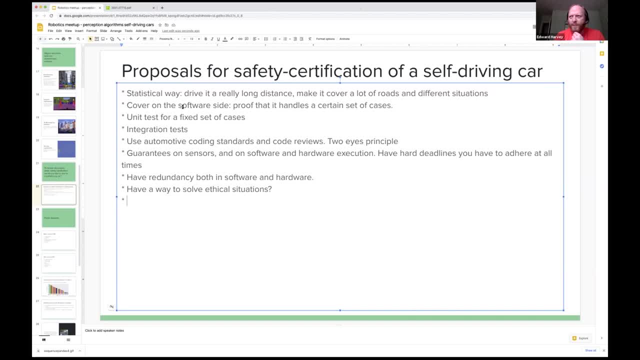 And what. so what they're doing is they're looking for, Um Uh, some kind of provable algorithm that uh is either able to give an answer that it can prove is correct or give an answer saying I don't know. 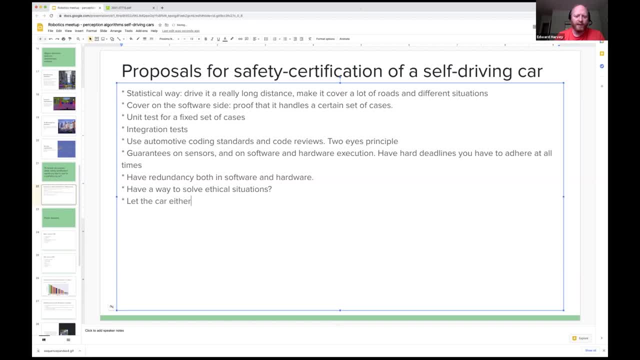 Uh, and you know, because it's just undecidable in the amount of time that was given or the algorithms that are given, or whatever. Um so, uh, so they're, they're looking for something that comes out with a deterministic answer, even though you know, we, we understand that the problem is unbounded. 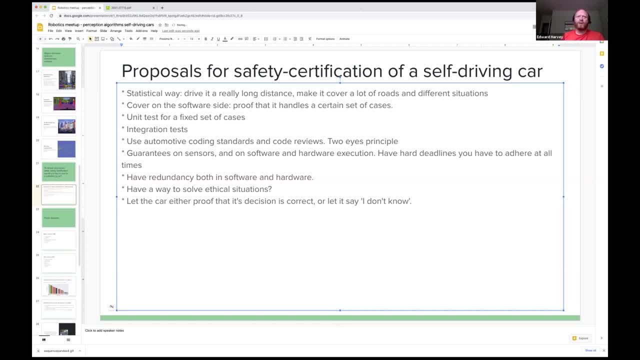 Um, so, uh, so they're, they're looking for something that comes out with a deterministic answer, even though you know we, we understand that the problem is unbounded is not a deterministic problem. Um, but you can deterministically come up with an answer that says: I don't know. in the situations where I don't know, 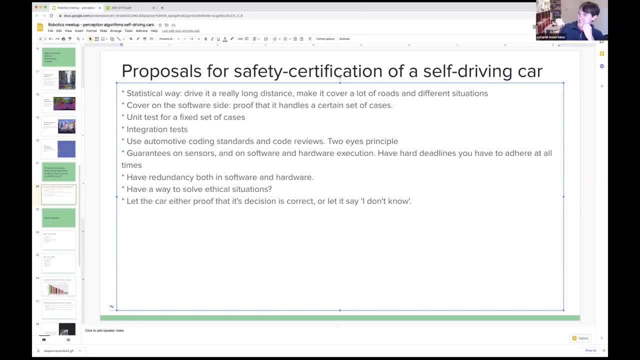 Yeah Well, what's Judy card do if it doesn't know? That's a really good question. So, uh, I think that touches on the the ethics question. So I took uh a class specifically on AI and robotic, uh ethics with uh Matias Schweitz, uh from Tufts, and um, uh, long story short there. 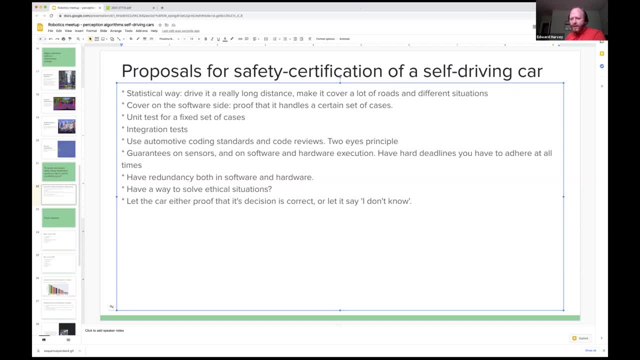 Uh, you can't just do nothing because lots of times, doing doing nothing is the unethical choice, And also you're on the highway at that moment, right, So you're driving really fast, Yeah, So so you can't just do nothing. 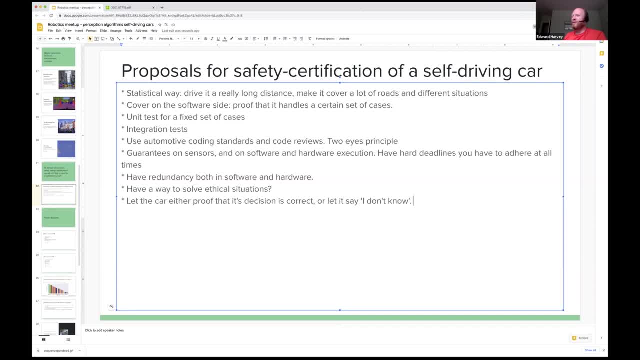 Um, and I'm trying to remember. this class was a few years ago now and it was just one class, Um, but uh, we had. the conclusion that we all reached was that you have to have an explicit ethical decision-making system and that it has to be a hybrid, that you try to make these deterministic choices if you can. 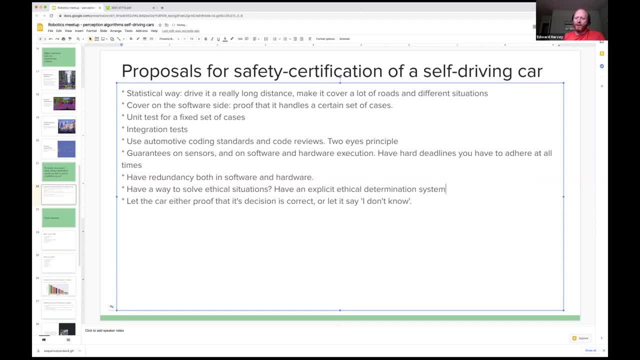 And whenever you can't make a deterministic choice, then you have to rely on something that is less precise, which may be a um I. I think we were concluding that the What seemed like the best non-deterministic uh, uh um agent was something that was uh cooperative, inverse, uh reinforcement learning, CIRL. 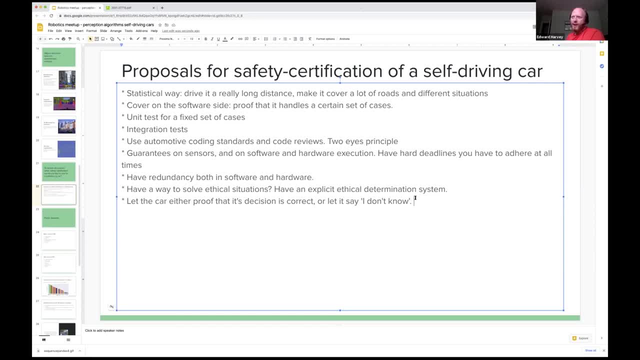 Um and uh, you know. so you train an agent, um, with an expert, uh, in these edge cases in advance, and then whatever you're able to train into it, that's what it has to go on at the time when something uncontrolled is happening. Um and uh, you know. so you train an agent, um, with an expert, uh, in these edge cases in advance, and then whatever you're able to train into it, that's what it has to go on at the time when something uncontrolled is happening. 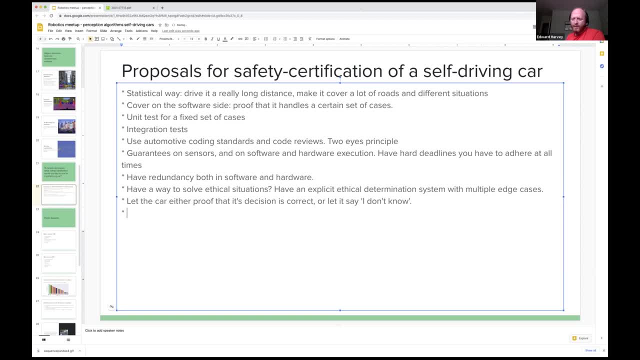 Yeah, It won't always be right, but neither will a human. Maybe, maybe one uh. one other proposal is to: to try to have the car always plan the safe path, uh, before making a uh, uh, planning for the next, uh. the next thing to note. 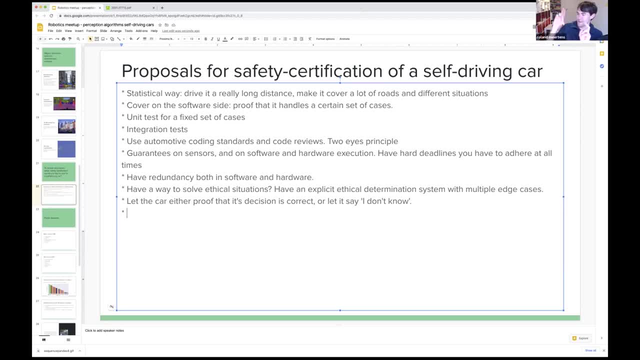 Okay. Well, if there is a problem arising in the next uh uh frame, or in a second, then I will at least be able to, for example, park on the side of the highway or at least uh, whatever happens after this decision. 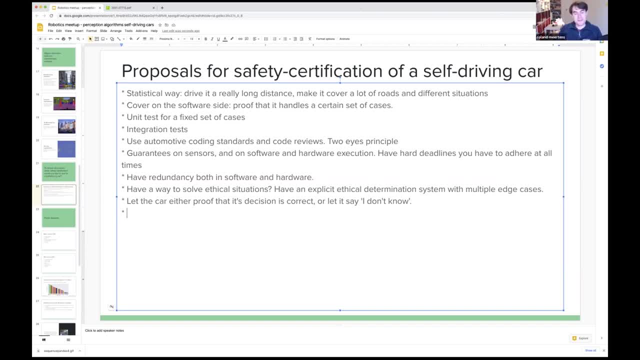 i will always be able to uh, to come to a safe stop. so i will just add um, add a safe, safe path. so where you have kind of maybe a more traditional classical planner, you just say, okay, well, what's, what's the worst that can happen? at least i will try to come to a safe stop and make sure. 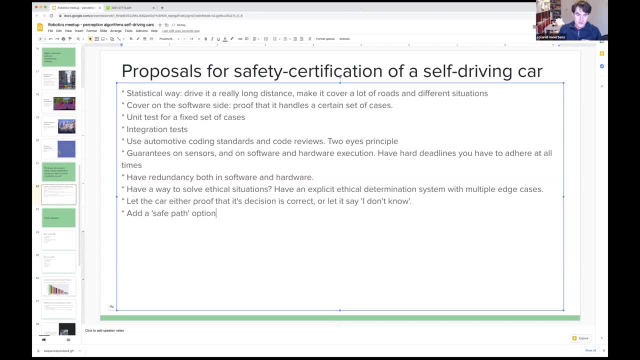 they always have a safe path to go. um option in your car, maybe? yeah, wait, i quickly want to look at. i also see that, uh, ignat georgiev had a couple of suggestions in the chat. uh, so i think he we have actually more um, but do you want me to read them, or? yeah, i can actually summarize this. 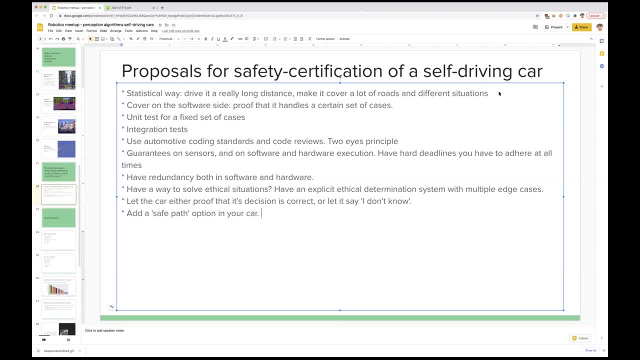 if, uh, you can hear me, that's my command. uh, it's vignesh here, so i would just uh put them all in one short point, like um. it would more or less second the comment from loy van beek with regards to the airplane industry. so, since we're already talking about, um, the highly 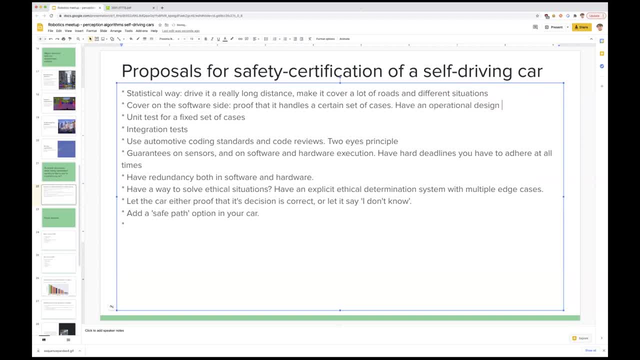 developed autonomous vehicle kind of a concept or a technology here. uh, we can probably make uh use of the uh or exploit the advantages that's already available in aircraft industry, such as a black box which would record in case of uncertain scenarios. so since we are dealing with um, you know, 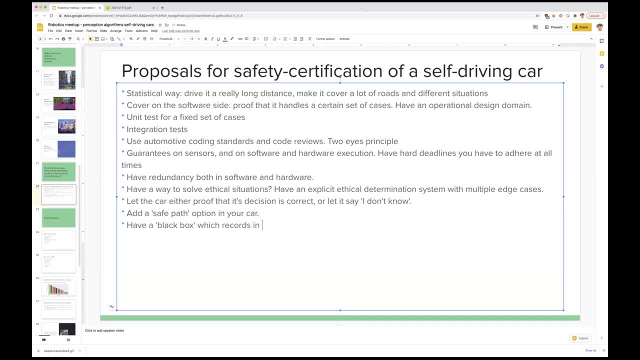 something that's out of your control and uh, such uh devices can help us to understand the critical or the corner cases, um, that can be recorded and what evasive actions from the user is usually done and which is a good evasive action and which is a critical or a lethal or unavoidable, uh evasive actions that's being carried out from. 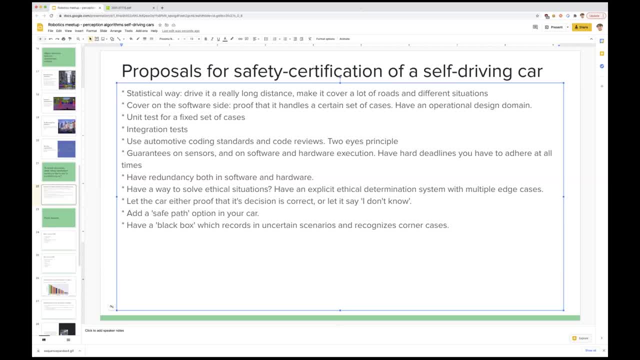 a driver point of view, because ultimately, what we might try to match is um the safety of the, the driver as well as the, uh, i mean to say the ego as well as the other counter vehicle or pedestrians um in the particular scene or incident whatsoever. so, uh, this can help us uh achieve at a more realistic inference of the situation and of. 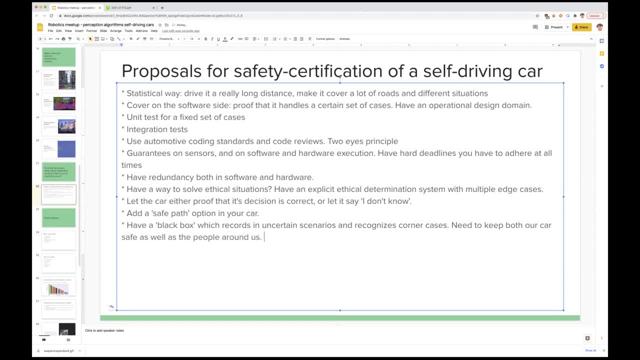 course, we don't have to always, um, look for the best case scenarios, because what we are trying to achieve is the development of the technology, and what we might look forward is towards addressing the corner cases, or what can be really be bad and um, so you don't have to really, you know, reinvent. 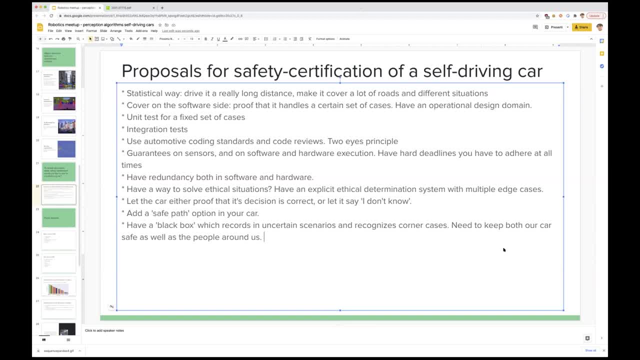 the wheel of trying to find some new standards. but, uh, when you have such a device which can give you the inputs of, uh, the reactions from the driver or whatever things can be locked in that particular incident, it's going to be an good information for us because, end of the day, this particular data would be 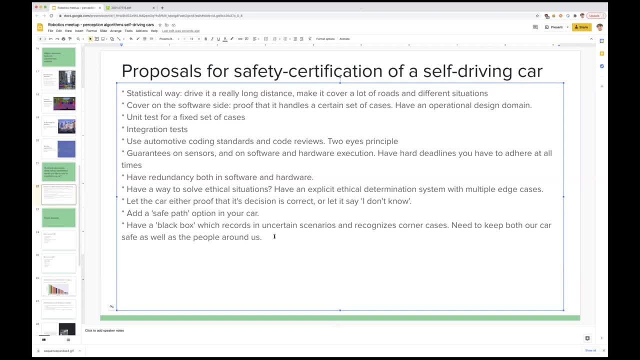 really precious for us to observe that. and secondly, um, since we are talking about self-driving now, we we are talking about all the neural networks and stuff and uh, to bring it into productions or make it realistic there, um, there are still a lot of steps. that needs to be understood, unlike 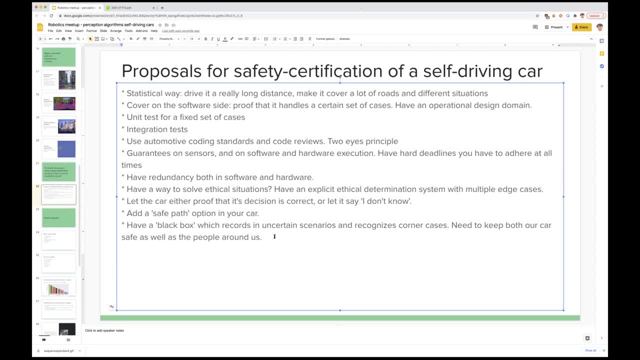 uh, you have the esp or an abs. that's more or less an algorithm based kind of an information. but here on the deep learning front we do not really have that understanding or a good grip as that of um, an abs or an esp technology and um, so so a standard or a. 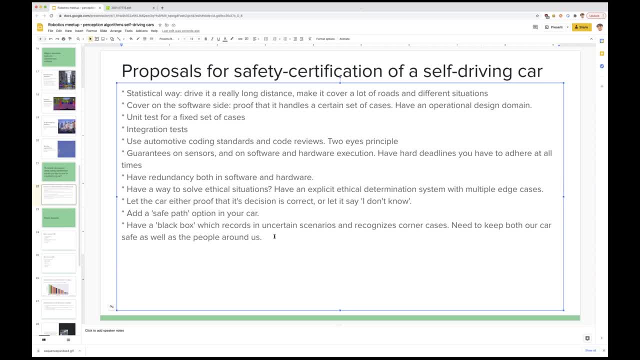 certification or a safety point with regards to the neural networks would be a important backbone that i feel uh, which will be needed to uh to understand and go towards a safety certification point of view for a self-driving car. so something like: right now we are pushing towards an explainable ai. that's like the trend that 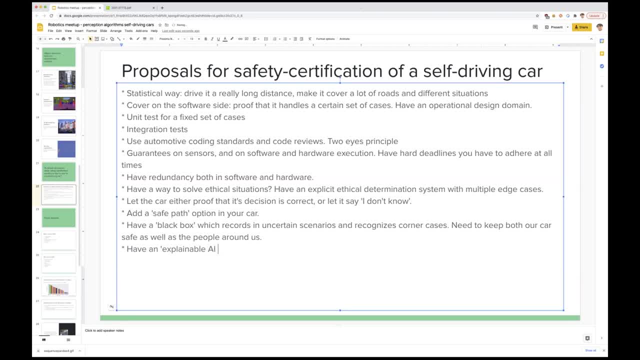 would be making sense. in a similar fashion, we would have to look at it for the networks that are being dealt in- self-driving cars, yeah, and that you better know, uh, what is this algorithm actually doing, or what it's actually thinking, or what? what can actually detect? that's what you're saying, that if you have a deep neural, 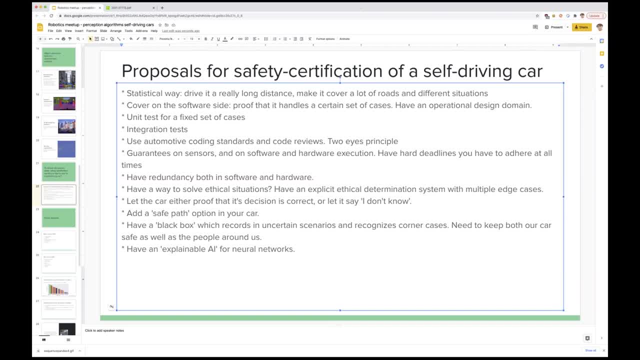 network in there. you should if, before you let this car on the road, you should also kind of show: oh, this is actually what the network learned, or this is what it. what it shows, uh yeah, pretty much like a cognitive intelligence, that we as humans have something that can be interpreted by the network. 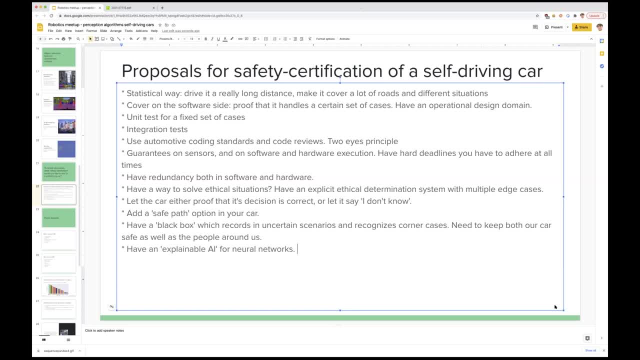 so, when we try to understand what behavior that it can give uh should be correlatable by us as well. for an, a scenario, a, this is what a collective information from a human, or a person as a human, would give, and does the network also have uh, such, um you know, reactions or output behaviors, and 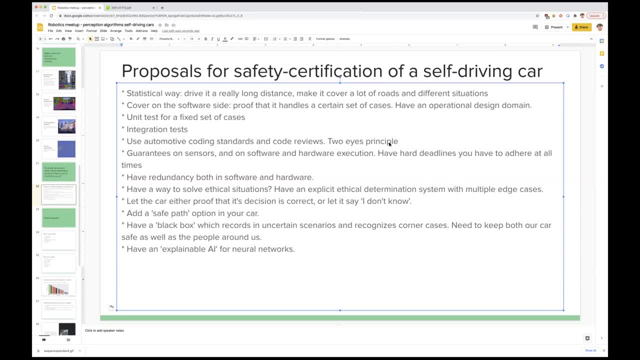 that that, basically, is going to give us an understanding about how the network would behave. so, just as uh seconding your point, that was, understanding how the network would behave, basically, yeah, yeah, yeah, yeah, it's an interesting one, um, cool, yeah, thanks, uh, then maybe, uh, we've had 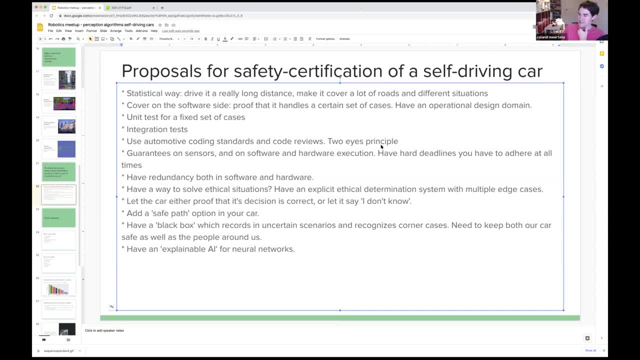 one more chance, right? so that was you right, vignesh? uh, like you can't see? uh, yes, that's me, that's me uh. so my points are pretty much summarized and i do not have any further questions. let me also write down your uh. you're using: using uh. end cap. 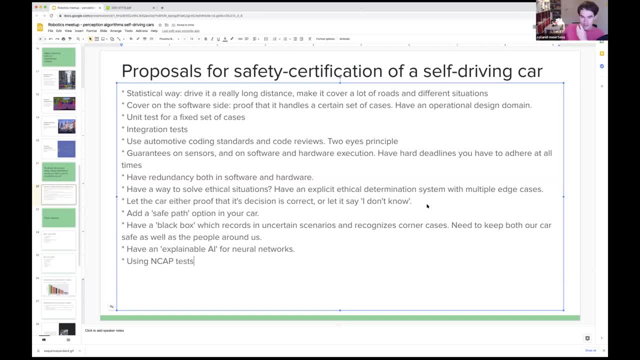 tests. uh, that's also a bit difficult. and then we had ignaz who said, okay, well, let's have an operation design domain uh, for example, daytime, uh, nighttime. so just make sure that you uh can drive under certain, certain circumstances, and then uh have people or have your cars only drive then and there, which i think is nice. i summarize it here: 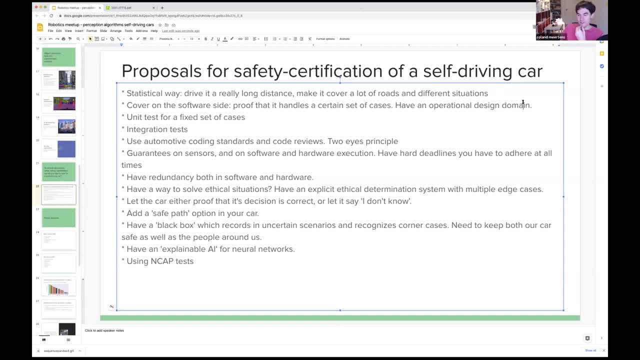 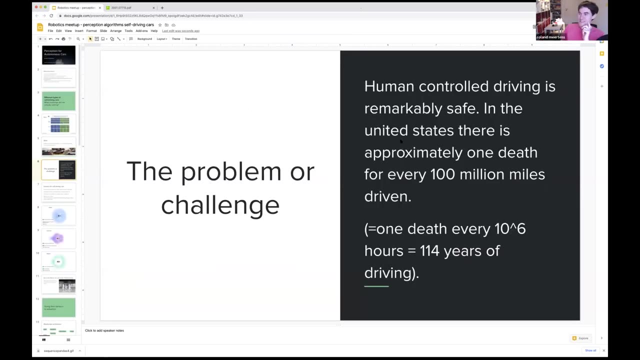 and he also says, okay, have more granular criteria for success, rather than just say, oh, we didn't crash, which is maybe the statistical way. there's maybe also a thing for the statistical way that we already saw that human control driving is remarkably safe. right, so if there's only one? 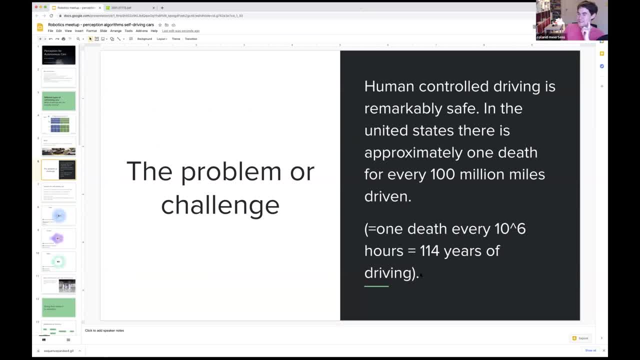 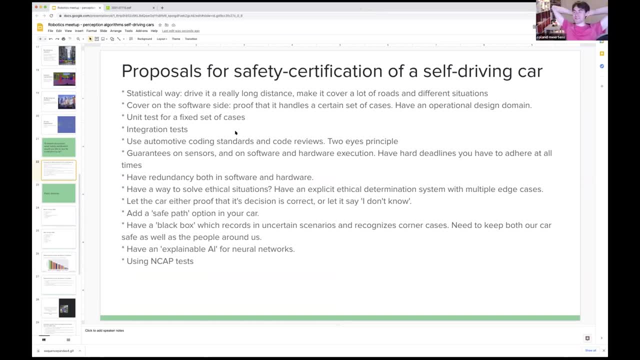 uh, one debt, the crash, every 114 years of driving. the statistical verification is really hard to do, uh, and i actually think it's interesting that for humans, uh, you base the decision whether a human is allowed to go on the road on a 20 minute, or like maybe an hour, driving test, where a driving 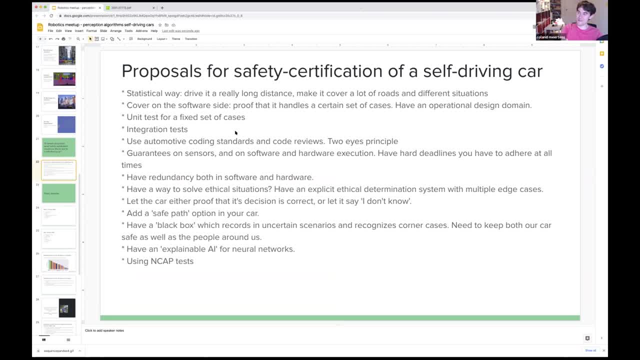 instructor sits next to you, so if you can manage to not cause an accident, uh, for an hour, that apparently is enough proof for our current country that's, uh, you'll probably not do anything anymore. ah, i think it's fair to say. uh, i think everybody will be given a chance toHANDA to turn around and 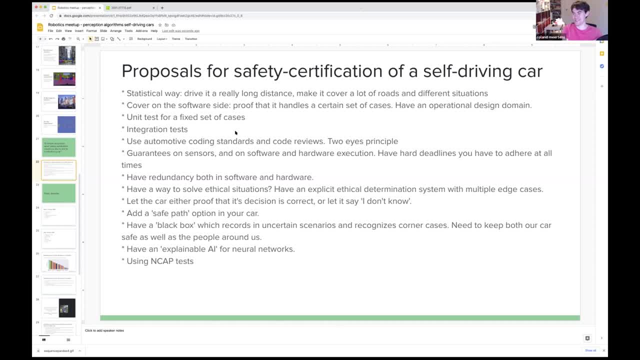 not to make a. make an, have an accident for the rest of your life. um, maybe something else which is interesting about the both: uh, maybe the statistical way, um is: uh, what happens if you do a software update right? so if you, for example, look at the driving test i mentioned, um, or yeah, 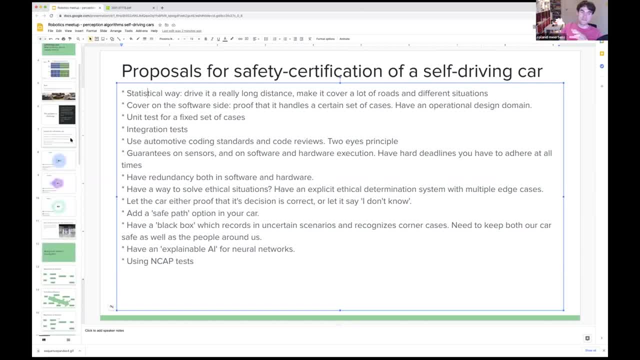 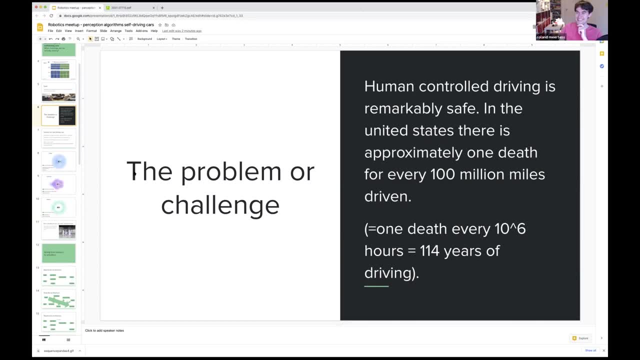 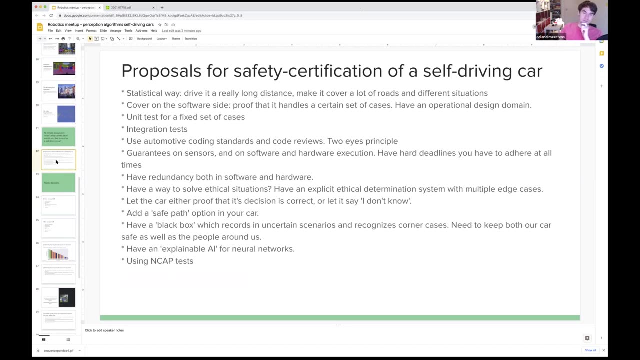 maybe another comment. if, if you want to do this in a statistical way for humans, uh, then actually you should have a driving test which, uh, which lasts like uh 114 years, so you would have to do a really long driving test. uh, i think it's a nice proposal, um, but if you want to do it in a 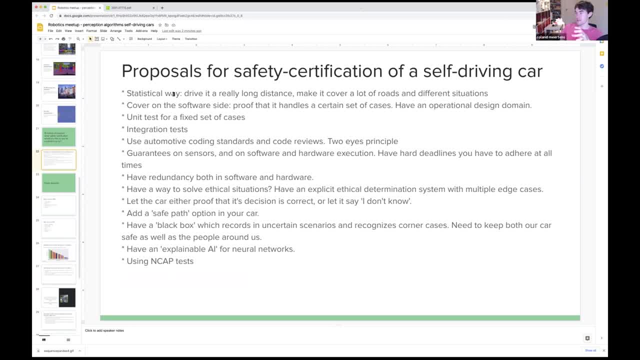 statistical way. what do you do if there's a software update? because if i'm uh deploying my car and uh of course you'll get into new situations and you have a software update at some point, um, what do you do with it then? do you have to, uh, do you just say, okay, well, 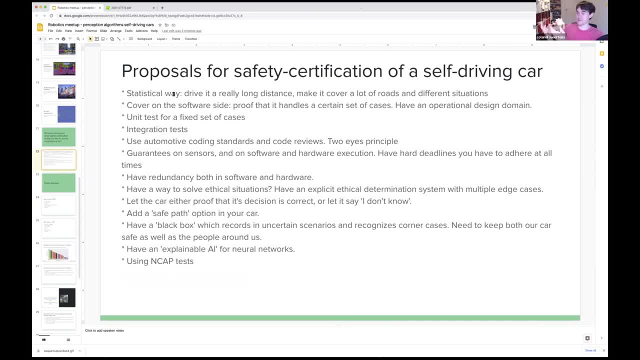 we saw that you're safer in this one fleet. uh, it's okay forever now. or do you uh also have? uh, have like uh all the other things, like your redundancy in hardware and software? uh, do you have your automotive coding standards up to date? doesn't mean you can just deploy new. 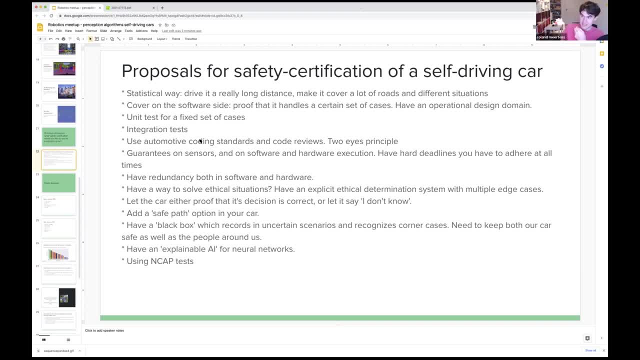 software, or do you have to go through the same statistical verification again? um, those are always interesting uh question. yeah, there's indeed, i'm with this- uh kind of things like: uh iso 262. um, let me also write that down. so that's really for the coding side, uh iso 26262. 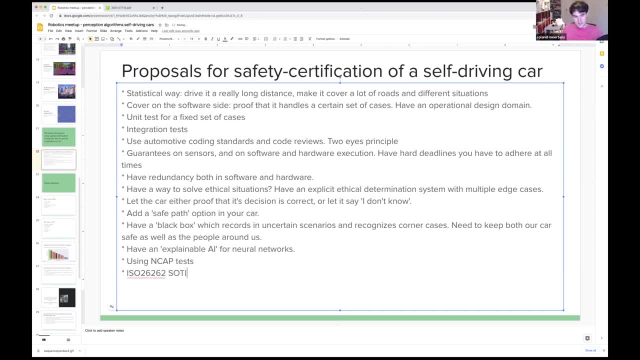 uh. there's also the safety of the intended functionality, so there's also um. there's also another new iso standards that people are working on, um, so there are some practices, uh, which you can use, um which is really interesting. anyways, i will go on with the presentation and 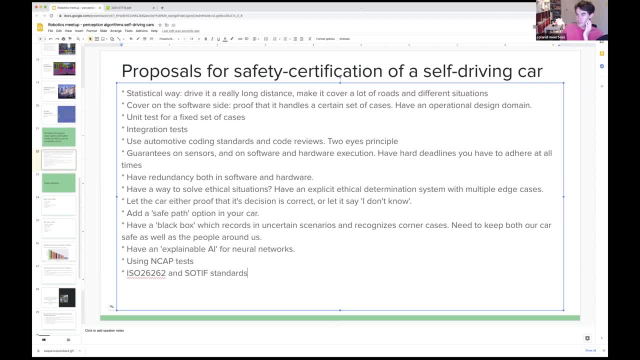 maybe after the presentation i will go on with the presentation and maybe after the presentation, after the meetup, we can have a bit of a longer discussion, if people want, if they like this. i at least really enjoy talking about this and i think all the suggestions are great. 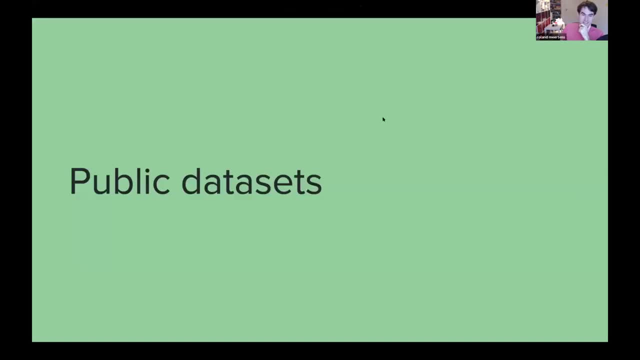 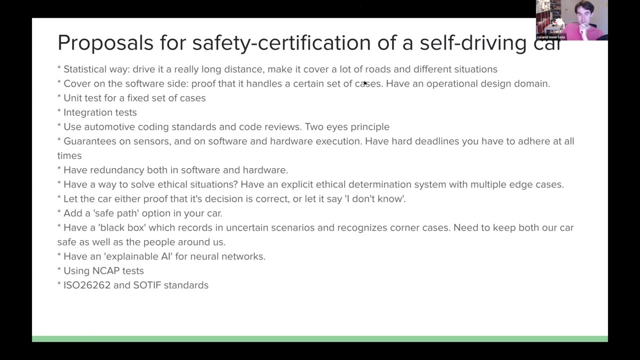 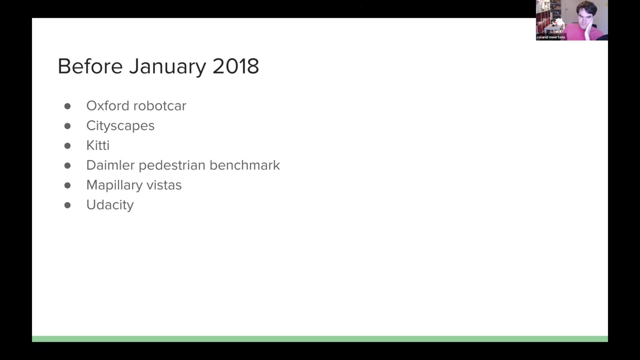 um, but yeah anyways. so i one way of doing it or one thing which people suggested is: uh, prove that henderson's test cases right, or um, prove that it makes certain decisions correct. and i think that, uh, or it starts with kind of data sets. so if you look at public data sets, um, self-driving is already has a big history of self-driving open. 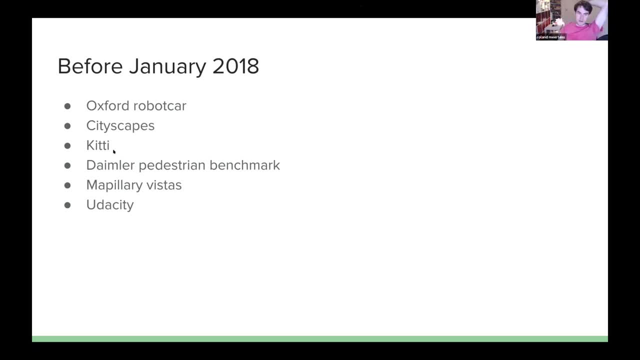 data sets like the kitty data set, which is already a pretty old cityscapes data set, which is still being used a lot, uh, today. uh, there's maybe larry vistas, which is still interesting nowadays. um, and in the last couple of years, there have been many big, massive data sets added for autonomous driving. 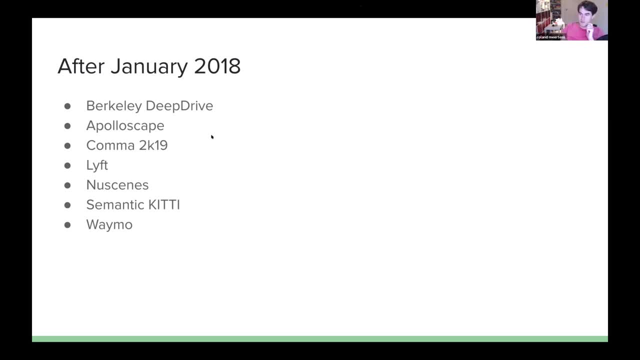 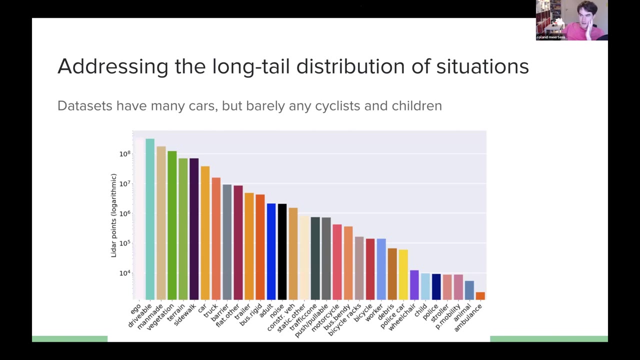 so you've got, for example, the strosky deep drive data set, which is really nice. there's the lift and semantic kitty and bemo data set, which all have loads of bounding boxes and loads of situations. you can train your algorithm, but one thing, which is one maybe a problem for this, is known: validation and the. 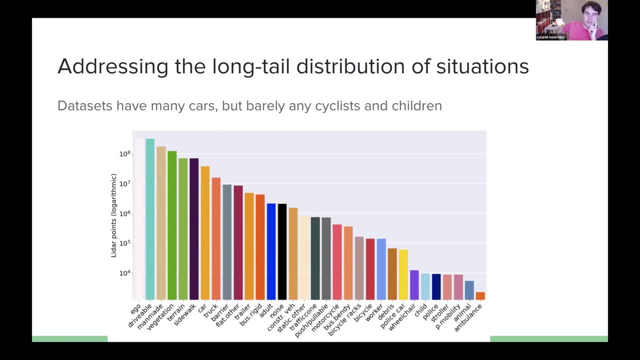 whole validation- self-driving cars on its own- is the fact that data sets are not really balanced. so if you look at- i think this is for the new scenes- uh, counted the points for each class and semantic segmentation, you can see that loads of lighter points hit driveable surface right and there's 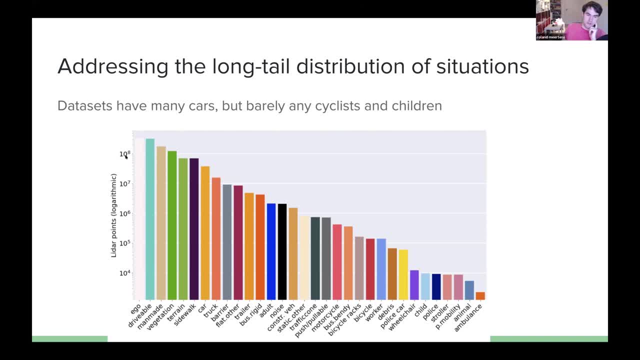 loads of lighter points which hits a car. so this goes logarithmic. so you can see that, for example, there's already more than 10 times the amount of lighter points hitting cars than hitting adults on the road. so it's not that weird. even so, traditionally machine learning algorithms, 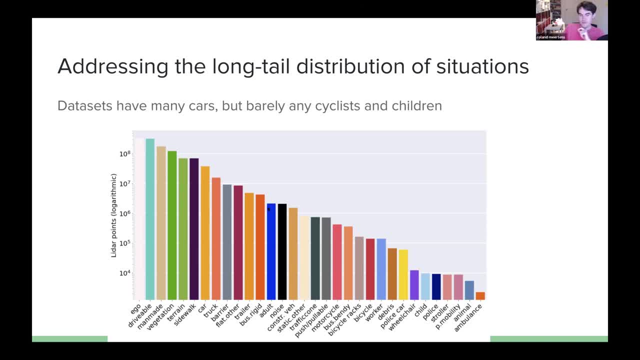 are kind of learning the underlying distribution of data, and the classes which you are training on are really important to have those kind of be the same. so it's not that weird that it's harder to detect pedestrians than detect cars, and if we go further you can see that it's already there's. 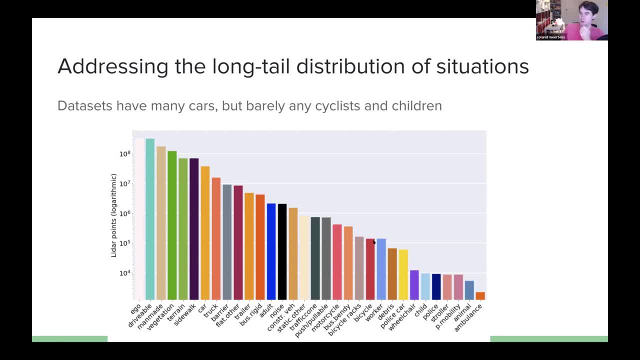 then 10 times the amount of, you can see that it's already. there's then 10 times the amount of points hitting pedestrian than hitting a bicycle. so bicycles are points hitting pedestrian than hitting a bicycle. so bicycles are points hitting pedestrian than hitting a bicycle. so bicycles are already, will already, be harder to. 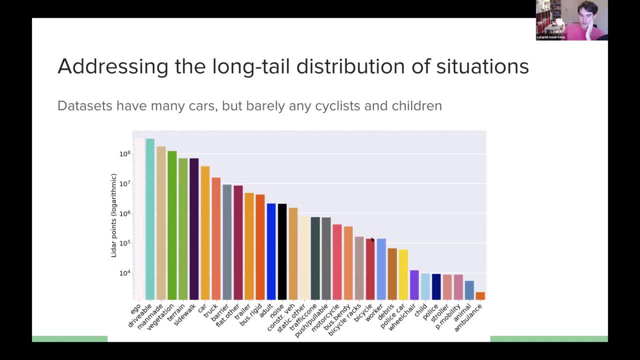 already will already be harder to, already will already be harder to detect and uh detect and uh detect and uh and see then uh and see then uh and see then uh than others if you don't do your data, than others if you don't do your data. 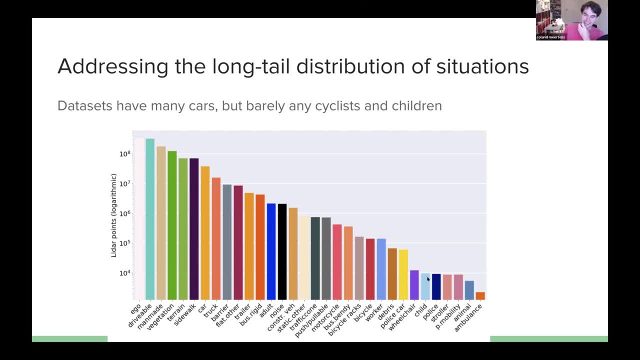 than others if you don't do your data sampling correctly, sampling correctly, sampling correctly. and yeah, children, uh are then more than 10. and yeah, children, uh are then more than 10. and yeah, children, uh are then more than 10 times as unlikely to spot as bicycles. 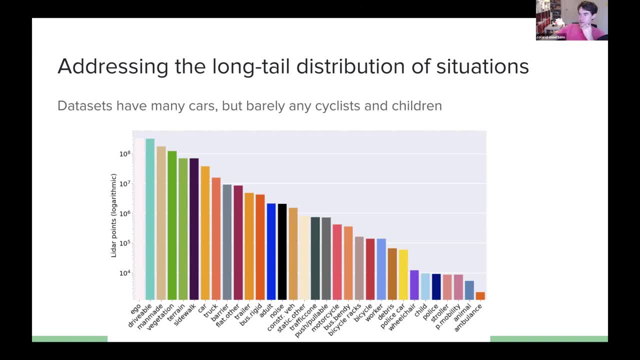 times as unlikely to spot as bicycles, times as unlikely to spot as bicycles. so if you are just naively training in, so if you are just naively training in, so if you are just naively training in our network, on our network, on our network, on whatever data you're just randomly 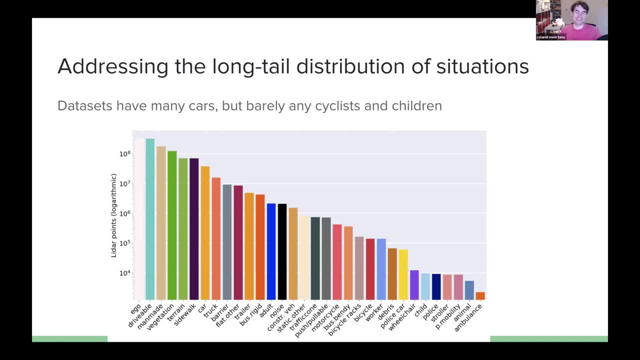 whatever data you're just randomly, whatever data you're just randomly selecting: uh, yeah, you're gonna have a selecting. uh, yeah, you're gonna have a selecting. uh yeah, you're gonna have a bad time. bad time, bad time. to say it in south parkway, um. to say it in south parkway, um. 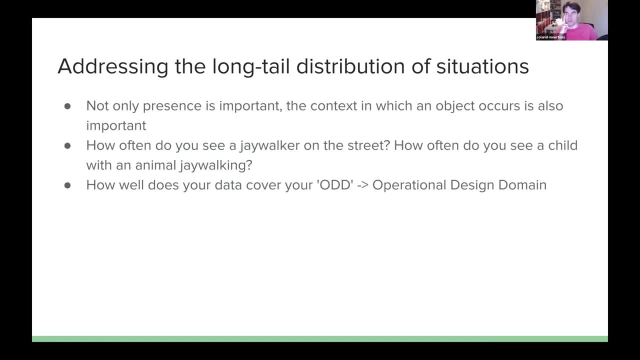 to say it in south parkway, um, and not only is present important, but and not only is present important, but and not only is present important, but the context in which an object occurs is the context in which an object occurs, is the context in which an object occurs is also important. 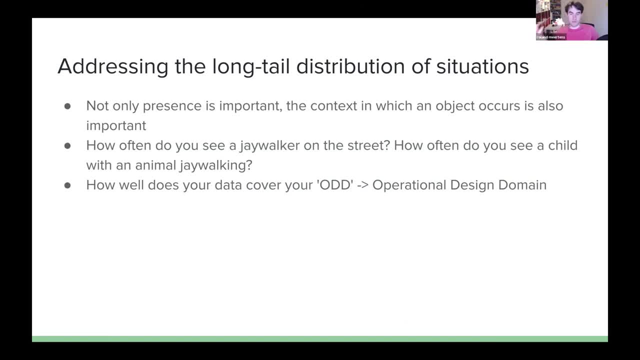 also important, also important. so, uh, how often do you, for example, see so? uh, how often do you, for example, see so? uh, how often do you, for example, see jaywalk on the street? so maybe jaywalk on the street, so maybe jaywalk on the street. so maybe your algorithm could have a. 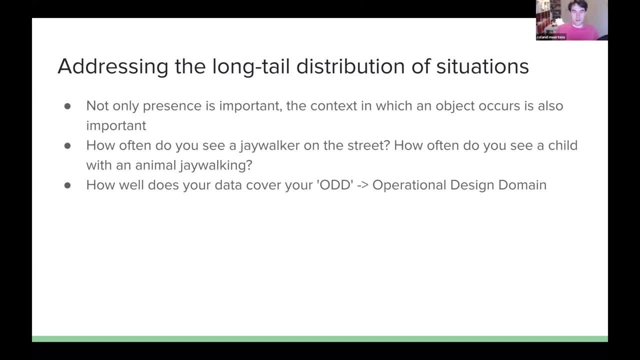 your algorithm could have a. your algorithm could have a kind of a prejudice against saying oh, kind of a prejudice against saying oh, kind of a prejudice against saying, oh, this person is, this person is, this person is: uh, this is a set of points on sidewalk, or? uh, this is a set of points on sidewalk, or? 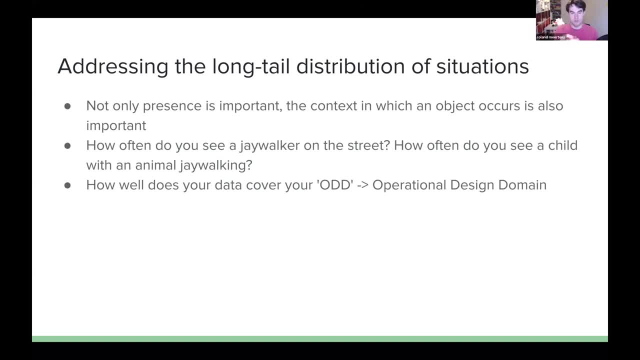 uh, this is a set of points on sidewalk, or there's probably a jaywalker. there's probably a jaywalker. there's probably a jaywalker. oh, there's a set of points, uh, above a. oh, there's a set of points, uh, above a. 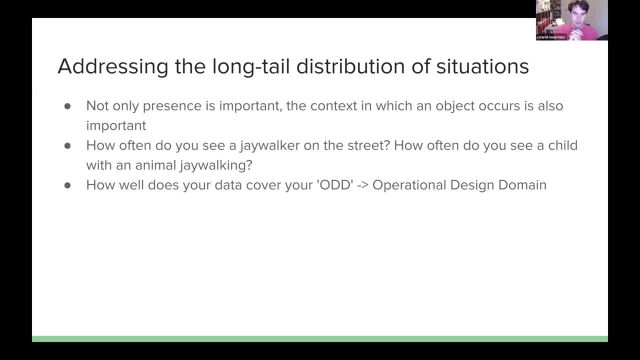 oh, there's a set of points: uh, above a big flat surface, oh, it's probably a car. big flat surface, oh, it's probably a car. big flat surface, oh, it's probably a car. um, and then maybe, how often do you see a um? and then, maybe, how often do you see a? 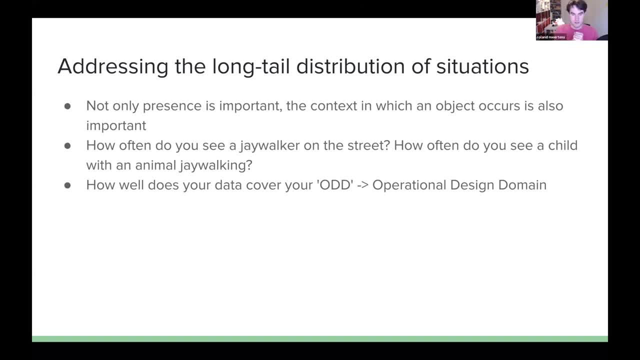 um, and then maybe, how often do you see a chart with animal jaywalking? so all chart with animal jaywalking, so all chart with animal jaywalking. so all these things are situations which are. these things are situations which are. these things are situations which are occurring on a daily basis. 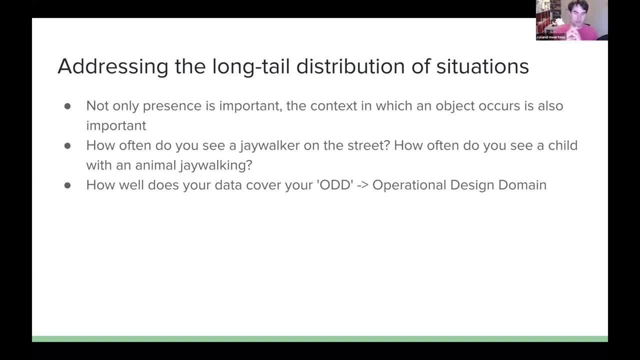 occurring on a daily basis. occurring on a daily basis, um, but it's really important that your um, but it's really important that your um, but it's really important that your data set covers it. data set covers it. data set covers it. so one question one should ask, if one is. so one question one should ask. if one is. so one question one should ask: if one is developing a self-driving car is, hey, how developing a self-driving car is hey, how developing a self-driving car is hey, how well does your data cover your? well, does your data cover your? 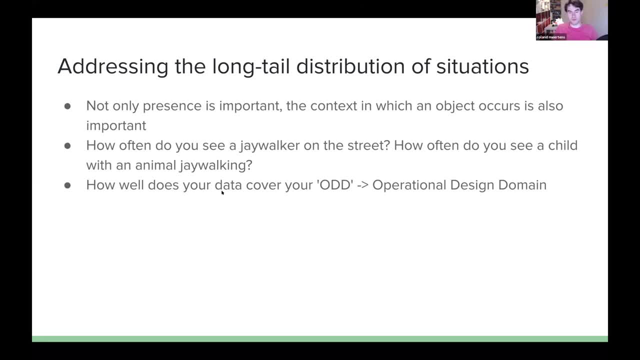 well. does your data cover your operational design domain? do you really operational design domain? do you really operational design domain? do you really need to cover all these situations? do need to cover all these situations. do need to cover all these situations. do you cover, for example, day? you cover, for example, day. 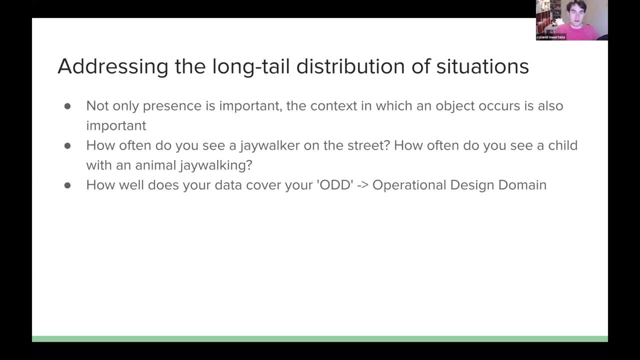 you cover, for example, day and night? do you cover a highway and in a and night? do you cover a highway and in a and night? do you cover a highway? and in a city, city, city, um, and that makes collecting and um, and that makes collecting and um, and that makes collecting and annotating data one of the bigger. 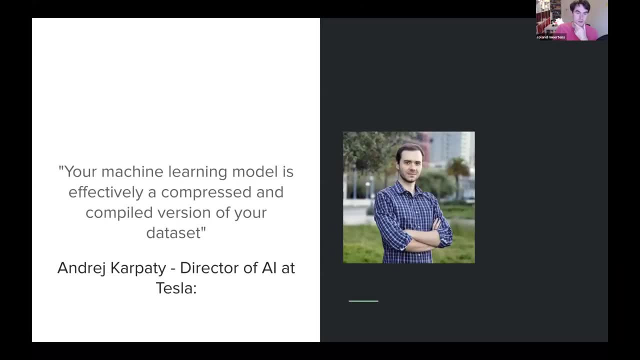 annotating data, one of the bigger annotating data, one of the bigger problems, i think, for now, making autonomous problems. i think, for now making autonomous problems. i think for now making autonomous vehicles, vehicles, vehicles. or to say it as andre kapathy, who's the, or to say it as andre kapathy, who's the, 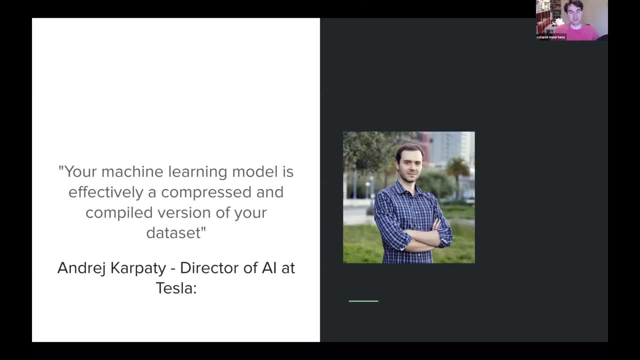 or to say it as andre kapathy, who's the director of director of director of ai tesla: your machine learning model is ai tesla. your machine learning model is basically a compressed and compiled, basically a compressed and compiled, basically a compressed and compiled version of your data set. 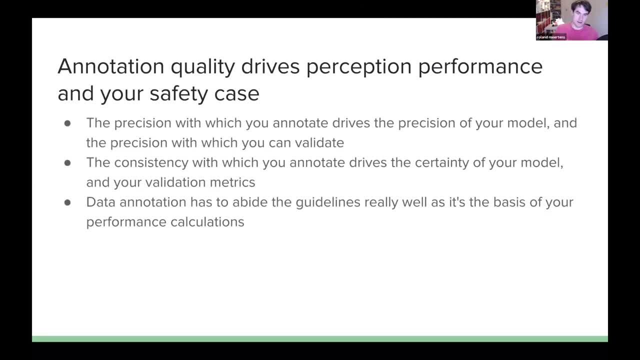 version of your data set. version of your data set. so having a high quality data set. so having a high quality data set. so having a high quality data set which is also balanced, which is also balanced, which is also balanced. that basically drives both your. that basically drives both your. 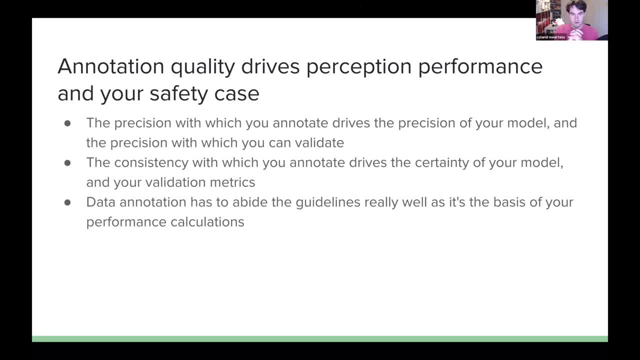 that basically drives both your perception performance and your safety perception performance, and your safety perception performance and your safety case, case, case. so in this case, it's also important that. so in this case, it's also important that. so in this case, it's also important that, for example, the position with which you 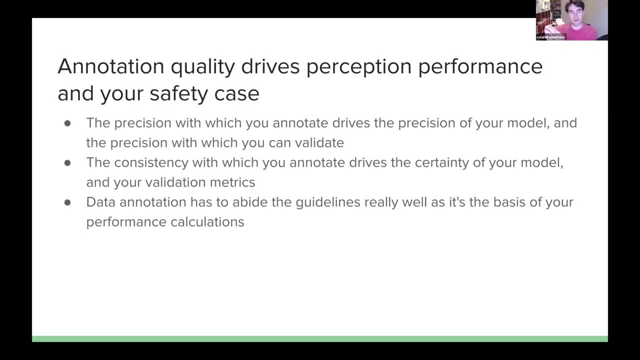 for example, the position with which you, for example, the position with which you annotate, annotate, annotate- drives the precision of your model and drives the precision of your model and drives the precision of your model and the precision with which you annotate. the precision with which you annotate, the precision with which you annotate your vehicles also drive the position. 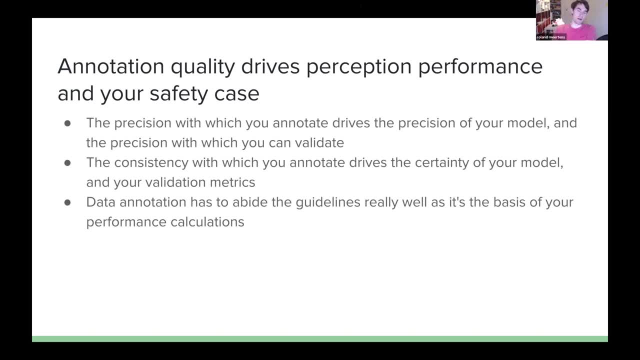 your vehicles also drive the position. your vehicles also drive the position with which you can validate right. so if, with which you can validate right, so if, with which you can validate right, so if you, for example, you, for example, you, for example, are annotating- uh, your bounding boxes. 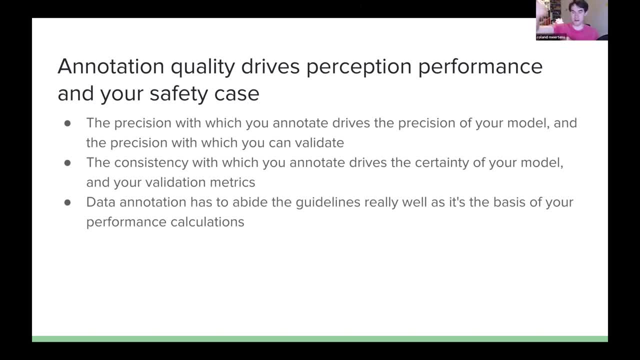 are annotating, uh, your bounding boxes are annotating, uh, your bounding boxes with untrained annotators who are just with untrained annotators who are just with untrained annotators who are just, oh, there's a car, there's a car there. oh, there's a car, there's a car there. 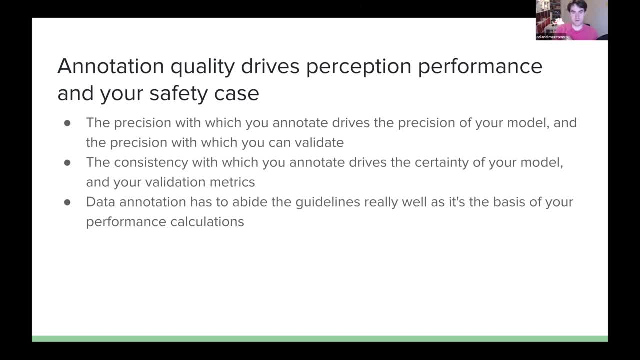 oh, there's a car, there's a car there, that's uh. that means that you can't say that's uh. that means that you can't say that's uh. that means that you can't say anymore: if your algorithm anymore, if your algorithm anymore, if your algorithm a is better than algorithm b, if your 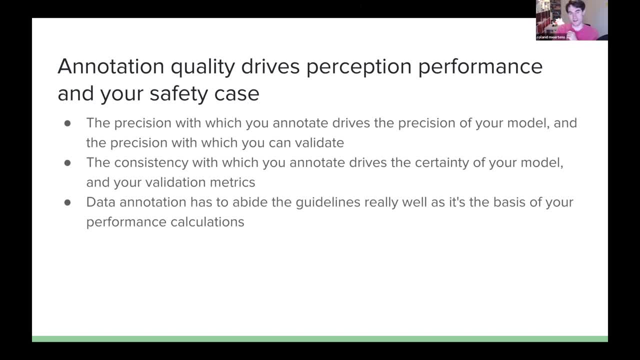 a is better than algorithm b, if your a is better than algorithm b, if your accuracy is not up to. accuracy is not up to. accuracy is not up to- uh, i don't know, uh, uh, i don't know. uh, uh, i don't know, uh, like, if you're, if you're annotating your 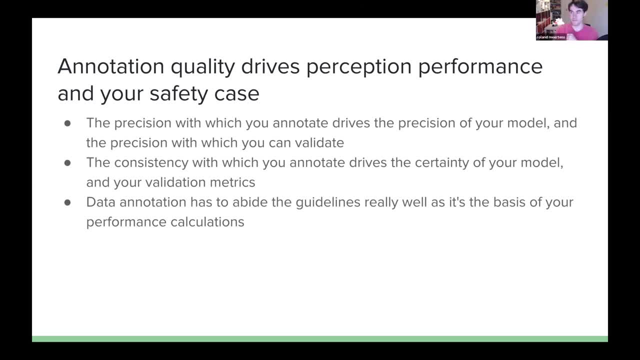 like, if you're, if you're annotating your like, if you're, if you're annotating your uh data with maybe an accuracy of half a uh data, with maybe an accuracy of half a uh data, with maybe an accuracy of half a meter, then you can't. 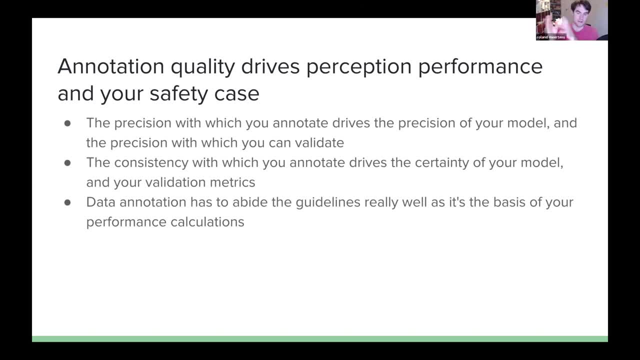 meter, then you can't meter, then you can't have an algorithm which is, or you can't have an algorithm which is, or you can't have an algorithm which is, or you can't validate that your outcome is. validate that your outcome is. validate that your outcome is more accurate than half a meter. 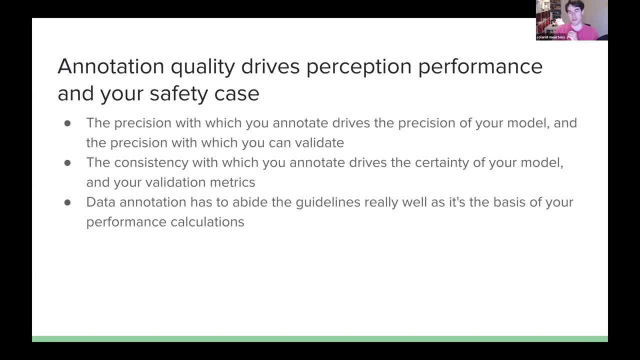 more accurate than half a meter, more accurate than half a meter, and also the consistency with which you and also the consistency with which you and also the consistency with which you annotate, annotate, annotate your data drives, the certainty of the your data drives, the certainty of the your data drives, the certainty of the model. 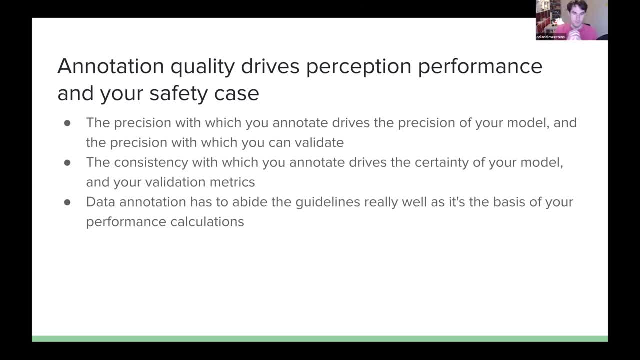 model, model and your validation metrics. so if you and your validation metrics, so if you and your validation metrics, so if you would have a, would have a, would have a um. if you want to see if you're already um. if you want to see if you're already. 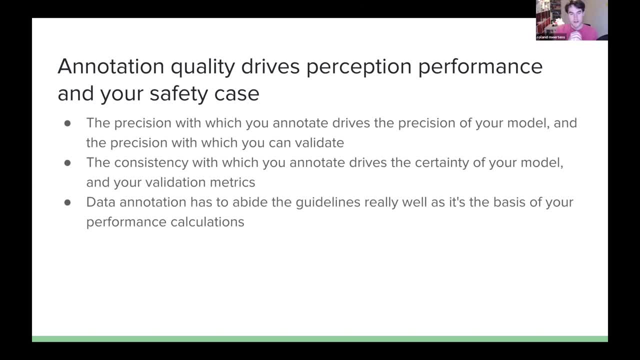 um, if you want to see if you're already detecting all the cars, cars, or detecting all the cars, cars, or detecting all the cars, cars or pedestrians as pedestrians, pedestrians, as pedestrians, pedestrians, um, or maybe you have more edge cases, pedestrians, um, or maybe you have more edge cases where you're defining when something is. 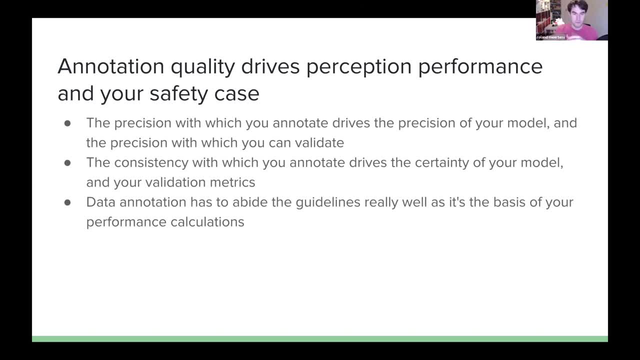 where you're defining when something is, where you're defining when something is a child, or when someone is an adult a child, or when someone is an adult a child, or when someone is an adult. all those things are really important to. all those things are really important to. 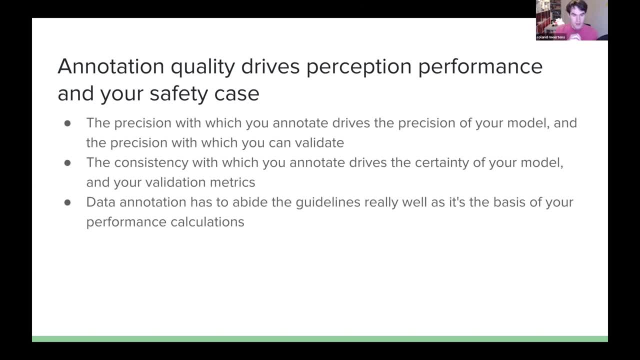 all those things are really important to get across to all your annotators. get across to all your annotators. get across to all your annotators: um, and also those people have to abide um, and also those people have to abide um, and also those people have to abide the guidelines. really well, as it's the 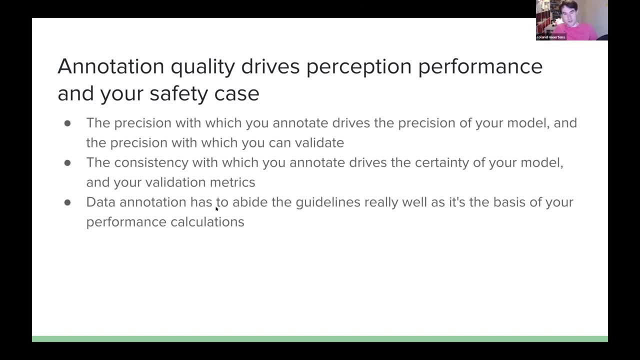 the guidelines really well as it's the the guidelines really well as it's the basics, basics, basics of your performance calculations, so of your performance calculations, so of your performance calculations. so these are things which i'm. these are things which i'm, these are things which i'm thinking a lot about on a daily basis. 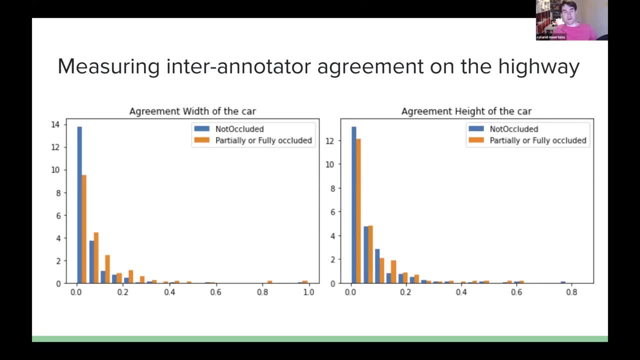 thinking a lot about on a daily basis. thinking a lot about on a daily basis and one maybe fun experiment to quickly, and one maybe fun experiment to quickly, and one maybe fun experiment to quickly. share, share, share, uh. is that we uh? is that we uh is that we took a lot of highway data? 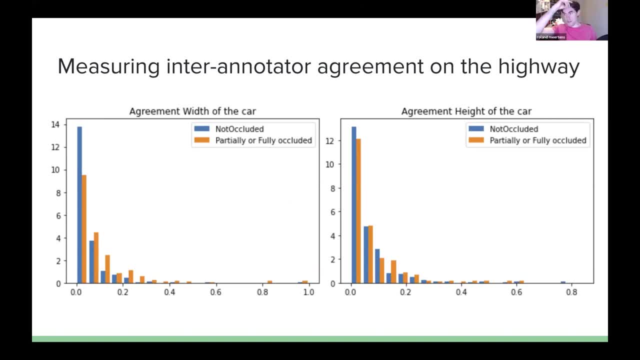 took a lot of highway data, took a lot of highway data, lidar data, and we annotated it twice. so lidar data and we annotated it twice. so lidar data and we annotated it twice. so that's not something you normally see in. that's not something you normally see in. 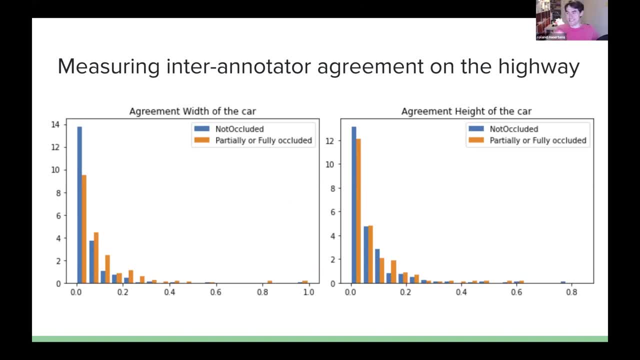 that's not something you normally see in the data set. because people the data set, because people the data set, because people just want to get more, more situations, just want to get more, more situations, just want to get more, more situations, rather than the same data for the same. 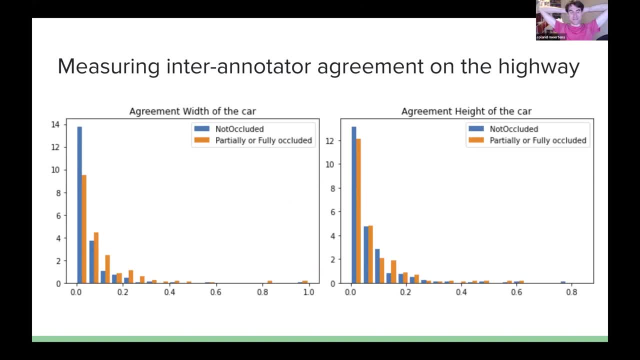 rather than the same data for the same for the same boring stretch of highway, for the same boring stretch of highway, for the same boring stretch of highway, but uh, what we did is? we asked uh, but uh, what we did is we asked uh, but uh, what we did is we asked uh. annotators, okay, how big do you think this? annotators- okay, how big do you think this? annotators? okay, how big do you think this car is how? why do you think this car is car is how? why do you think this car is car is how? why do you think this car is based on slider data and also. 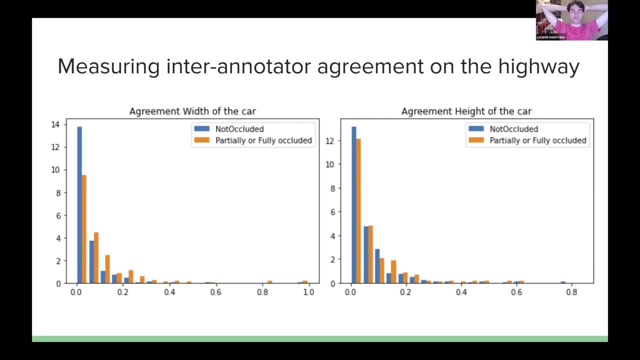 based on slider data and also based on slider data and also let me know if it's uh, maybe a bit. let me know if it's uh, maybe a bit. let me know if it's uh, maybe a bit occluded. so let me know if you can. 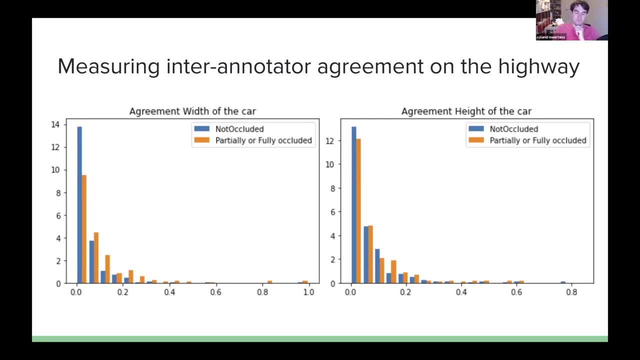 occluded, so let me know if you can. occluded, so let me know if you can really make a decision or not really make a decision, or not really make a decision or not. and we matched- uh, we missed match and we matched. uh, we missed match and we matched. uh, we missed match situations. 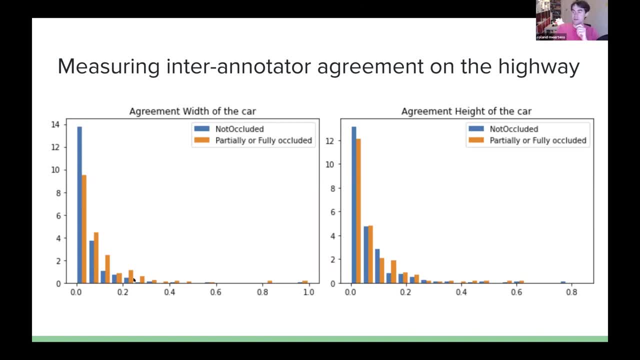 situations, situations, um. you can already see that, for example, um. you can already see that, for example, um. you can already see that, for example, for the width of the vehicle, for the width of the vehicle, for the width of the vehicle on the highway, you'll see loads of. 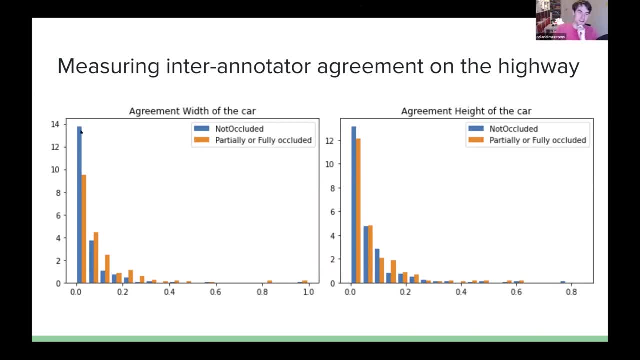 on the highway. you'll see loads of on the highway. you'll see loads of vehicles from behind, vehicles from behind, vehicles from behind. so they're all annotators kind of agree. so they're all annotators kind of agree. so they're all annotators kind of agree. um. 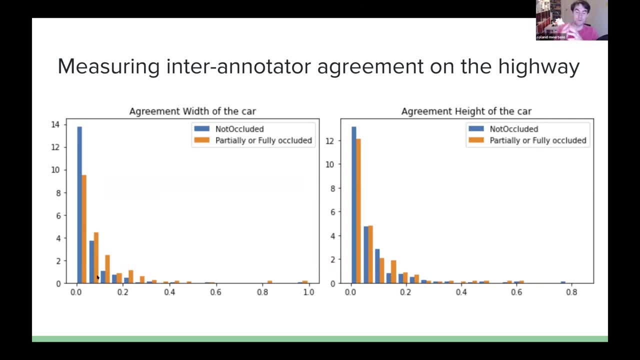 um, um, up to maybe a couple of centimeters. up to maybe a couple of centimeters. up to maybe a couple of centimeters. accuracy, how wide cars are, which is accuracy. how wide cars are, which is accuracy. how wide cars are, which is amazing. and they do it better if they. 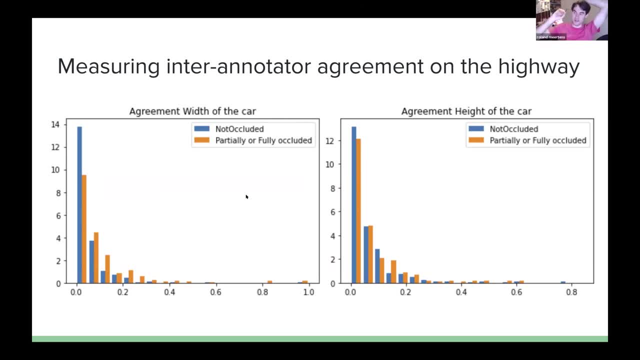 amazing and they do it better if they amazing and they do it better if they objects are not included, and also for objects are not included, and also for objects are not included, and also for the heights, the heights, the heights. objects are really easy to estimate in. objects are really easy to estimate in. 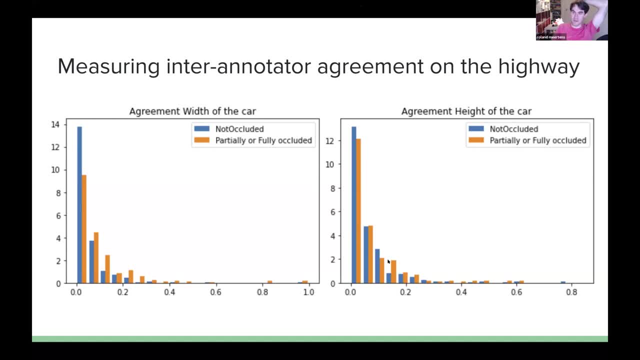 objects are really easy to estimate. in lidar, lidar, lidar, there are people really agree with each. there are people really agree with each. there are people really agree with each other and other and other, and you can see that if you are looking at. you can see that if you are looking at. 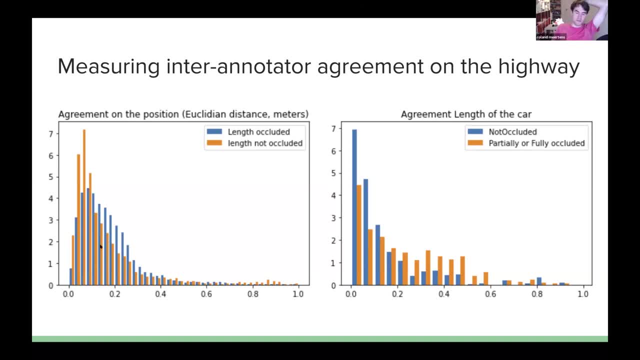 you can see that if you are looking at the center points, the center points, the center points, people already tend to agree. maybe a bit people already tend to agree. maybe a bit people already tend to agree, maybe a bit less, less, less, especially for the, especially for the. 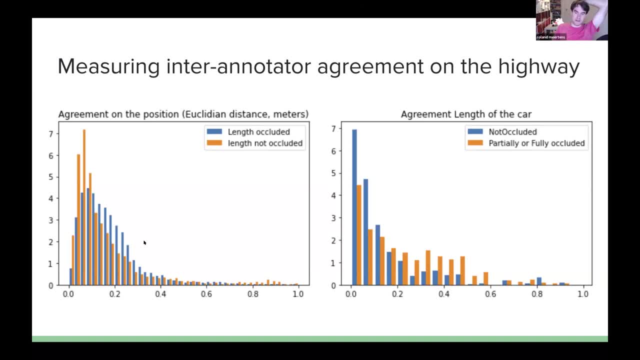 especially for the occluded vehicles. occluded vehicles, occluded vehicles- it's uh, it's uh, it's uh. it's a bit harder to estimate where exactly. it's a bit harder to estimate where exactly. it's a bit harder to estimate where exactly the center is if you don't know exactly. 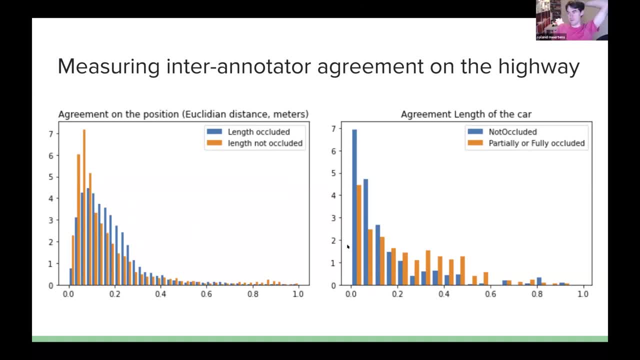 the center is if you don't know exactly the center is, if you don't know exactly how long a vehicle is, how long a vehicle is, how long a vehicle is, and also for the length of the vehicle, and also for the length of the vehicle and also for the length of the vehicle in lidar, you can't if you see an object. 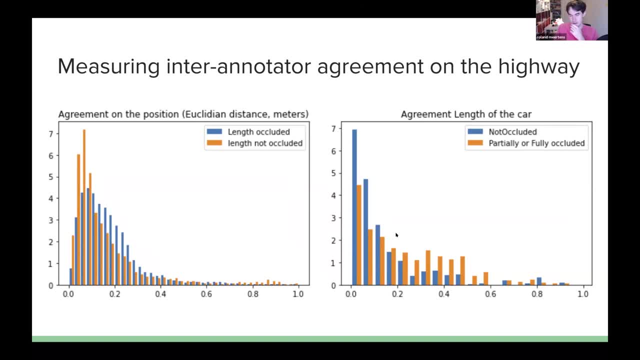 in lidar. you can't. if you see an object in lidar, you can't. if you see an object from behind, you can't really say how from behind you can't really say how long it is. you can see that long it is. you can see that. 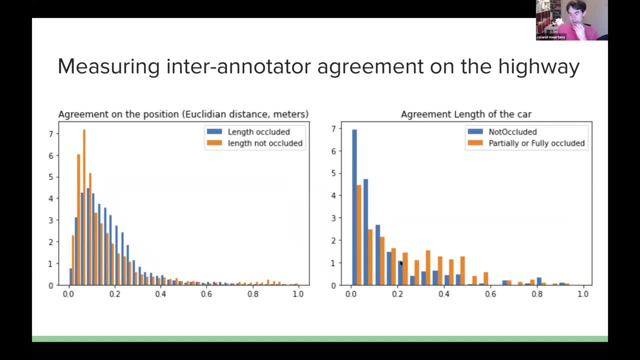 long it is. you can see that. we also see that the. we also see that the. we also see that the accuracy then maybe drops where accuracy then maybe drops where accuracy then maybe drops where everyone agrees up to like 50 centimeters. everyone agrees up to like 50 centimeters. 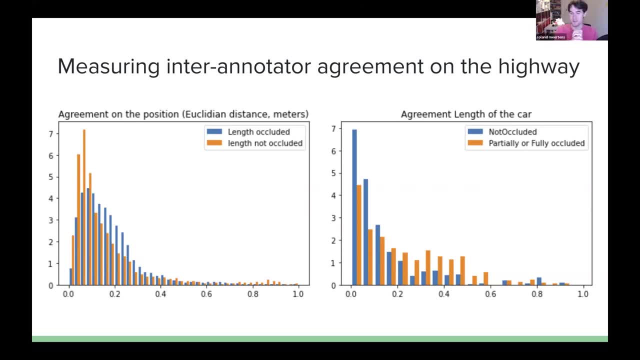 everyone agrees, up to like 50 centimeters, how long and how long and how long and how long a car is, uh, but it's not this: how long and how long a car is, uh, but it's not this: how long and how long a car is, uh, but it's not this clear. oh, it's. 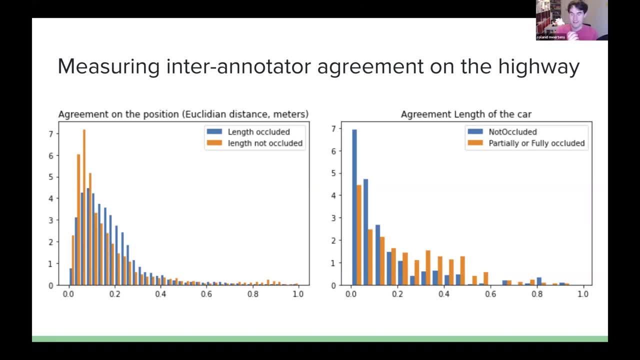 clear. oh, it's clear. oh, it's five, five or ten centimeters accurate. five, five or ten centimeters accurate. five, five or ten centimeters accurate. but it also means that if you're if, but it also means that if you're if, but it also means that if you're if you're writing an algorithm on this, uh, 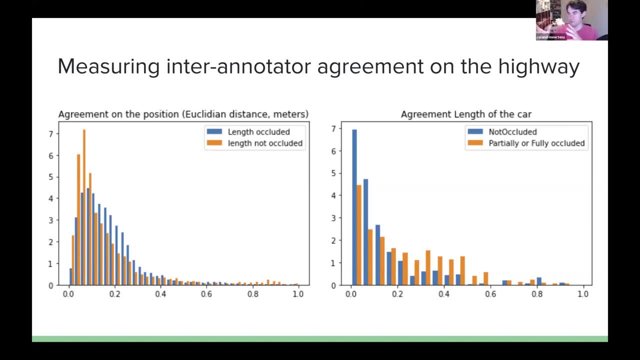 you're writing an algorithm on this. uh, you're writing an algorithm on this. uh, training data, training data, training data. you can't say anymore, oh, this algorithm. you can't say anymore, oh this algorithm. you can't say anymore, oh, this algorithm is good or bad if it's uh, performing um. 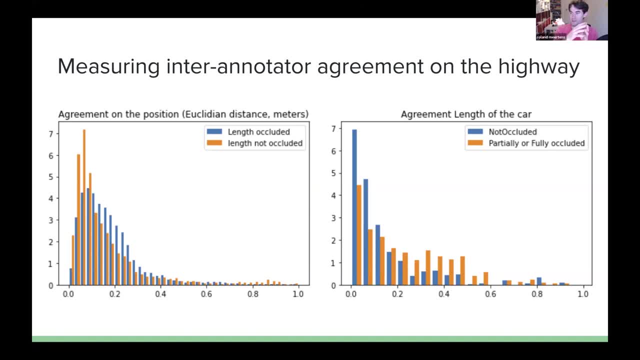 is good or bad if it's uh performing um is good or bad if it's uh performing um. like can only kind of compare this, like can only kind of compare this, like can only kind of compare this algorithm to algorithm to algorithm to the same annotated or annotated data. 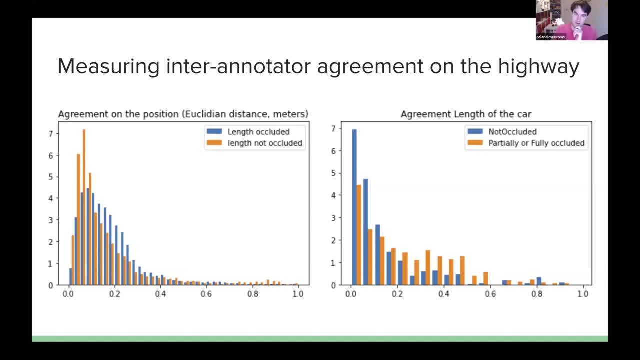 the same annotated or annotated data. the same annotated or annotated data twice. to see if your algorithm is a twice. to see if your algorithm is a twice. to see if your algorithm is a human-like precision or not. um human-like precision or not. um human-like precision or not. um, so yeah, and then maybe the last thing. 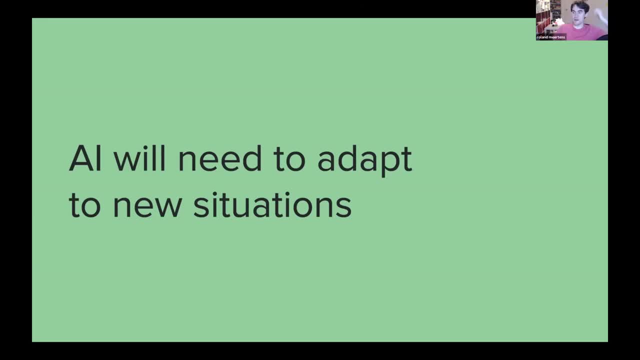 so yeah, and then maybe the last thing, so yeah, and then maybe the last thing which i think is interesting, uh, about which i think is interesting, uh about which i think is interesting, uh about kind of the data labeling or annotation, kind of the data labeling or annotation. 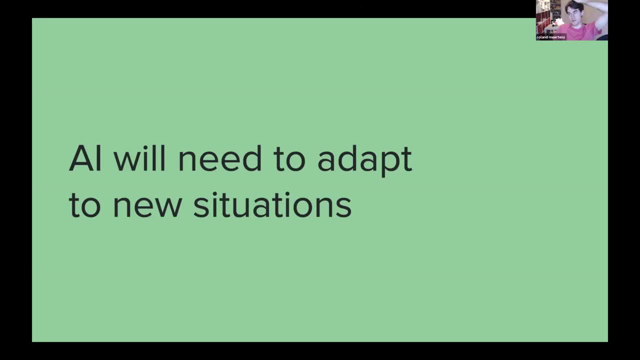 kind of the data labeling or annotation. business, business, business. is that ai will need to adapt to new? is that ai will need to adapt to new? is that ai will need to adapt to new situations? right, so we often think about situations, right so we often think about. 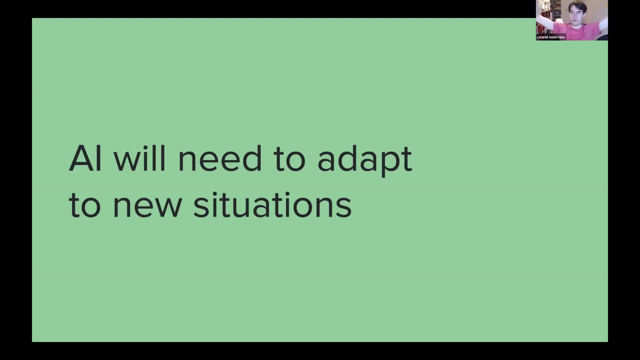 situations right. so we often think about: oh, let's just build a robot and release. oh, let's just build a robot and release. oh, let's just build a robot and release it in the world and we'll kind of just it in the world and we'll kind of just. 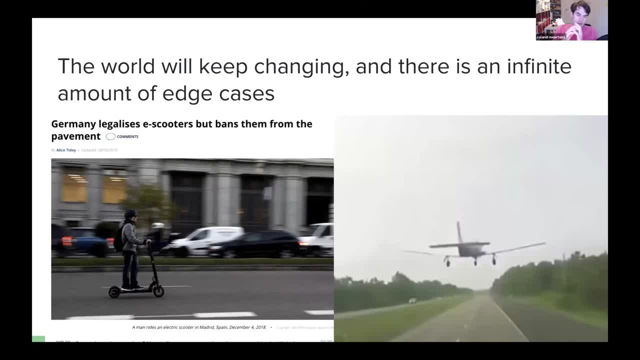 it in the world and we'll kind of just keep doing this task, keep doing this task, keep doing this task, but especially uh for robot taxis, the, but especially uh for robot taxis, the, but especially uh for robot taxis. the world will keep changing. world will keep changing. 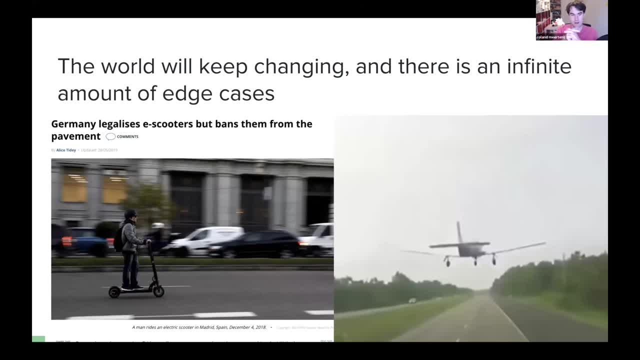 world will keep changing. and there's an infinite amount of edge and there's an infinite amount of edge and there's an infinite amount of edge cases. so here in germany, cases, so here in germany, cases. so here in germany, already two years ago we got those. already two years ago we got those. 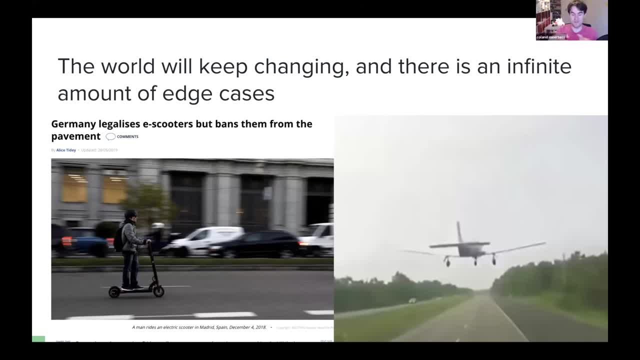 already two years ago we got those e-scooters, e-scooters, e-scooters, and they were not allowed to drive on and they were not allowed to drive on and they were not allowed to drive on the pavement, so they had to drive on the. 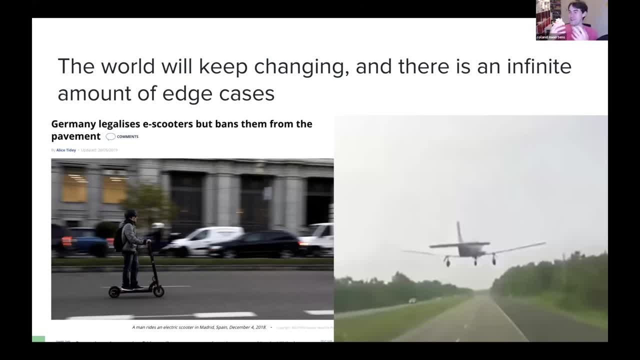 the pavement, so they had to drive on the the pavement, so they had to drive on the roads, roads, roads. so you can guess, uh, who was driving our. so you can guess, uh, who was driving our. so you can guess, uh, who was driving our. recording vehicle, recording vehicle. 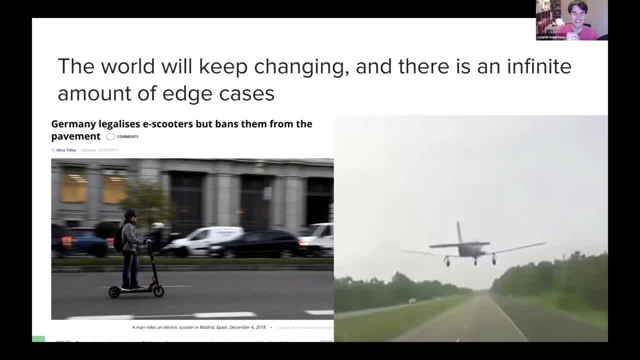 recording vehicle that day to catch all the situations that day, to catch all the situations that day, to catch all the situations because, suddenly, because, suddenly, because, suddenly, uh like the tiny thin objects which were, uh like the tiny thin objects which were, uh like the tiny thin objects which were normally classified as pedestrians were. 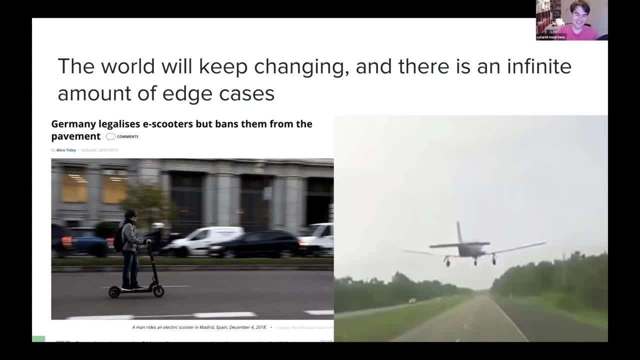 normally classified as pedestrians were, normally classified as pedestrians were going at 20 or 30 kilometers an hour, going at 20 or 30 kilometers an hour, going at 20 or 30 kilometers an hour over the roads, over the roads, over the roads, but yeah, so this is that's like a real 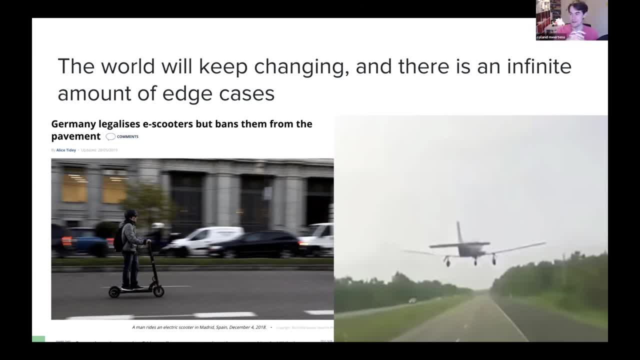 but yeah, so this is that's like a real, but yeah, so this is that's like a real life case of life, case of life, case of uh, which i guess is maybe pretty uh, which i guess is maybe pretty uh, which i guess is maybe pretty solvable, because we knew this and we 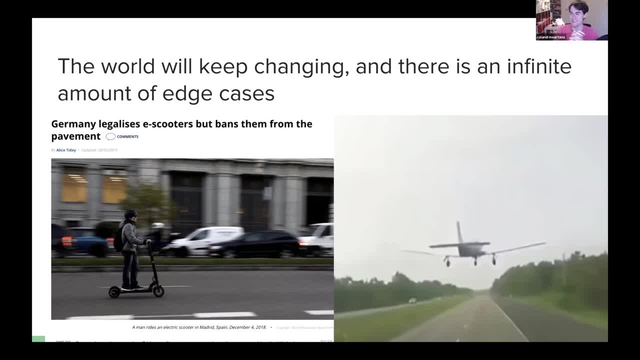 solvable because we knew this and we solvable because we knew this and we could take our recording vehicle and could take our recording vehicle and could take our recording vehicle and drive around and collect way more drive around and collect way more drive around and collect way more information and way more data. and 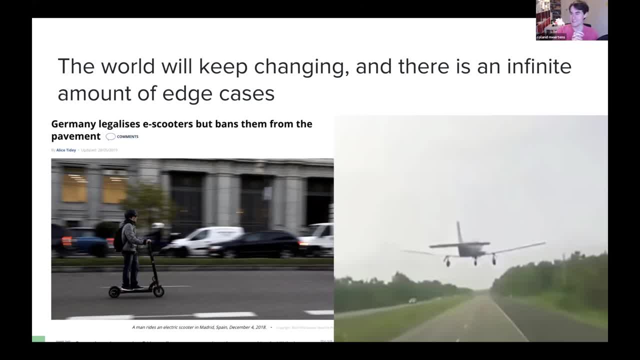 information and way more data and information and way more data and quickly label that, quickly label that, quickly label that. but there's also edge cases which you are. but there's also edge cases which you are, but there's also edge cases which you are never really seeing, like if there's a 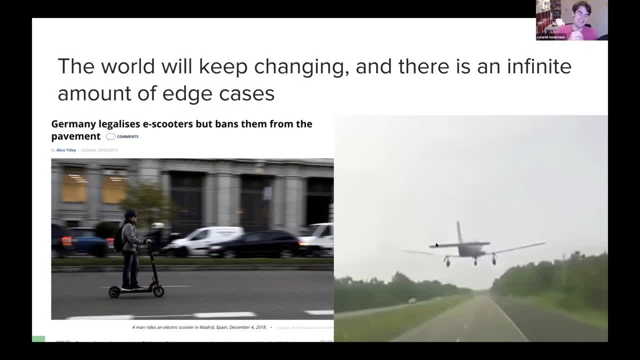 never really seeing like if there's a. never really seeing like if there's a plane landing, plane landing, plane landing. uh, you and i, you know, we all know, uh, uh, you and i, you know, we all know, uh, uh, you and i, you know, we all know, uh, this is uh, that's bad news, if you see. this is- uh, that's bad news if you see. this is- uh, that's bad news if you see it in front of you. so you keep loads of it in front of you. so you keep loads of it in front of you. so you keep loads of distance. 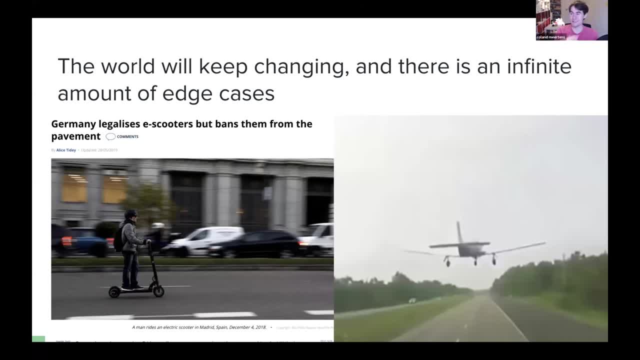 distance, distance, but for your self-driving car they never. but for your self-driving car, they never. but for your self-driving car, they never see this, or they maybe see this, or they maybe see this, or they maybe. entire features is only once and it's entire features is only once and it's. 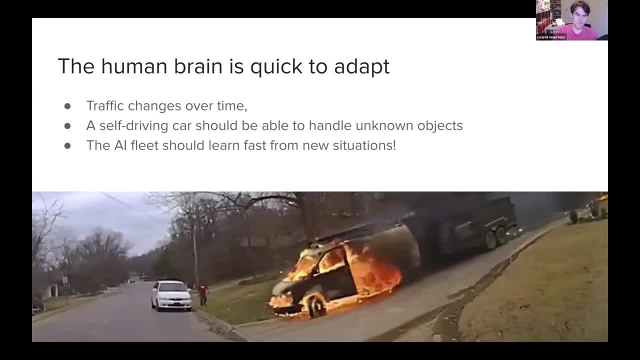 entire features is only once, and it's really important. you're able to really important. you're able to really important. you're able to handle this um and maybe also the human handle this um, and maybe also the human handle this um, and maybe also the human brain is quick to adapt. so this is a 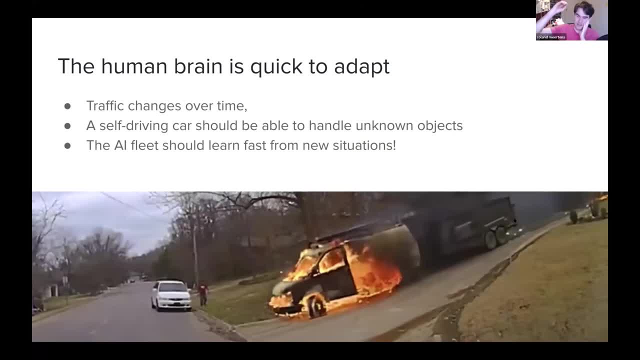 brain is quick to adapt, so this is a brain is quick to adapt, so this is a snapshot from a video where this car is snapshot, from a video where this car is snapshot, from a video where this car is on fire and on fire, and on fire, and it's um, at some point the brakes break. 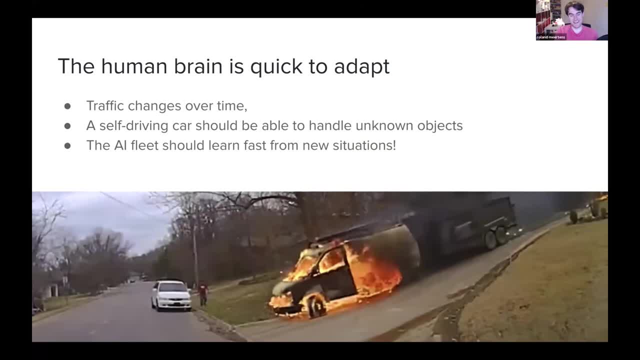 it's um at some point the brakes break. it's um at some point the brakes break, so it comes burning down this hill. so it comes burning down this hill. so it comes burning down this hill and uh, even though normally uh, if you if, and uh, even though normally uh, if you if. 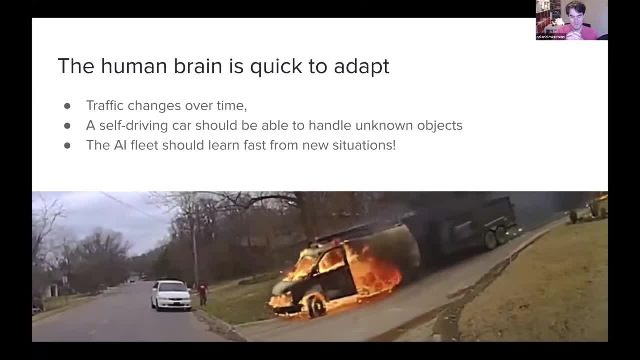 and uh, even though normally, uh, if you, if this was a view from a self-driving, this was a view from a self-driving, this was a view from a self-driving car, car, car, um, you would think, ah, it is my right of um, you would think, ah, it is my right of. 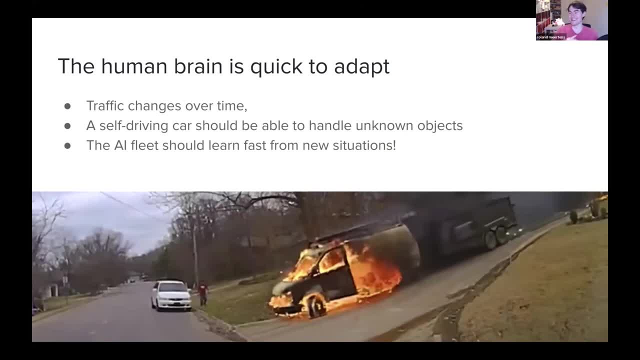 um, you would think, ah, it is my right of way, way, way. but we, as a human, know that this car. but we, as a human, know that this car, but we, as a human, know that this car which is on fire and coming down, the, which is on fire and coming down, the. 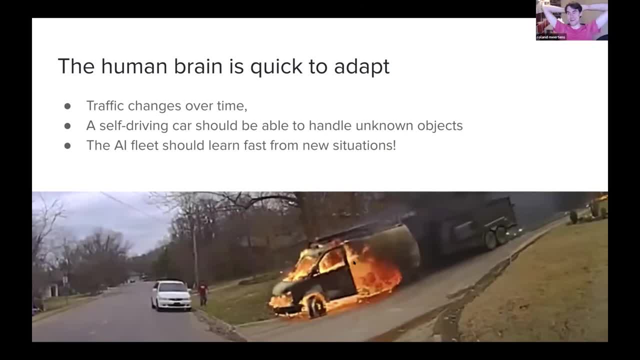 which is on fire and coming down the hill, is not going to give you right of hill, is not going to give you right of hill, is not going to give you right of way, way, way. so i like, as a human, we are kind of. so i like, as a human, we are kind of. 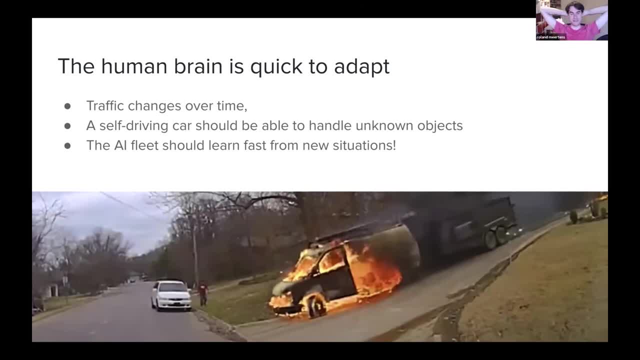 so i like as a human, we are kind of making loads of assumptions, making loads of assumptions, making loads of assumptions, um, and a self-driving car fleet should um, and a self-driving car fleet should um, and a self-driving car fleet should also be able to handle. 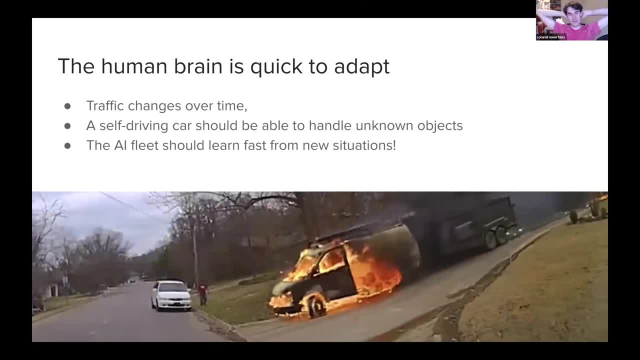 also be able to handle, also be able to handle unknown objects and other situations. unknown objects and other situations. unknown objects and other situations. um so yeah, traffic changes over time. um so yeah, traffic changes over time. um so yeah, traffic changes over time. think about those, uh. think about those uh. 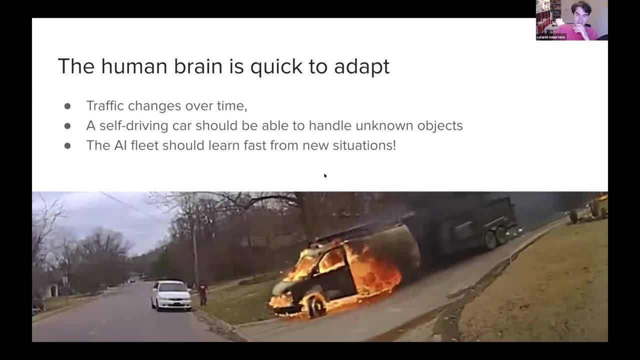 think about those uh, e-scooters finally, or sometimes e-scooters finally, or sometimes e-scooters finally, or sometimes suddenly popping up, suddenly popping up, suddenly popping up, and i think an ai fleet should learn, and i think an ai fleet should learn and i think an ai fleet should learn fast from new situations, because new. 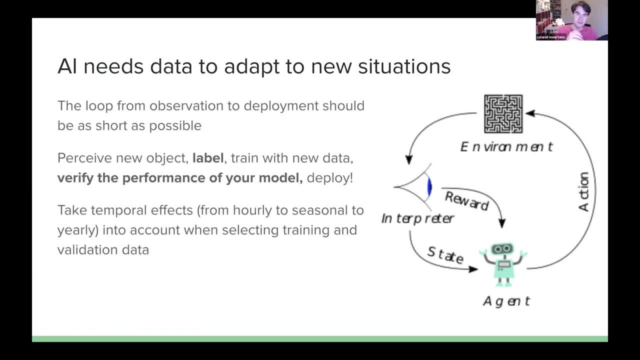 fast from new situations because new. fast from new situations, because new situations will pop up on a daily basis. situations will pop up on a daily basis. situations will pop up on a daily basis. so your so, your so, your ai, or your loop from observing, ai, or your loop from observing. 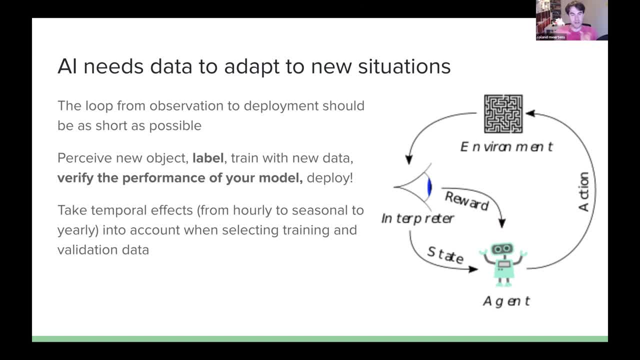 ai, or your loop, from observing a new weird or interesting situation- a new weird or interesting situation- a new weird or interesting situation- to deploying a model should be as short. to deploying a model should be as short. to deploying a model should be as short as possible. so if you perceive a new, 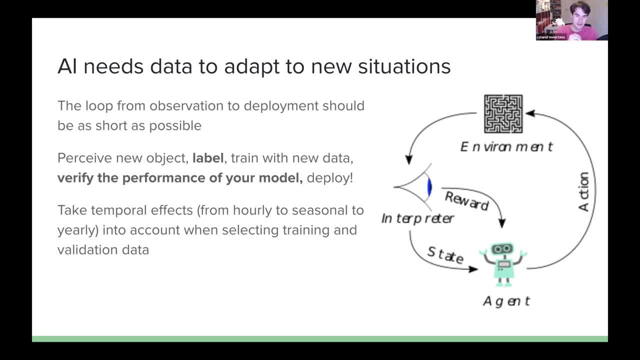 as possible. so if you perceive a new, as possible. so if you perceive a new object, you should be able to label it. object: you should be able to label it. object: you should be able to label it super quickly, super quickly, super quickly. retrain your model with new data. 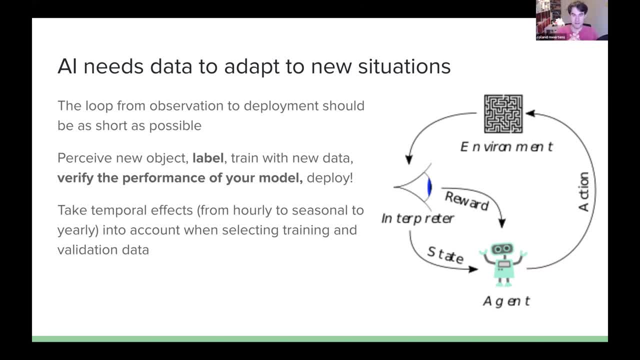 retrain your model with new data. retrain your model with new data. verify the performance of your model. we verify the performance of your model. we verify the performance of your model. we talked about that before right. did you talked about that before right? did you talked about that before right? did you make sure that everything is still okay? 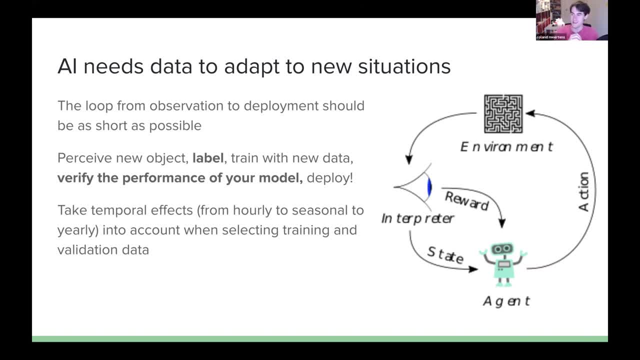 make sure that everything is still okay. make sure that everything is still okay. that maybe your explainable ai. that maybe your explainable ai. that maybe your explainable ai. someone suggested that, someone suggested that. someone suggested that still has the right explainability and still has the right explainability, and. 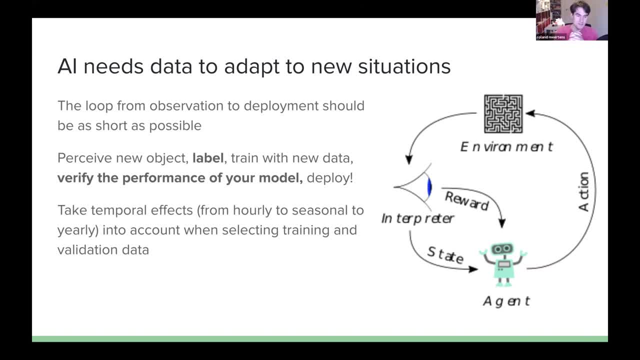 still has the right explainability and then you can deploy it, then you can deploy it, then you can deploy it and make sure that you take temporal and make sure that you take temporal and make sure that you take temporal effects from maybe hourly effects from maybe hourly. 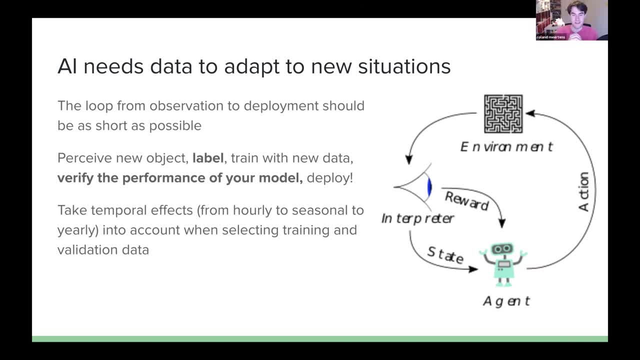 effects from maybe hourly effects to maybe seasonal or yearly. so effects to maybe seasonal or yearly. so effects to maybe seasonal or yearly. so maybe, maybe, maybe in winter, unless people are using e in winter, unless people are using e in winter, unless people are using e scooters in the summer. 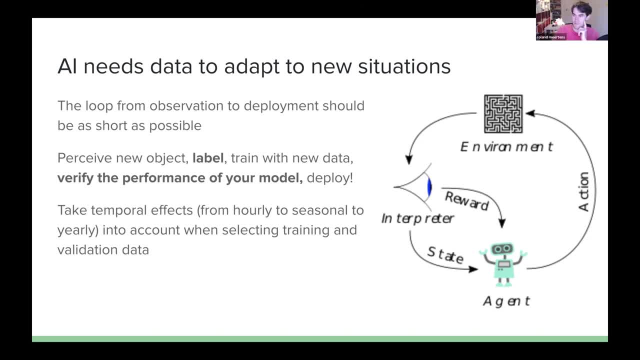 scooters in the summer: scooters in the summer. make sure that you all take this into. make sure that you all take this into account when selecting training and account when selecting training and account when selecting training. and validation, data validation, data validation data. um so yeah, we went over the levels of 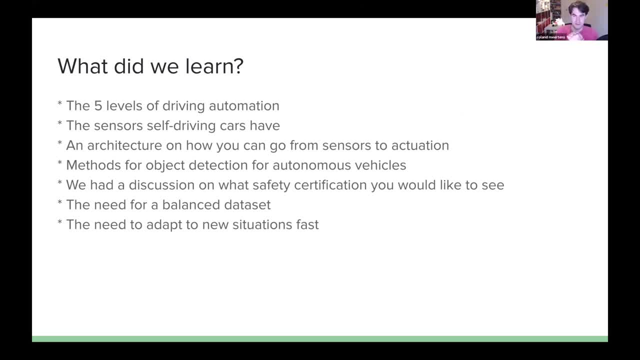 um. so yeah, we went over the levels of. um so yeah, we went over the levels of driving automations. we went over the driving automations. we went over the driving automations. we went over the sensors. we went over an architecture of sensors. we went over an architecture of. 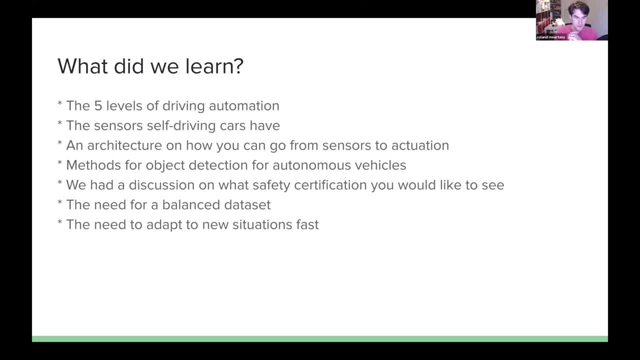 sensors. we went over an architecture of how you can go to. how you can go to how you can go to actuation- we uh actuation, we uh actuation, we uh went over some over a couple of methods, went over some over a couple of methods, went over some over a couple of methods, and we had a discussion on what safety. 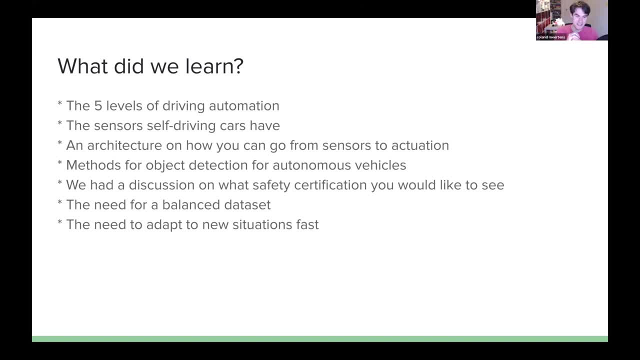 and we had a discussion on what safety, and we had a discussion on what safety verification you would like to see verification. you would like to see verification. you would like to see, uh, the need for a balanced data set and uh, the need for a balanced data set, and. 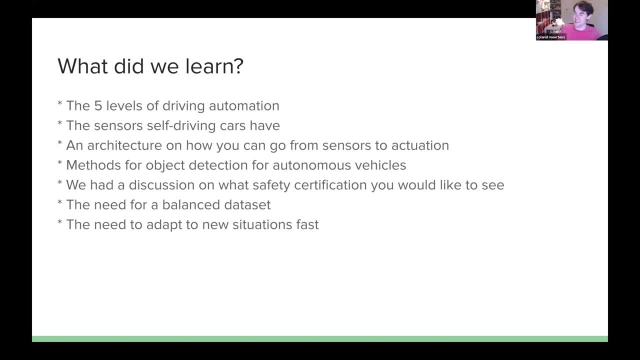 uh, the need for a balanced data set and new to new. there needs to adapt to new, new to new. there needs to adapt to new, new to new. there needs to adapt to new situations, situations, situations. so, if people have questions or want to. so, if people have questions or want to, 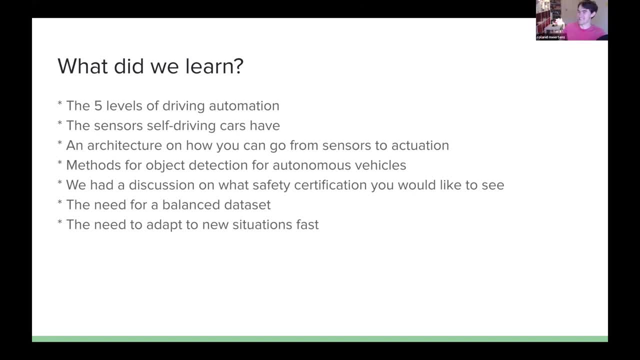 so if people have questions or want to continue a discussion, continue a discussion, continue a discussion. let me know. i already see one hand raised. i already see one hand raised. i already see one hand raised. yeah, i think you can admit yourself, uh. yeah, i think you can admit yourself, uh. 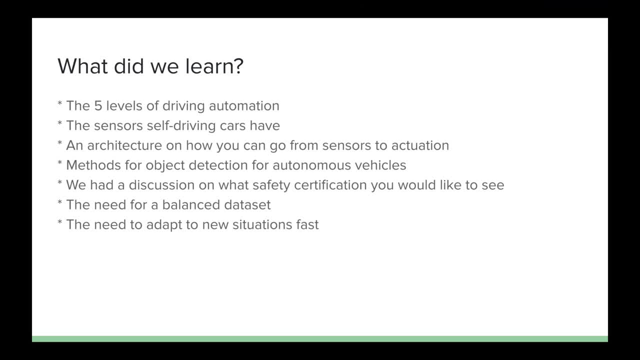 yeah, i think you can admit yourself: uh, it's pos, it's pos, it's pos, it should be possible, so just go ahead. it should be possible, so just go ahead. it should be possible, so just go ahead. yeah, hi, thank you for the time um so. yeah, hi, thank you for the time um so. 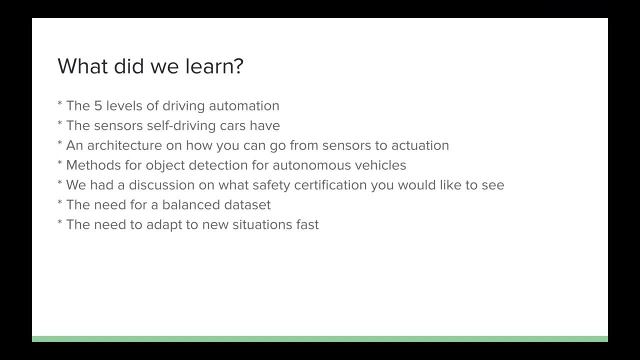 yeah, hi, thank you for the time. um, so, i've just also popped in the question. i've just also popped in the question. i've just also popped in the question, just in case. just in case, just in case. uh, people are not able to capture that. uh, people are not able to capture that. 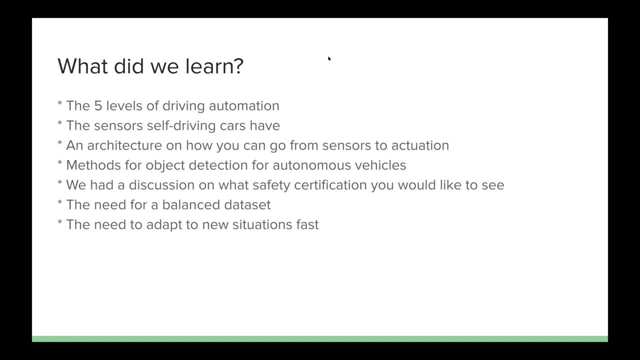 uh, people are not able to capture that. so right now we see a lot of data sets. so right now we see a lot of data sets. so right now we see a lot of data sets coming up from coming up, from coming up from both corporates as well as on the 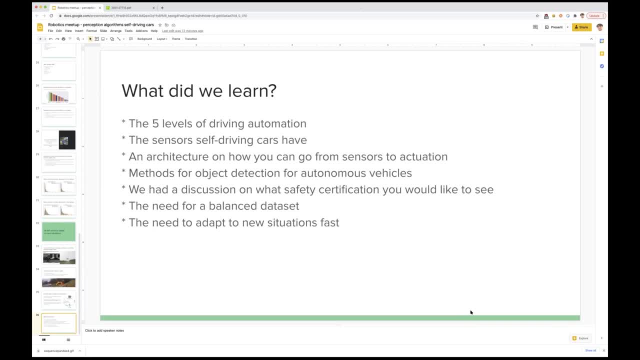 both corporates as well as on the both corporates as well as on the research front, research front, research front: uh like waymo kitty or aptiv. uh like waymo kitty or aptiv. uh like waymo kitty or aptiv. and even as old as oxford data set. 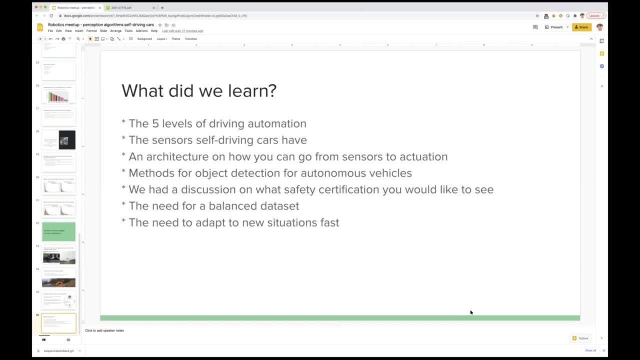 and even as old as oxford data set and even as old as oxford data set and things like that and things like that and things like that um being an active. you know um person who's um being an active. you know um person who's um being an active. you know um person who's interested in these. 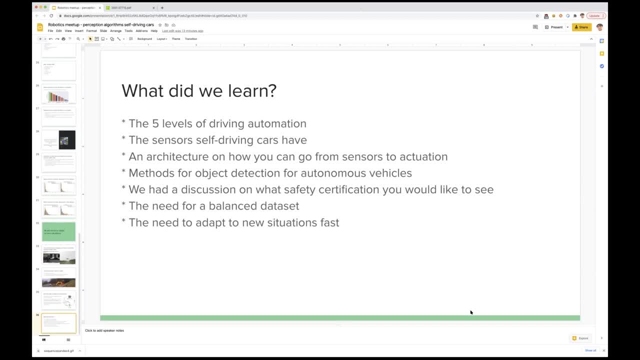 interested in these, interested in these topics. uh, i find that when you move topics, uh, i find that when you move topics, uh, i find that when you move across one particular data set to the across, one particular data set to the across, one particular data set to the other, there is no particular standard. 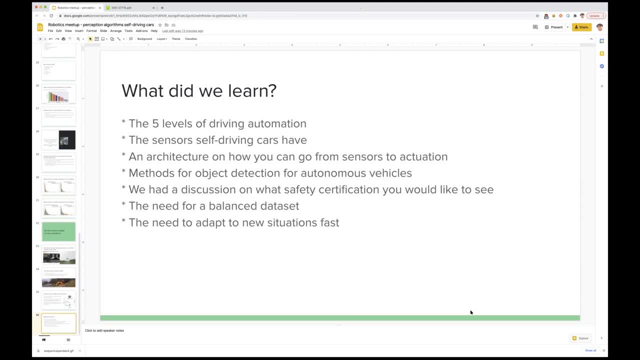 other, there is no particular standard. other, there is no particular standard. that's being, that's being, that's being carried out. um in in different levels. i carried out um in in different levels. i carried out um in in different levels. i completely agree that the sensor usage. 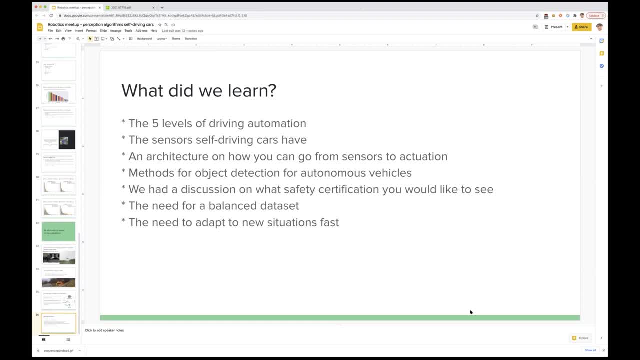 completely agree that the sensor usage, completely agree that the sensor usage or the count of the sensors can be, or the count of the sensors can be, or the count of the sensors can be different, different, different. but um in terms of uh the ground, but um in terms of uh the ground. 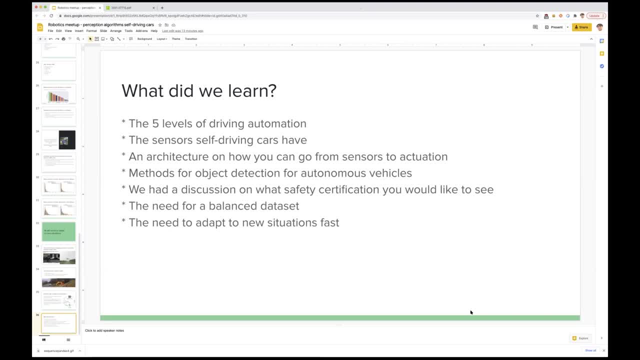 but, um, in terms of, uh, the ground, fundamental understanding, if it's a fundamental understanding, if it's a fundamental understanding if it's a camera image, camera image, camera image, for example, and if you're doing, or, for example, and if you're doing, or, for example, and if you're doing or generating data sets for a 2d object. 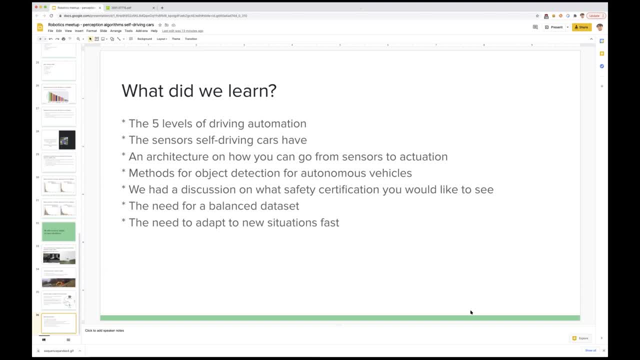 generating data sets for a 2d object. generating data sets for a 2d object: detection, detection, detection, then the formatting or the annotation, then the formatting or the annotation, then the formatting or the annotation scheme. scheme is not universal across different places. is not universal across different places. 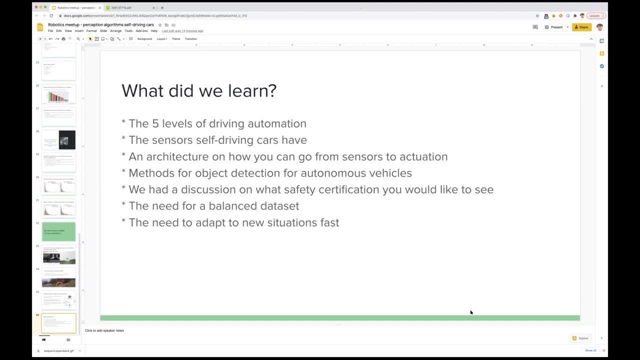 is not universal across different places, and this and this and this, um, i personally feel that takes in a lot. um, i personally feel that takes in a lot. um, i personally feel that takes in a lot of time to first get the understanding of of time, to first get the understanding of. 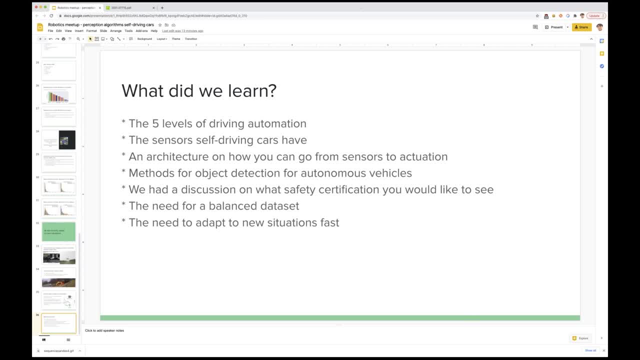 of time to first get the understanding of how, what, how, what, how, what and how the data set is being generated, and how the data set is being generated and how the data set is being generated, and a lot of time can go into. and a lot of time can go into. 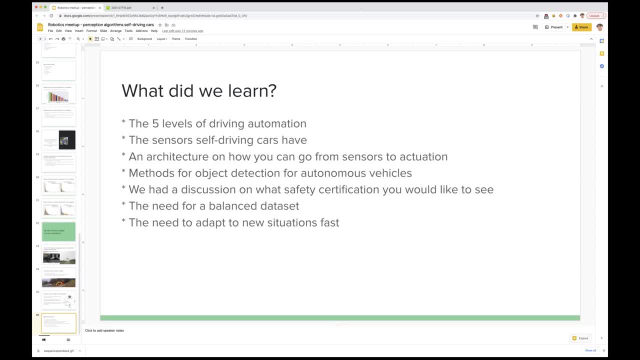 and a lot of time can go into understanding about the data set, in understanding about the data set, in understanding about the data set in itself, itself, itself, and also the next point would be how, and also the next point would be how, and also the next point would be: how better can we exploit that? 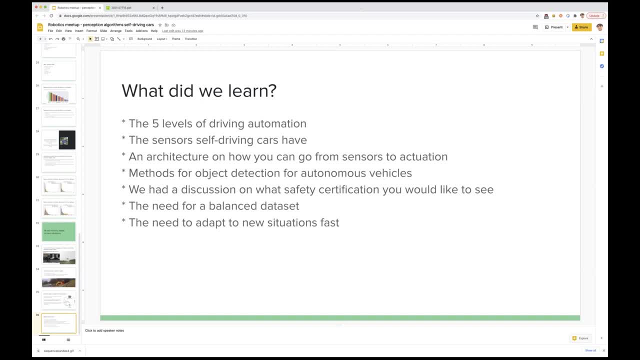 better. can we exploit that for uh any use case on a research friend, for uh any use case on a research friend, for uh any use case on a research friend or any other or any other or any other topic? so is there any development on topic? so is there any development on? 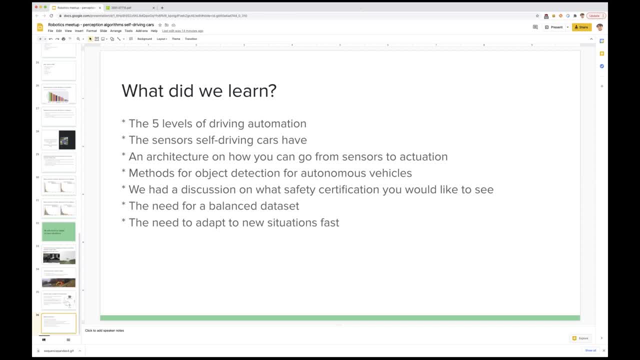 topic. so is there any development on that friend to standardize, or make it that friend to standardize, or make it that friend to standardize, or make it like a universal guideline, like a universal guideline, like a universal guideline? that on generating data sets which can, that on generating data sets which can. 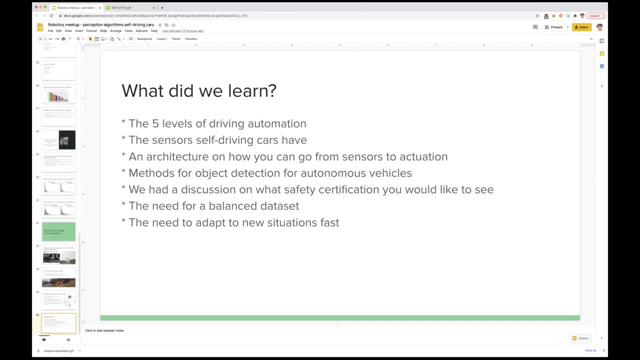 that on generating data sets which can make things simpler for use. make things simpler for use. make things simpler for use. people, i think there's one one standard. i people. i think there's one one standard. i people, i think there's one one standard. i don't know a lot about it, but there's. 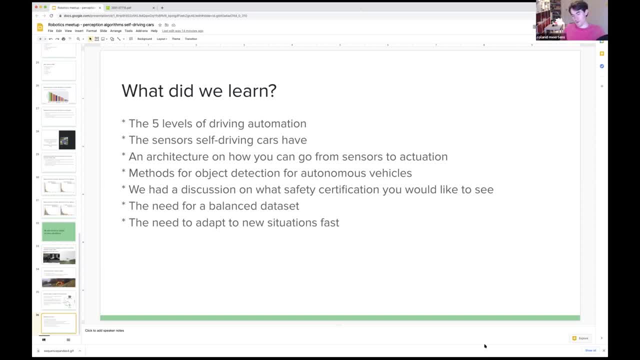 don't know a lot about it, but there's- don't know a lot about it, but there's at least the uh open label, uh label, at least the uh open label, uh label, at least the uh open label, uh label, standard, i think, which is trying to make. 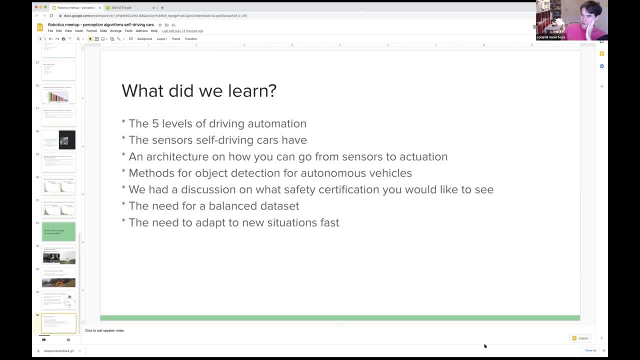 standard, i think which is trying to make standard, i think which is trying to make sure that at least people have the same sure, that at least people have the same sure, that at least people have the same kind of annotation schema formula style, kind of annotation schema formula style. 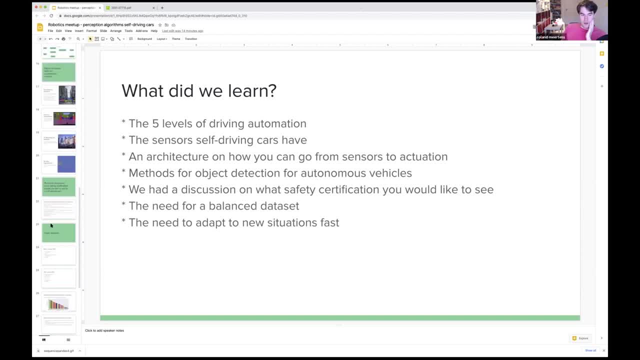 kind of annotation, schema, formula style. i think one inherent problem is that. i think one inherent problem is that. i think one inherent problem is that is the labels you choose are really. is the labels you choose are really? is the labels you choose are really important, right? so if you look at uh, 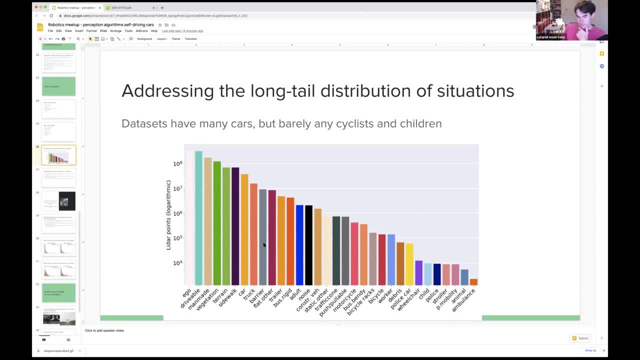 important, right. so if you look at uh- important, right. so if you look at uh here, the labels which nuisance uses here, the labels which nuisance uses here, the labels which nuisance uses: yeah, they. they have, for example, a: yeah, they, they have, for example, a: yeah, they. they have, for example, a difference between a car and a truck. 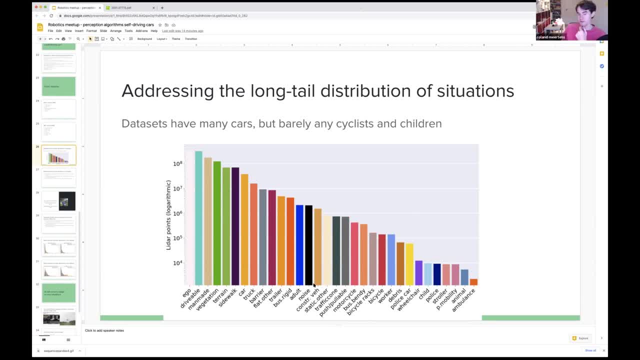 difference between a car and a truck, difference between a car and a truck and a trailer and a bus and a trailer and a bus, and a trailer and a bus and a construction vehicle and a construction vehicle and a construction vehicle. um, so, those are all and the police car. 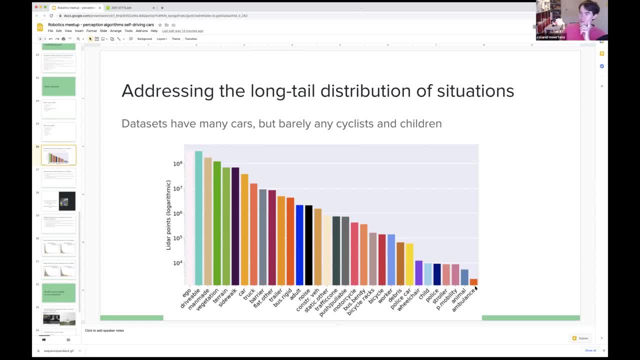 um. so those are all. and the police car, um, so those are all. and the police car and uh and the ambulance. so those are, and uh and the ambulance. so those are, and uh and the ambulance. so those are all different kind of vehicles, all different kind of vehicles. 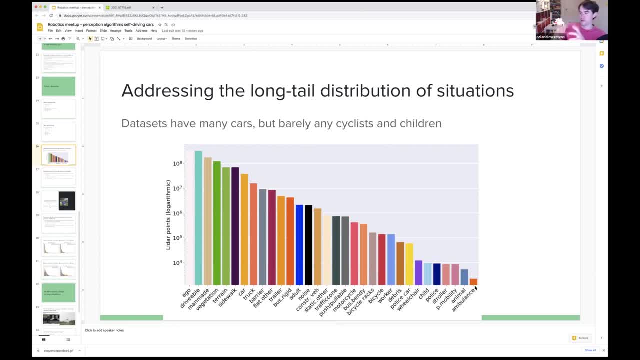 all different kind of vehicles. so one basically has to make a hierarchy. so one basically has to make a hierarchy. so one basically has to make a hierarchy of: okay, well, these are the high level of. okay, well, these are the high level of. okay, well, these are the high level classes. and then there's these: 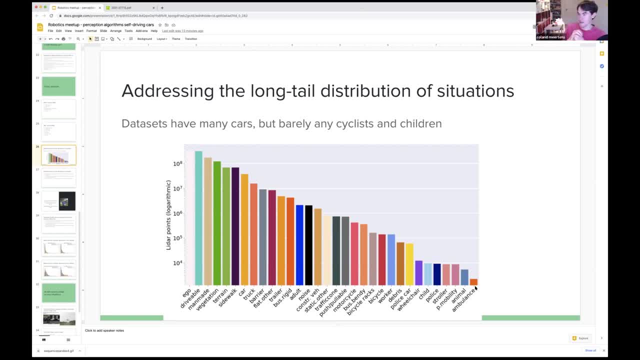 classes, and then there's these classes, and then there's these subclasses, subclasses, subclasses. so if someone proposes that everyone can, so if someone proposes that everyone can, so if someone proposes that everyone can go with it and can agree with it, go with it and can agree with it. 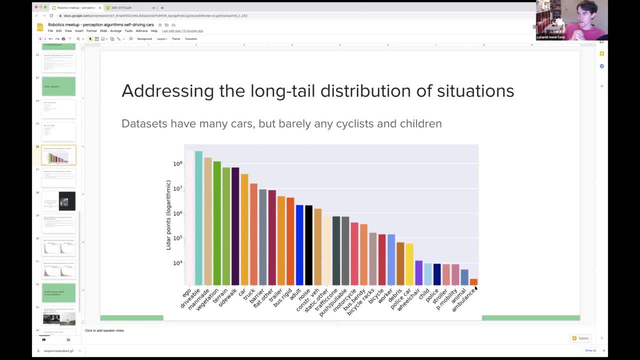 go with it and can agree with it, i think that's fine. but until then, i think that's fine, but until then i think that's fine, but until then, right now, basically, it's just right now. basically, it's just right now. basically it's just. every company has their own idea of what. 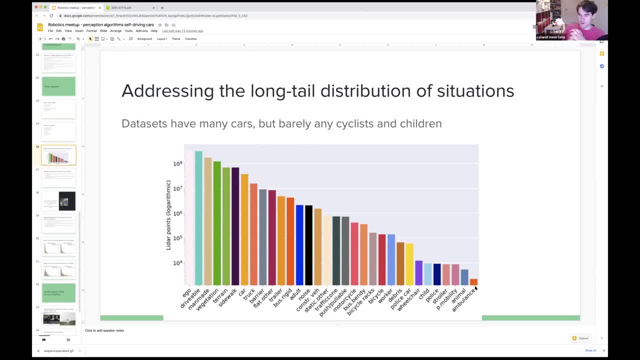 every company has their own idea of what. every company has their own idea of what they find important. they find important, they find important, and especially if you are thinking that, and especially if you are thinking that and especially if you are thinking that, for example, a robo. 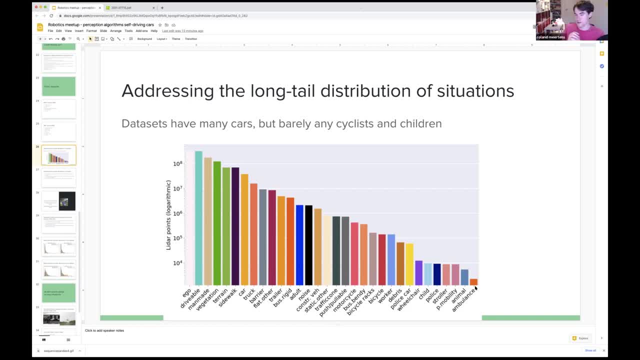 for example, a robo. for example, a robo, so why pay for annotating this? if so, why pay for annotating this? if so, why pay for annotating this? if you're needed or don't want it, you're needed or don't want it. you're needed or don't want it. um same, for i don't know, maybe. 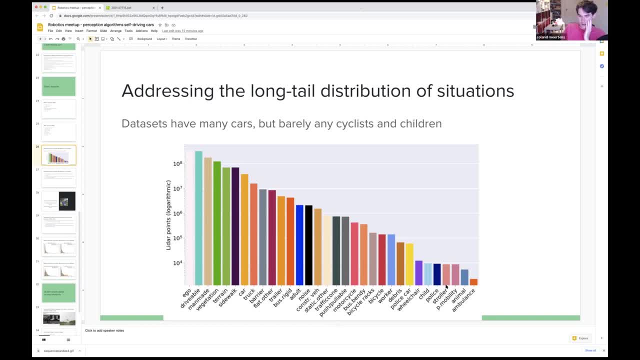 um same for i don't know. maybe um same for i don't know. maybe you want to know exactly whether it's a. you want to know exactly whether it's a. you want to know exactly whether it's a stroller or stroller or stroller or or something else. um, like you can make. 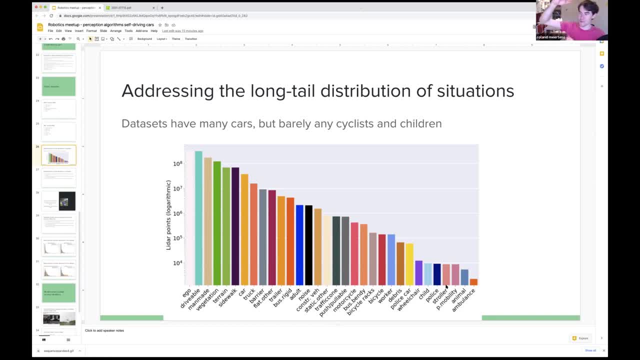 or something else, um like you can make, or something else, um like you can make this, this, this, you can make this labeling, you can make this labeling. you can make this labeling specification, specification, specification super long and have a thousand super long and have a thousand super long and have a thousand different edge cases for annotators. 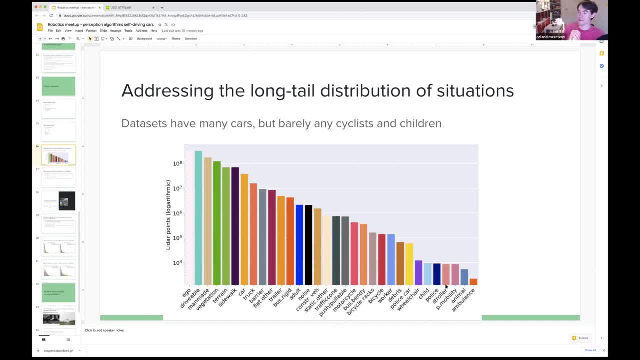 different edge cases for annotators. different edge cases for annotators: or you can make it really short and just, or you can make it really short and just, or you can make it really short and just say okay, say okay, say okay, annotate everything which is drivable. 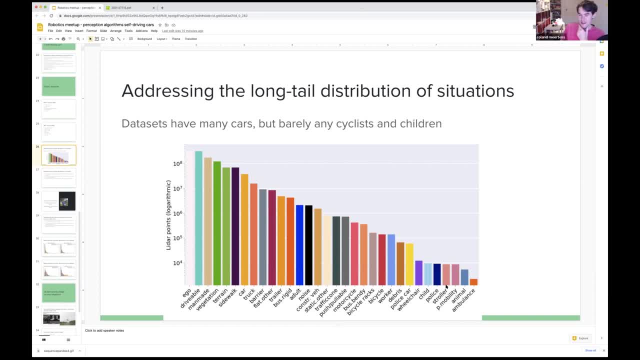 annotate everything which is drivable. annotate everything which is drivable or has a. has an engine as one one class, or has a. has an engine as one one class, or has a. has an engine as one one class. uh, so different data sets have different. uh, so different data sets have different. 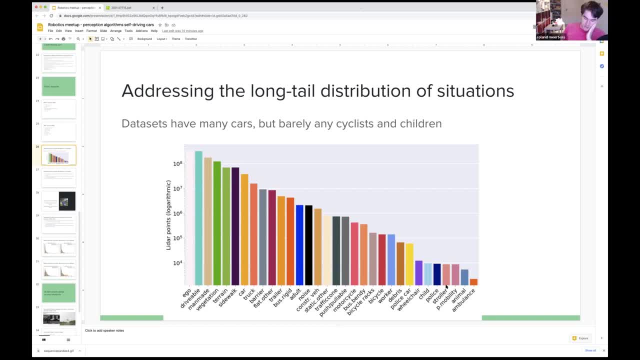 uh. so different data sets have different, different uh different things. i know that different uh different uh different things. i know that different uh different uh different things. i know that there's one for semantic, there's one for semantic, there's one for semantic segmentation. i think um. 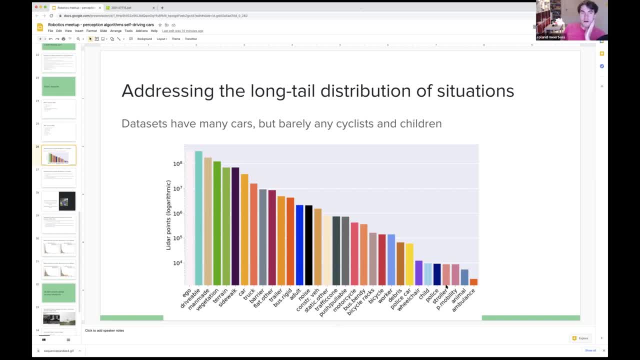 segmentation. i think um segmentation. i think um for iros last year, for iros last year, for iros last year: uh, some, there was a paper. i forgot the. uh. some there was a paper, i forgot the. uh. some there was a paper, i forgot the name. 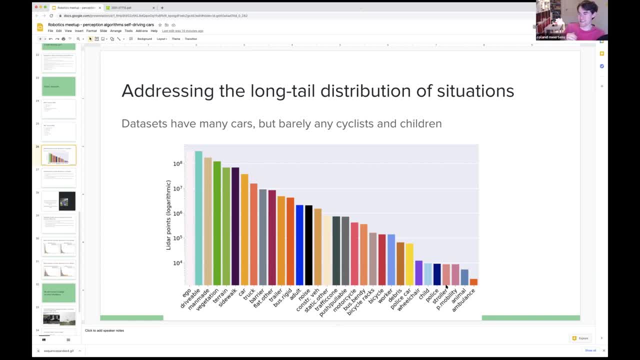 name, name, but they basically took loads of cemented. but they basically took loads of cemented, but they basically took loads of cemented. segmentation data sets. segmentation data sets. segmentation data sets: um, um, um. used a way to make a new, make new. used a way to make a new, make new. 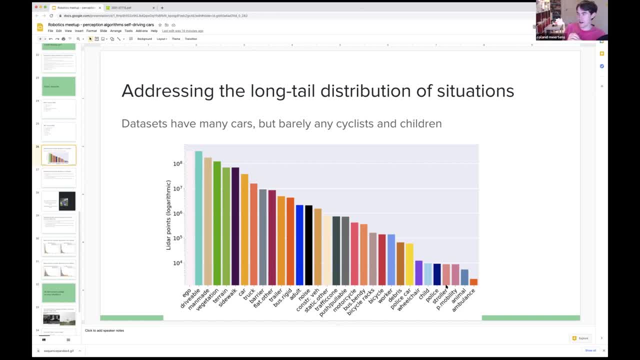 used a way to make a new, make new hierarchies across all these hierarchies, across all these hierarchies, across all these annotations, and then trained one big annotations and then trained one big annotations and then trained one big neural network on all these data sets at 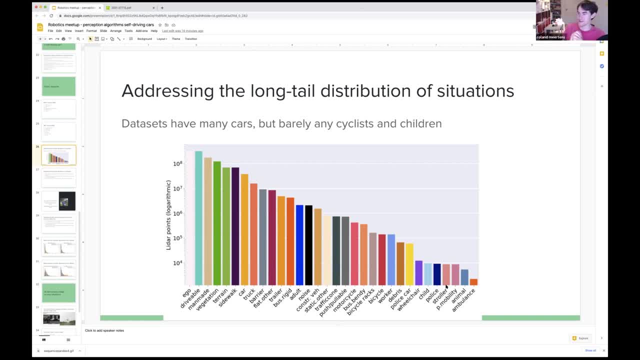 neural network, on all these data sets, at neural network, on all these data sets at the same time, the same time, and then you did super amazing results. and then you did super amazing results. and then you did super amazing results. where, where, where you could recognize indoor scenes, outdoor. 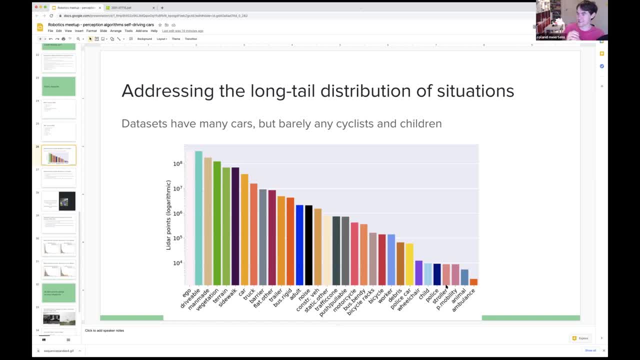 you could recognize indoor scenes, outdoor. you could recognize indoor scenes, outdoor scenes, all kind of scenes, all kind of scenes, all kind of all kinds of things. so if someone does that, all kinds of things, so if someone does that all kinds of things, so if someone does that for self-driving cars, that would be. 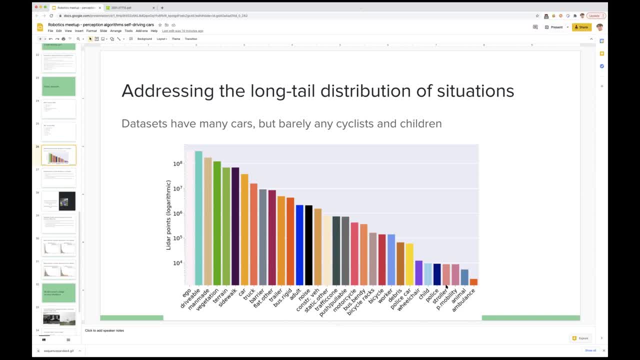 for self-driving cars. that would be for self-driving cars. that would be amazing, amazing, amazing. that's really cool uh, so that's really cool uh. so that's really cool, uh. so can you probably uh share a link, or if? can you probably uh share a link, or if? 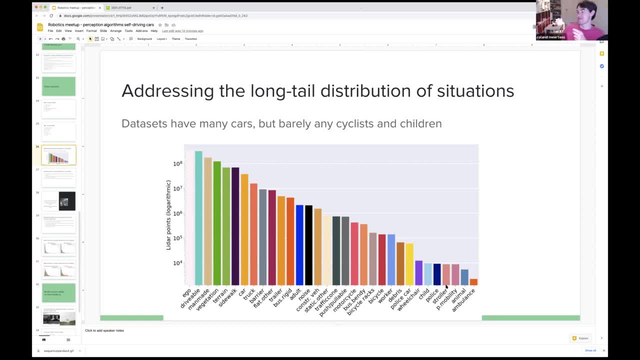 can you probably uh share a link or if there's a paper or something, if you there's a paper or something, if you there's a paper or something, if you remember later, maybe remember later, maybe remember later, maybe, if i find it, i will uh, i will uh. 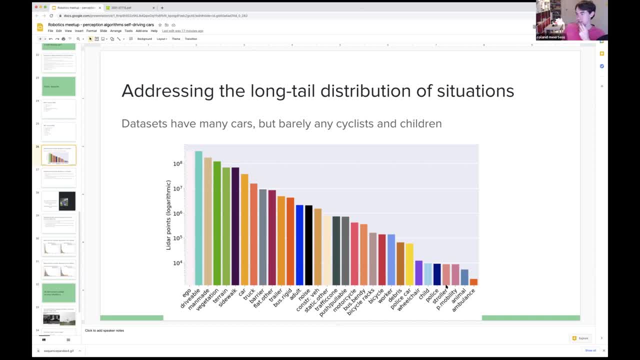 if i find it, i will uh, i will uh. if i find it, i will uh, i will uh send it um. but yeah, send me a message on send it um. but yeah, send me a message on send it um. but yeah, send me a message on linkedin. so i will try to. i will try to. linkedin, so i will try to. i will try to linkedin, so i will try to. i will try to search for it. search for it, search for it. it's a bit hard to search for it. because it's a bit hard to search for it because 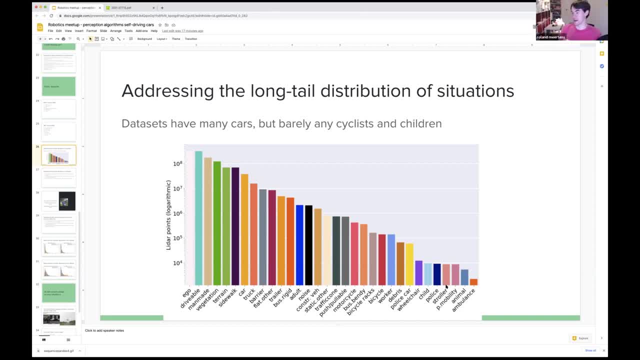 it's a bit hard to search for it, because the only thing i remember, if the only thing i remember, if the only thing i remember, if someone else in this chat, by the way, someone else in this chat, by the way, someone else in this chat, by the way, knows it, i mostly remember that they. 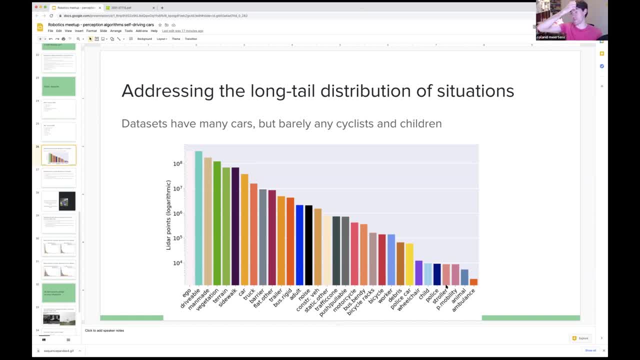 knows it. i mostly remember that they knows it. i mostly remember that they had a, had a, had a video of people making loads of backflips. video of people making loads of backflips, video of people making loads of backflips. and the neural network was recognizing. 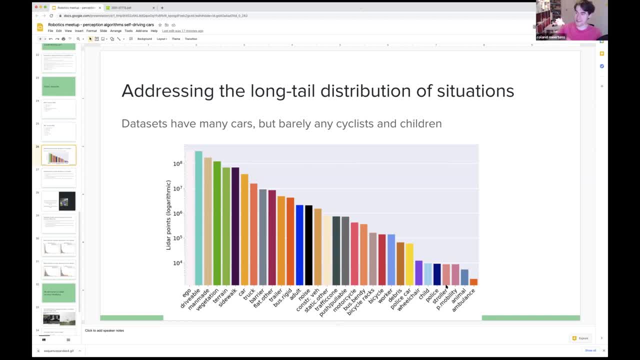 and the neural network was recognizing. and the neural network was recognizing that. if people now think, oh yeah, there's that. if people now think, oh yeah, there's that. if people now think, oh yeah, there's one paper where they had a video with one paper where they had a video with 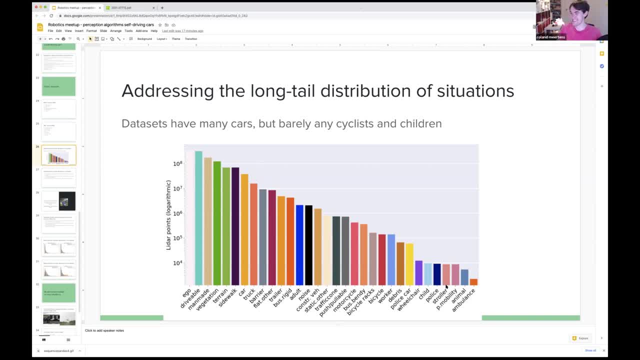 one paper where they had a video with loads of backflips, loads of backflips, loads of backflips. that's the one. okay, uh, send me a. that's the one. okay, uh, send me a. that's the one. okay, uh, send me a message on linkedin. i'll find it for. 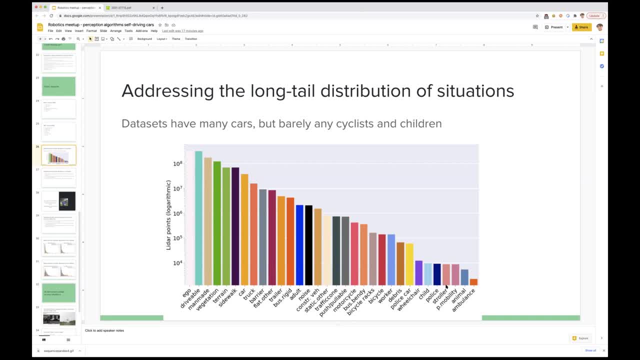 message on linkedin. i'll find it for you. sure, uh, one last question. i wouldn't you sure, uh, one last question. i wouldn't you sure, uh, one last question. i wouldn't wind it up with that. so wind it up with that. so wind it up with that. so, uh, everybody, or the industry, is now. 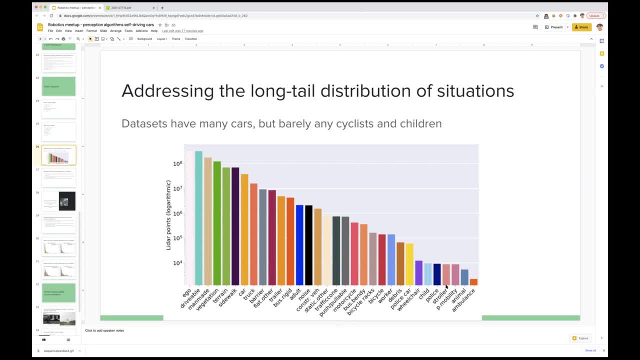 uh, everybody or the industry is now. uh, everybody or the industry is now driving towards um developing, driving towards um developing, driving towards um developing autonomous vehicles, but then on the autonomous vehicles, but then on the autonomous vehicles, but then on the other side, other side, other side, is there any foresight towards developing? 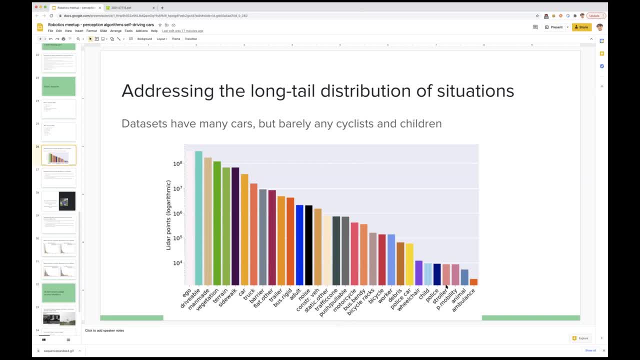 is there any foresight towards developing? is there any foresight towards developing the infrastructure that can make it more, the infrastructure that can make it more, the infrastructure that can make it more? realizable because realizable, because realizable, because- just the last point that we discussed um, 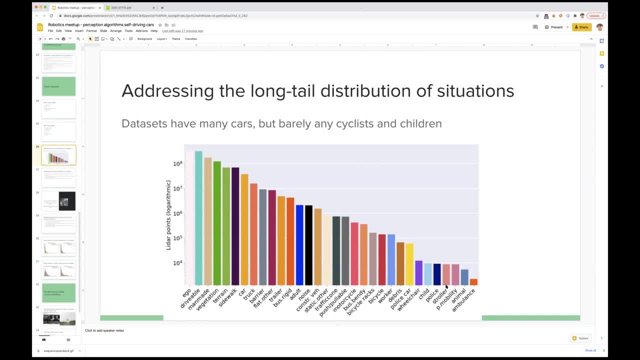 just the last point that we discussed, um. just the last point that we discussed, um. or the edge cases and other topics. or the edge cases and other topics. or the edge cases and other topics. uh, very simple example of uh the e. uh, very simple example of uh the e. 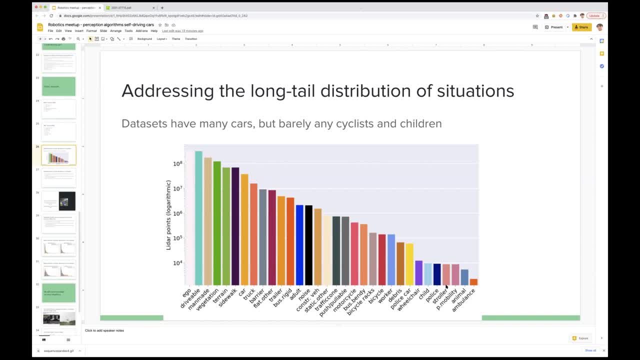 uh, very simple example of: uh, the e scooter that's been driving scooter that's been driving scooter that's been driving on the road or any other parking based on the road, or any other parking based on the road or any other parking based scenarios, scenarios, scenarios, but that can differ from country to. 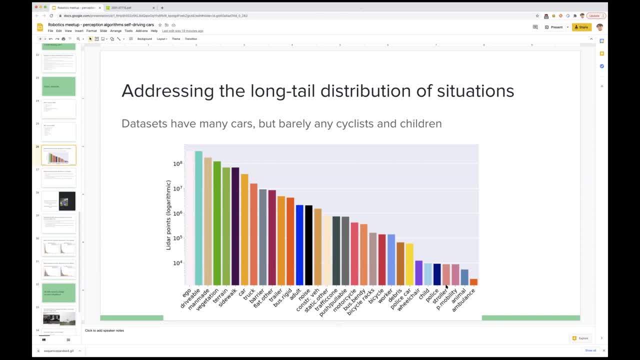 but that can differ from country to, but that can differ from country to country or country or country or globally so um, globally so, um, globally so, um, my question is like an open-ended like. my question is like an open-ended like. my question is like an open-ended like: is there a future towards developing the? 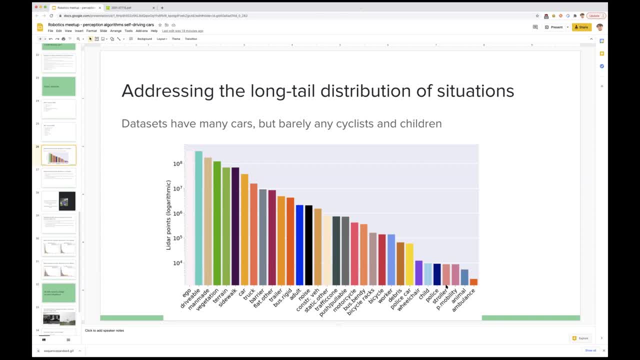 is there a future towards developing the? is there a future towards developing the infrastructure that can also go in, infrastructure that can also go in, infrastructure that can also go in uh speeding up the realization of, uh speeding up the realization of uh speeding up the realization of autonomous vehicle? 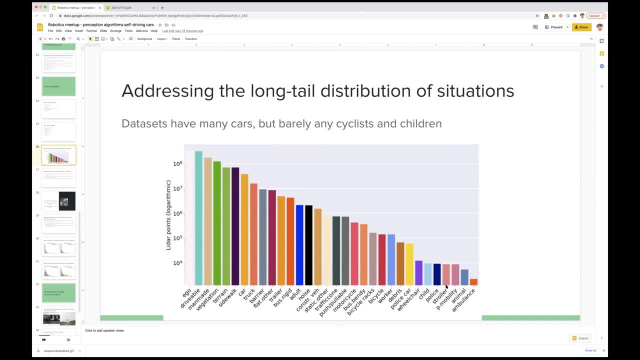 autonomous vehicle. autonomous vehicle. or would it be a demand on the? or would it be a demand on the? or would it be a demand on the development of autonomous vehicle being. development of autonomous vehicle being. development of autonomous vehicle being ready to adapt to any situations like: ready to adapt to any situations like. 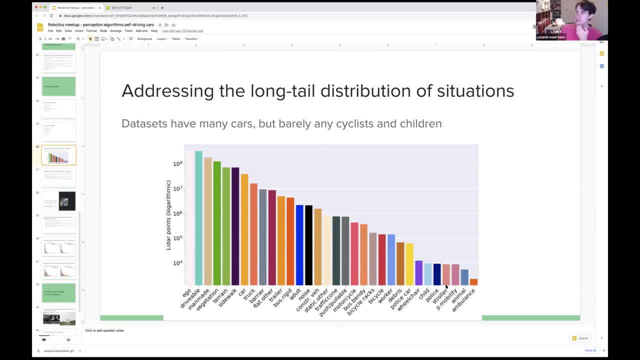 ready to adapt to any situations like which one is a proper trade-off? which one is a proper trade-off? which one is a proper trade-off? yeah, good question, so i actually won a. yeah, good question, so i actually won a. yeah, good question, so i actually won a hackathon in 2017. 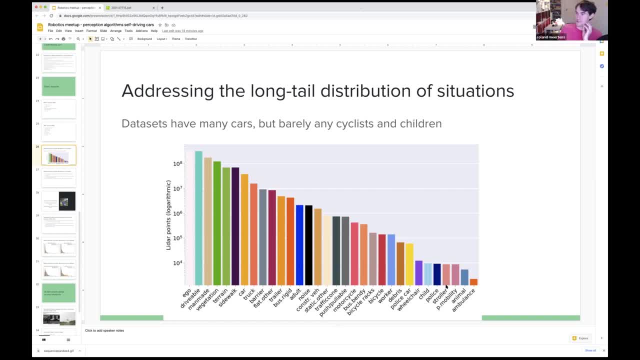 hackathon in 2017. hackathon in 2017: uh for coming up with proposals for the uh. for coming up with proposals for the uh. for coming up with proposals for the. for local government to improve their. for local government to improve their. for local government to improve their infrastructure for self-driving cars. 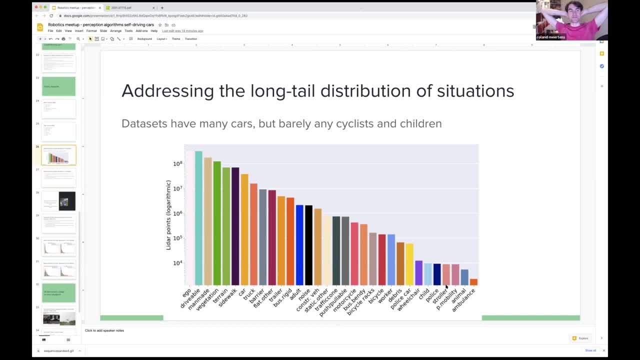 infrastructure for self-driving cars. infrastructure for self-driving cars- so that was cool, um, but so so you can. so that was cool, um, but so so you can. so that was cool, um, but so so you can see that. see that. see that, even like smaller, smaller governments are. 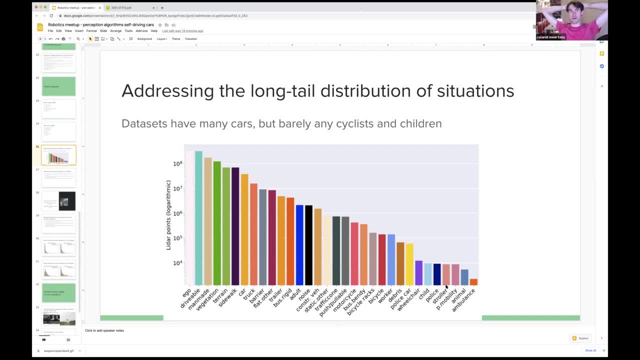 even like smaller, smaller governments are, even like smaller, smaller governments are thinking about: okay, what's what do we thinking about? okay, what's what do we thinking about? okay, what's what do we want to want to want to do? and in the netherlands, for example, do. and in the netherlands, for example, 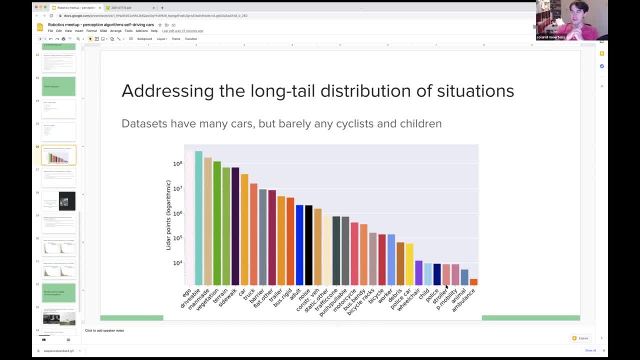 do, and in the netherlands, for example, there's already loads of yeah, they call there's already loads of yeah, they call. there's already loads of yeah, they call it's uh intelligence, uh for kids. it's uh intelligence, uh for kids. it's uh intelligence, uh for kids. intelligent intersections. 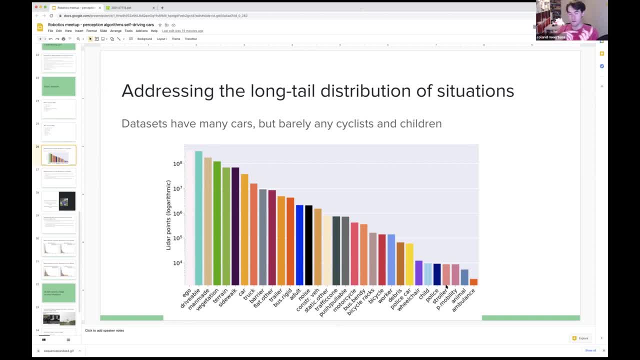 intelligent intersections. intelligent intersections where they are, where they are, where they are, like over the internet. you can already get like over the internet. you can already get like over the internet. you can already get the traffic light information, the traffic light information, the traffic light information, so you know if your self-driving car can. 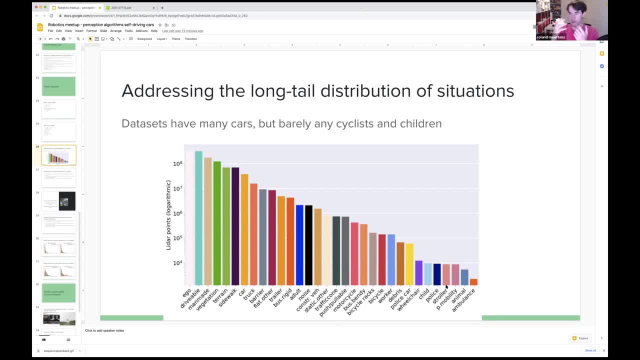 so you know if your self-driving car can. so you know if your self-driving car can drive or not drive or not drive or not. so other countries are maybe lagging a, so other countries are maybe lagging a. so other countries are maybe lagging a bit behind that. 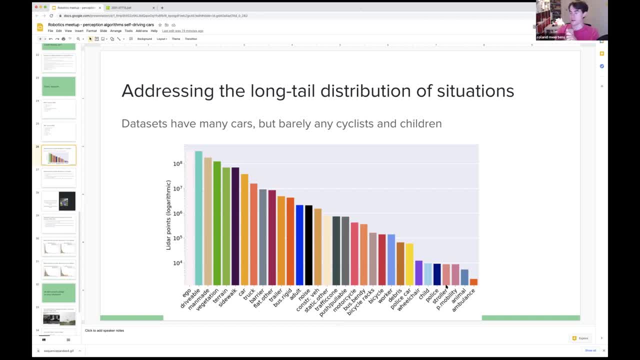 bit behind that, bit behind that. if you look at, for example, pony ai, who is. if you look at, for example, pony ai who is. if you look at, for example, pony ai who is operating in china- they just made a deal- operating in china. they just made a deal. 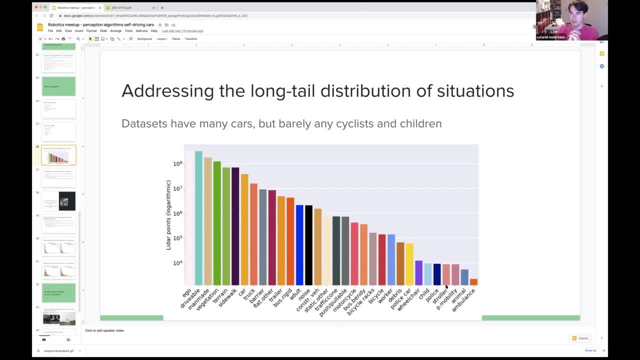 operating in china. they just made a deal with the local chinese government, with the local chinese government, with the local chinese government. i think that the government in china is, i think that the government in china is. i think that the government in china is way more lenient towards. oh well, let's. 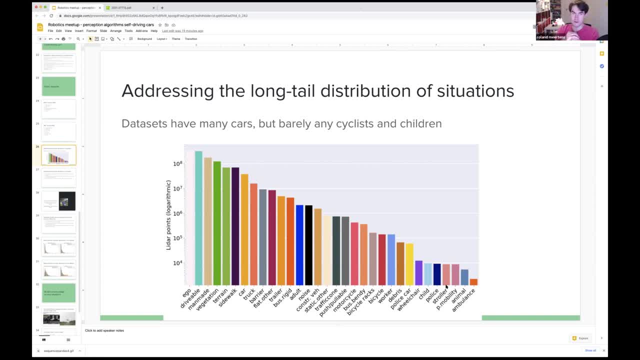 way more lenient towards- oh well, let's way more lenient towards- oh well, let's just do this, just do this, just do this, because it gives us a lot of economic, because it gives us a lot of economic, because it gives us a lot of economic benefits. 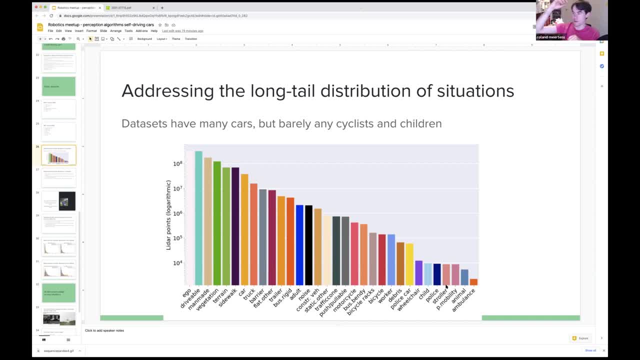 benefits, benefits: um to us uh putting lidars, for example, um to us uh putting lidars, for example, um to us uh putting lidars, for example, on intersections, on intersections, on intersections, so that in really difficult traffic, so that in really difficult traffic, so that in really difficult traffic situations you can just rely on. 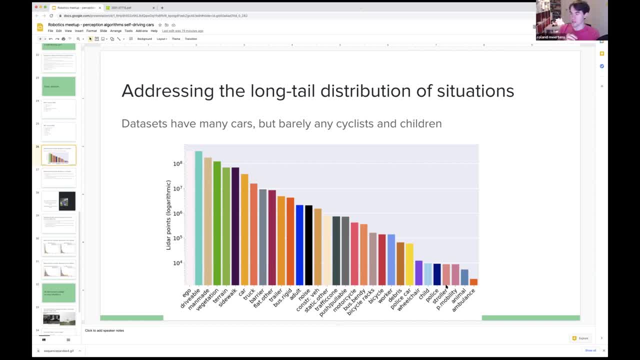 situations. you can just rely on situations. you can just rely on intersection to give you intersection to give you intersection to give you information yourself. driving car needs information yourself. driving car needs information yourself. driving car needs so you need, so you need, so you need to have a less impressive perception stack. 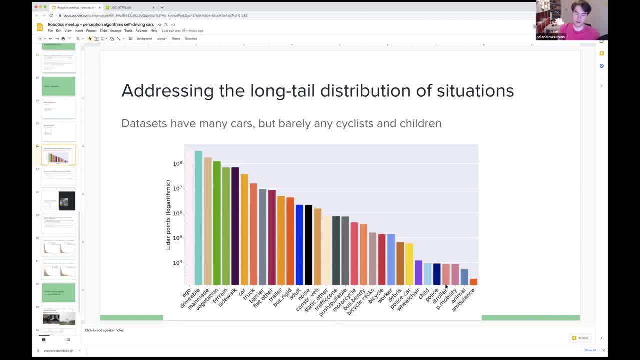 to have a less impressive perception stack. to have a less impressive perception stack, you basically have an extra center, or an. you basically have an extra center, or an. you basically have an extra center or an extra, extra, extra. source of information- um for where. source of information: um for where. 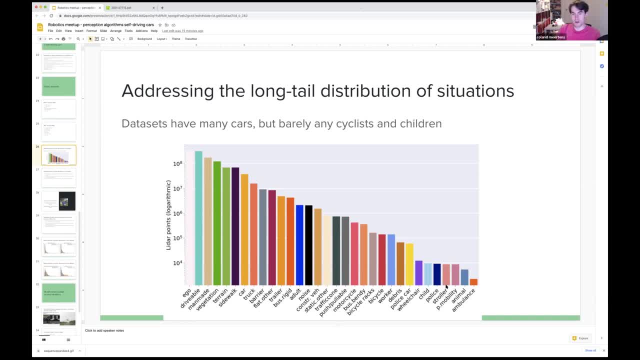 source of information, um, for where objects are and where they're going and objects are and where they're going, and objects are and where they're going, and what's what they are allowed to do. what's what they are allowed to do? what's what they are allowed to do? uh, i think one big problem is that, uh, 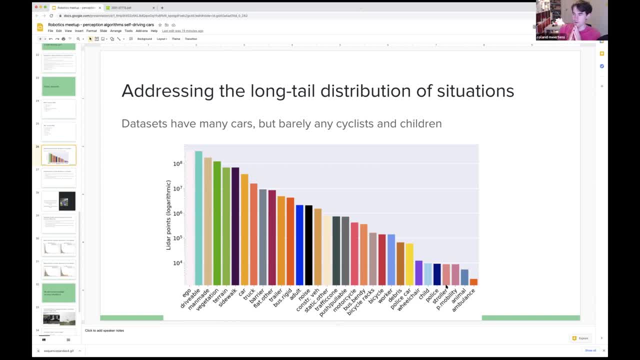 uh, i think one big problem is that, uh, uh, i think one big problem is that, uh, in other countries, maybe you're not in other countries, maybe you're not in other countries, maybe you're not willing to wait that long, uh, or wait. or willing to wait that long, uh, or wait, or. 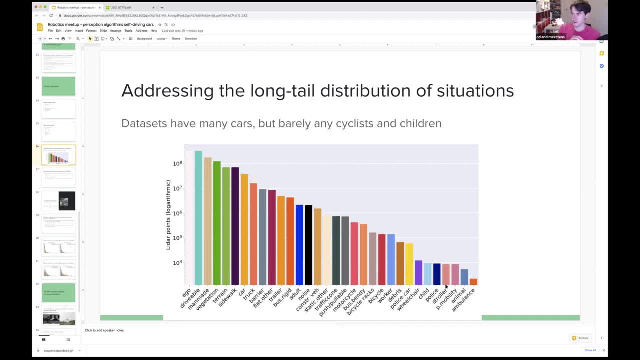 willing to wait that long. uh, or wait, or yeah, be dependent on the government. to yeah, be dependent on the government. to yeah, be dependent on the government to change your infrastructure, change your infrastructure, change your infrastructure. so i think that, loads of self-driving. so i think that loads of self-driving. 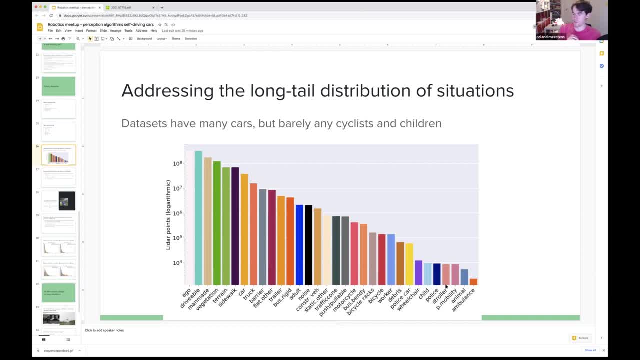 so i think that loads of self-driving car companies still want to solve the car companies still want to solve the car companies still want to solve the problem without a need problem, without a need problem, without a need to adapt infrastructure. uh, simply because to adapt infrastructure? uh, simply because. 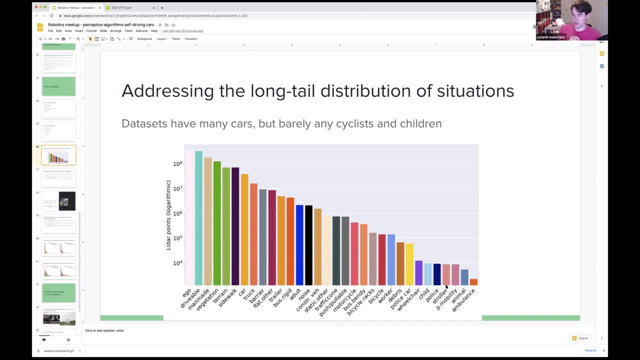 to adapt infrastructure? uh, simply because you have to solve this problem anyways, you have to solve this problem anyways. you have to solve this problem anyways, if you want to expand globally, if you want to expand globally, if you want to expand globally. uh, see you afterwards. uh, thanks for. 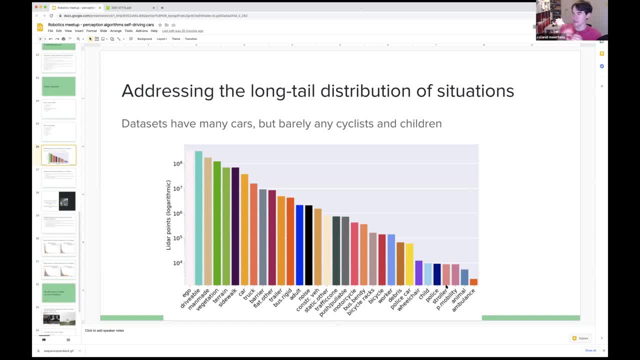 uh see you afterwards. uh, thanks for uh see you afterwards. uh, thanks for being here, being here, being here, um, so yeah, if you have to solve the um, so yeah. if you have to solve the um, so yeah. if you have to solve the problem, anyways you have to solve it. 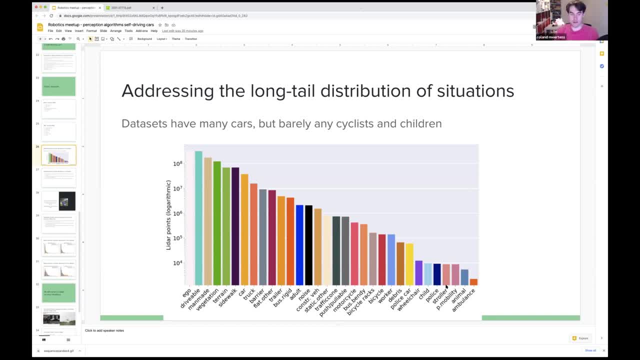 problem anyways, you have to solve it. problem anyways, you have to solve it anyways, um, anyways, um, anyways, um. so yeah, it is definitely infrastructure. so yeah, it is definitely infrastructure. so yeah, it is definitely infrastructure, is definitely a point, is definitely a point, is definitely a point, but um, yeah, yeah. 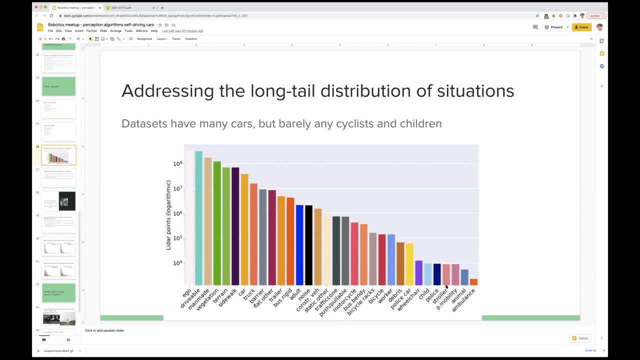 but um, yeah, yeah, but um, yeah, yeah, okay, i mean it makes sense like not okay. i mean it makes sense like not okay. i mean it makes sense like not every government across every government, across every government, across different countries, would be ready and different countries would be ready, and 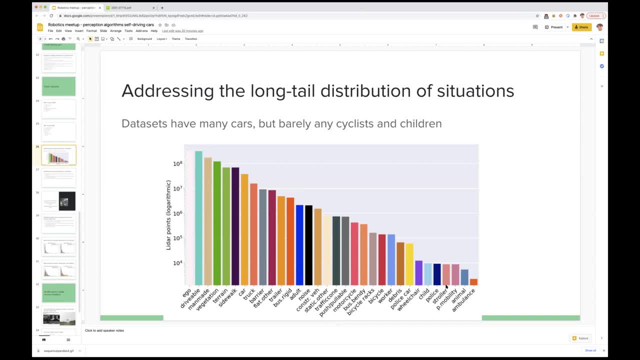 different countries would be ready and would have the? uh. would have the uh. would have the uh. the technology at hand to do that, uh. so the technology at hand to do that uh. so the technology at hand to do that uh. so okay, and pretty much, that's it, thank you. 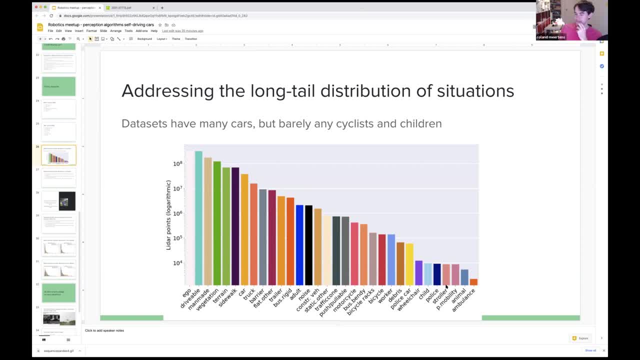 okay, and pretty much that's it. thank you. okay and pretty much that's it. thank you very much for your answers. very much for your answers. very much for your answers. no problem, i actually have some questions um, do you? i actually have some questions um, do you? 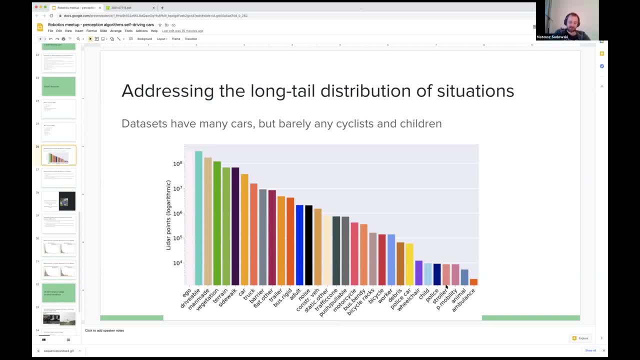 i actually have some questions. um, do you have you seen? have you seen? have you seen many people using event cameras, many people using event cameras, many people using event cameras- oh yeah, event cameras are really. oh yeah, event cameras are really. oh yeah, event cameras are really show. is uh posting them always on his 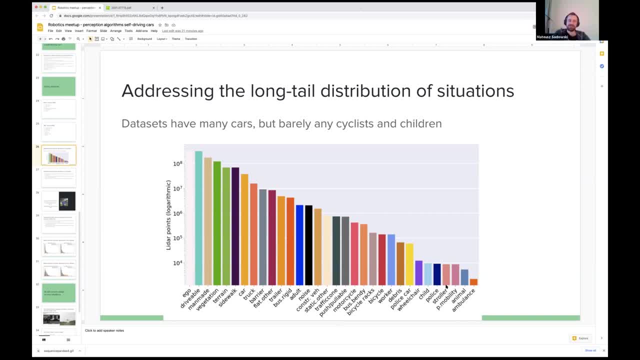 show. is uh posting them always on his show? is uh posting them always on his linkedin right, linkedin right, linkedin right? yeah, yeah, so i always see his videos. yeah, yeah, so i always see his videos. yeah, yeah, so i always see his videos. yeah, yeah, yeah, so i always see his videos, yeah. 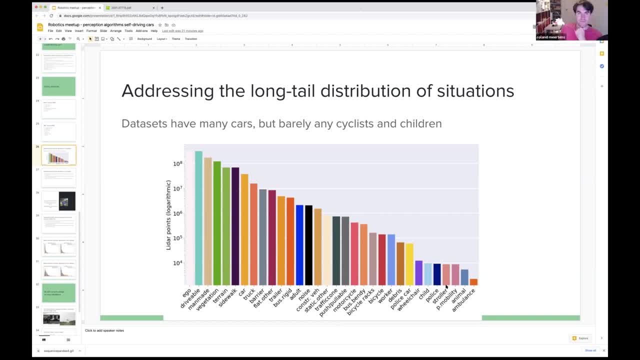 yeah, yeah, so i always see his videos. yeah, but yeah, i don't know if any. but yeah, i don't know if any, but yeah, i don't know if any. um serious, um serious, um serious. self-driving car company has them on. self-driving car company has them on. 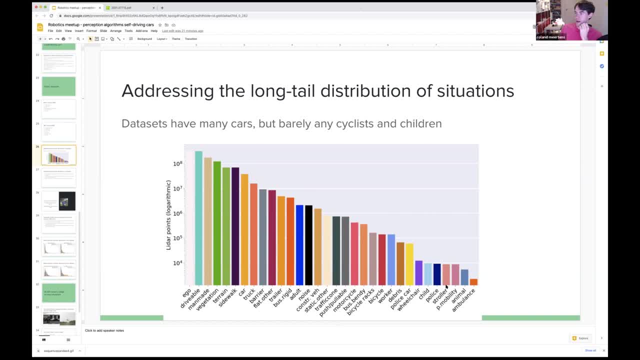 self-driving car company has them on their, their, their uh on their vehicle already. i haven't uh on their vehicle already. i haven't uh on their vehicle already. i haven't seen any specific open cell driving car, seen any specific open cell driving car. seen any specific open cell driving car? data sets with, eventually, event cameras. 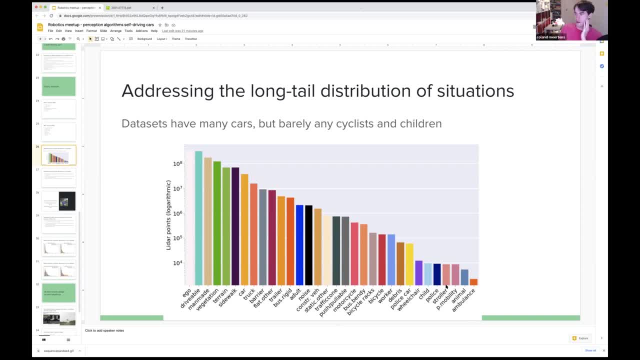 data sets with, eventually, event cameras. data sets with eventually event cameras: like yeah, they look really interesting. like, yeah, they look really interesting. like. yeah, they look really interesting, especially in combination with like. especially in combination with like, especially in combination with like. spiking neural networks: uh, spiking neural networks uh. 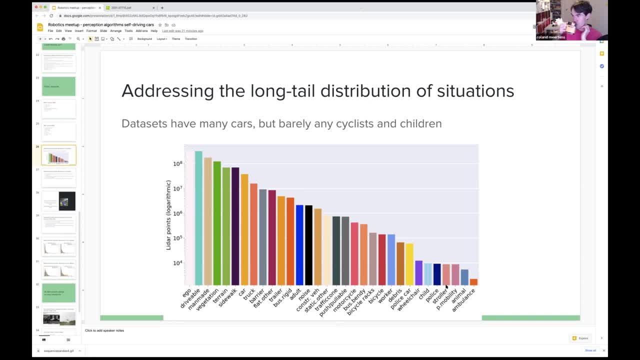 spiking neural networks. uh, it could be a, it could be a big thing. um, it could be a, it could be a big thing. um, it could be a, it could be a big thing. um, yeah, yeah, yeah, yeah, yeah, yeah, i'm wondering how they would come rain. 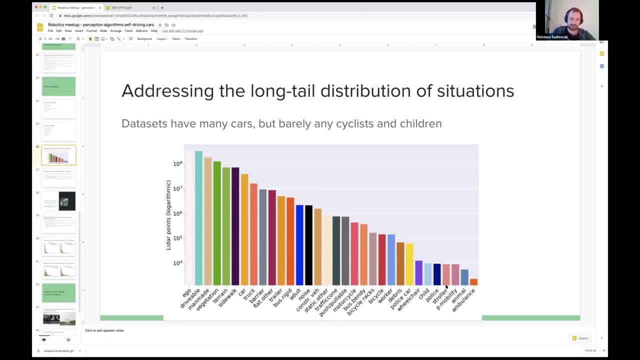 i'm wondering how they would come rain. i'm wondering how they would come rain, but uh, i'll try to get someone uh, but uh, i'll try to get someone uh, but uh, i'll try to get someone uh, working with event cameras to do a. working with event cameras to do a. 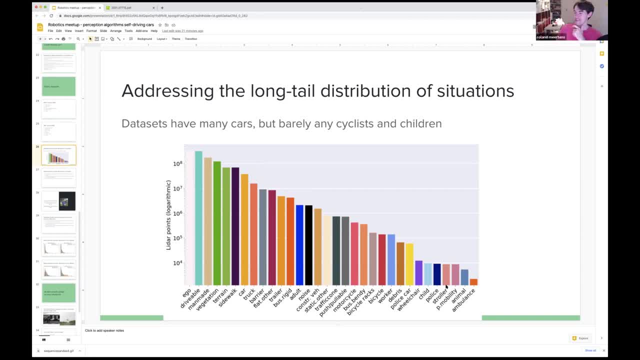 working with event cameras to do a meetup. i think it would be super meetup. i think it would be super meetup. i think it would be super interesting, interesting, interesting, i, i would love to uh to play around with. i, i would love to uh to play around with. 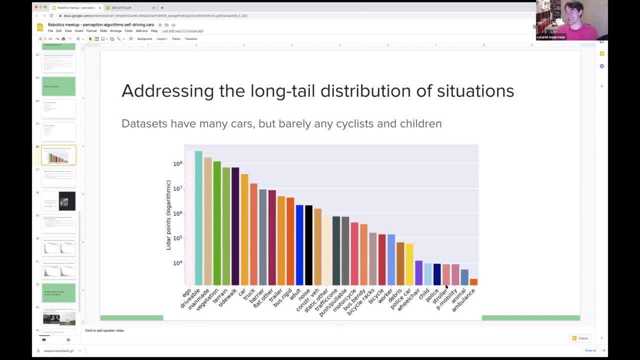 i, i would love to uh, to play around with it for a for a couple of weeks. yeah so if it for a for a couple of weeks, yeah so if it for a for a couple of weeks, yeah. so if someone has like a spare one, someone has like a spare one. 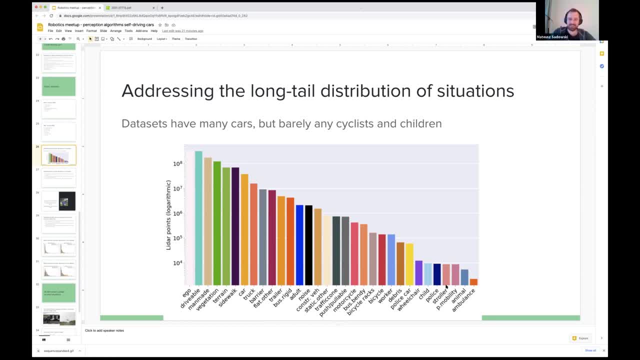 someone has like a spare one, let me know, let me know. let me know. i think they cost at least three k's at. i think they cost at least three k's at. i think they cost at least three k's at least, least, least when i looked into them about two years. 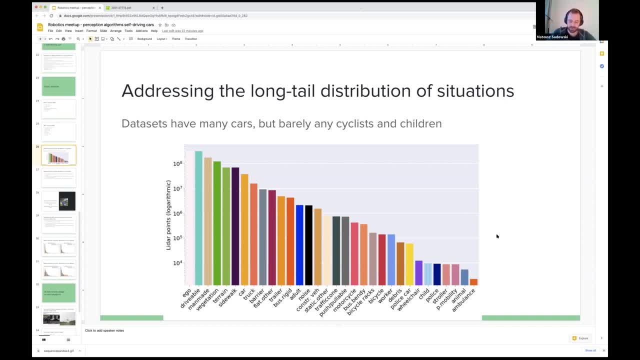 when i looked into them about two years, when i looked into them about two years ago ago ago, um, so not not terrible compared to um. so not not terrible compared to um. so not not terrible compared to liners, liners, liners, yeah, yeah, another. another question i have is: uh, 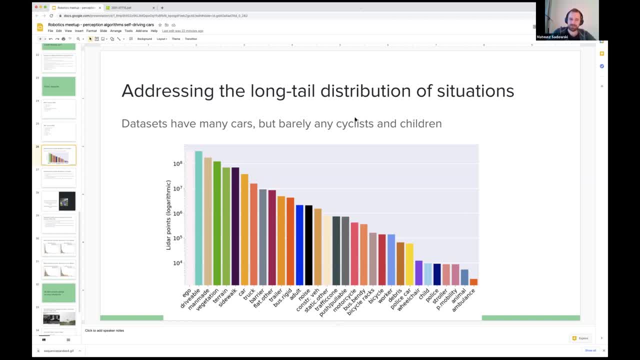 another question i have is uh. another question i have is: uh, do you happen to know? do you happen to know, do you happen to know? michael the court, michael the court, michael the court, yeah, yeah, yeah, um, and i think he's pushing a. um, and i think he's pushing a. 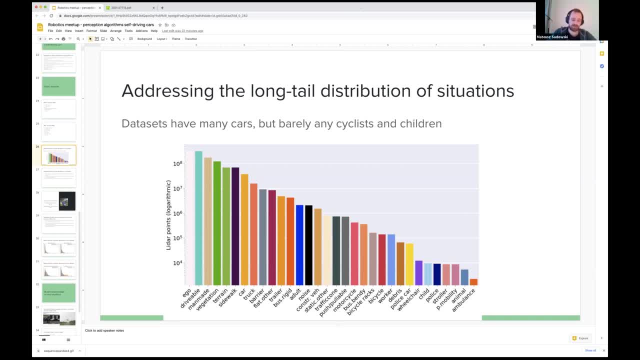 um, and i think he's pushing a simulator, uh, simulator, uh, simulator, uh. so he's developing a simulator and he's so he's developing a simulator and he's so he's developing a simulator, and he's arguing that, arguing that, arguing that most of the self-drivings 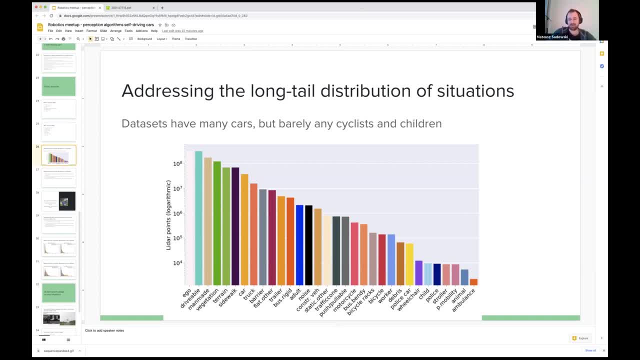 most of the self-drivings, most of the self-drivings. uh stacks are done uh in the wrong. uh stacks are done uh in the wrong. uh stacks are done uh in the wrong way. way, way, yeah, yeah, yeah, because you run everything in a single. 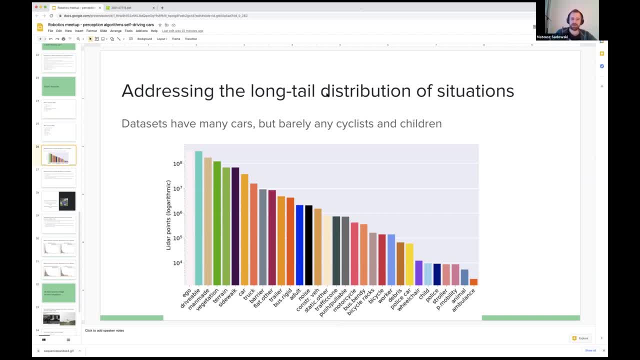 because you run everything in a single, because you run everything in a single process, and instead process and instead process, and instead everything should be decoupled, so every everything should be decoupled, so every everything should be decoupled. so every process should be decoupled, and then 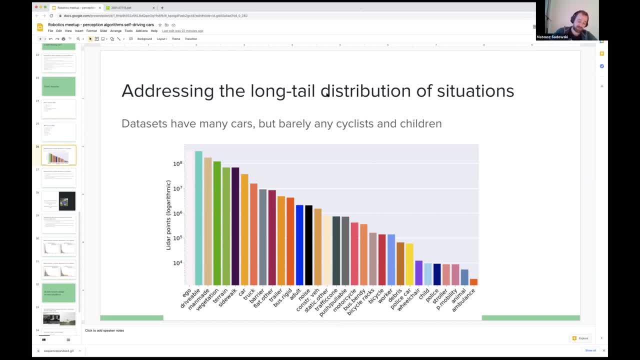 process should be decoupled, and then process should be decoupled, and then your simulation should work in your simulation should work in your simulation should work in such a way, such a way, such a way. but i don't think i fully grasp it, so i'm 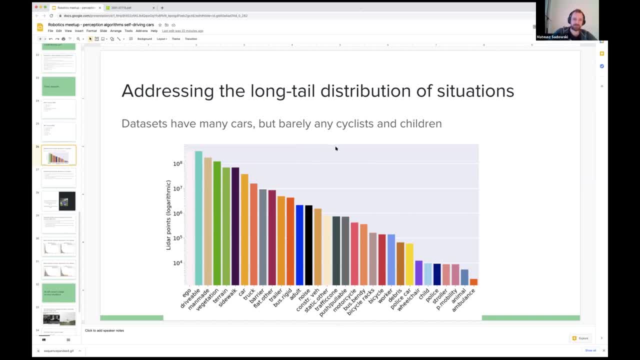 but i don't think i fully grasp it. so i'm, but i don't think i fully grasp it. so i'm wondering: what do you think about this? wondering what do you think about this? wondering: what do you think about this? if you know, if you know? 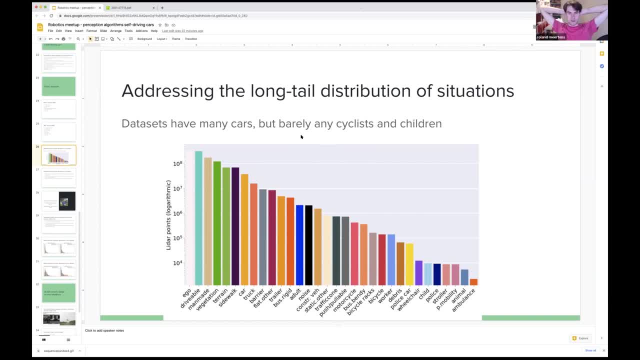 if you know what this is about. yeah well, so the first what this is about: yeah well, so the first what this is about: yeah, well. so the first thing is, maybe that michael is thing is maybe that michael is thing is maybe that michael is always a person who, on linkedin, is really 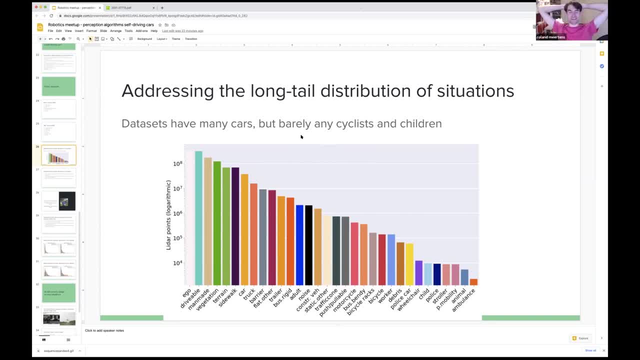 always a person who on linkedin is really always a person who on linkedin is really pessimistic, pessimistic, pessimistic about. he is always writing medium articles about. he is always writing medium articles about. he is always writing medium articles about everything self-driving car- about everything self-driving car. 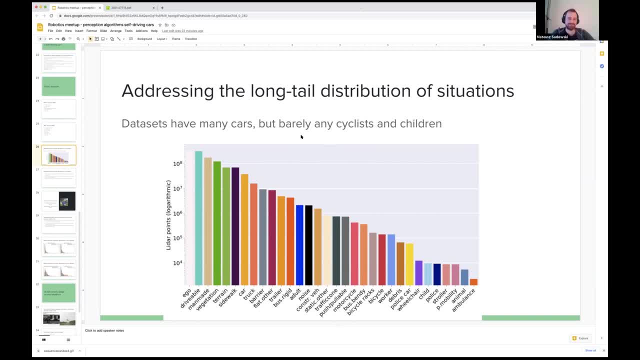 about everything self-driving car companies are doing is wrong companies are doing is wrong. companies are doing is wrong, which i think is an interesting premise, which i think is an interesting premise, right in that sense, that right in that sense, that right in that sense that there needs to be a really thorough. 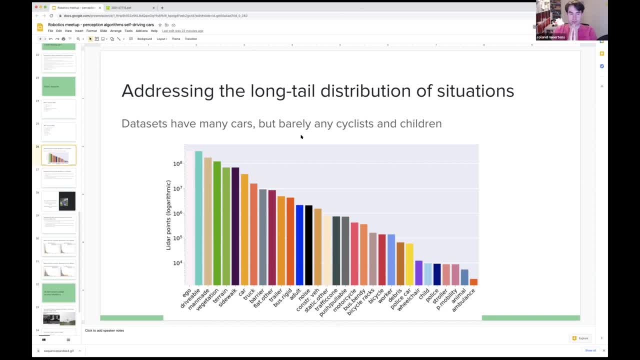 there needs to be a really thorough. there needs to be a really thorough validation, validation, validation which is something which is harder to, which is something which is harder to, which is something which is harder to find, or which self-driving cars find, or which self-driving cars find, or which self-driving cars car companies are less open about. so 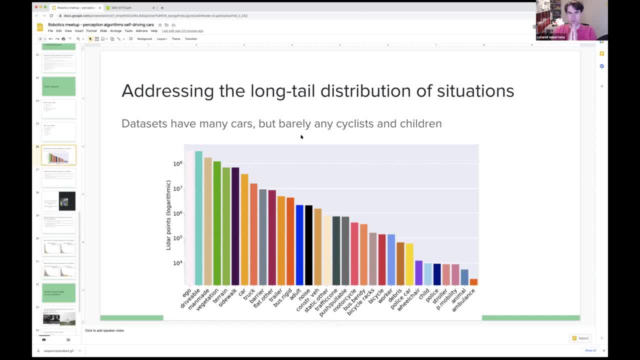 car companies are less open about so. car companies are less open about so. even if you look at the safety reports, even if you look at the safety reports, even if you look at the safety reports, kind of every self-driving company has a, kind of every self-driving company has a. 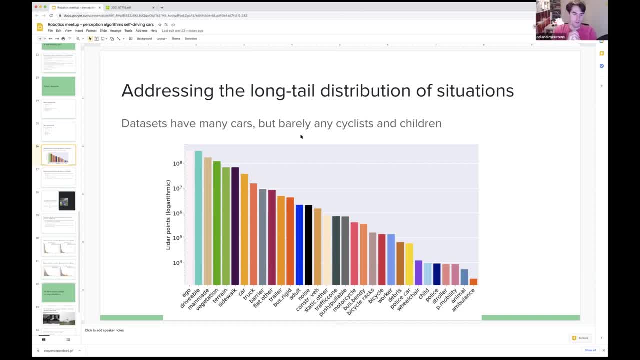 kind of every self-driving company has a safety report now of like 100 pages, safety report now of like 100 pages, safety report now of like 100 pages. and i think one justified critique of, and i think one justified critique of, and i think one justified critique of michael is that 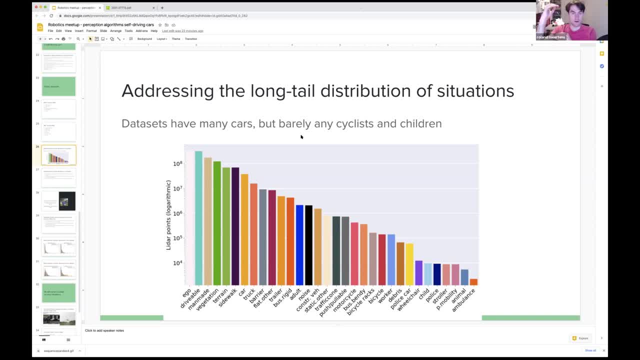 michael is that? michael is that the safety report is both something to the safety report, is both something to the safety report, is both something to sell your company. sell your company, sell your company as well as put your safety case in, and as well as put your safety case in and. 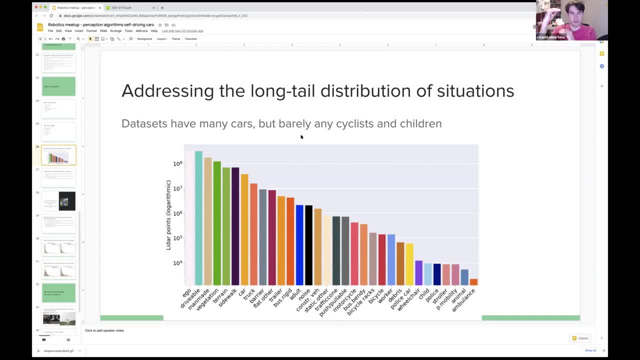 as well as put your safety case in, and there's a lot of selling in those. there's a lot of selling in those. there's a lot of selling in those reports and reports and reports and maybe not enough safety case. so maybe not enough safety case so. 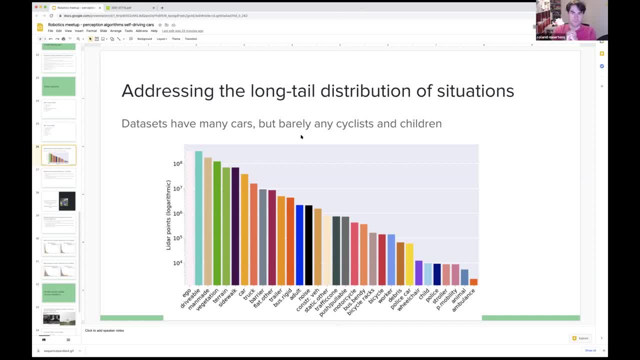 maybe not enough safety case. so something which you can't find, something which you can't find, something which you can't find is, um, what is the effective range of is? um? what is the effective range of is um? what is the effective range of your lidar? what kind of uh? 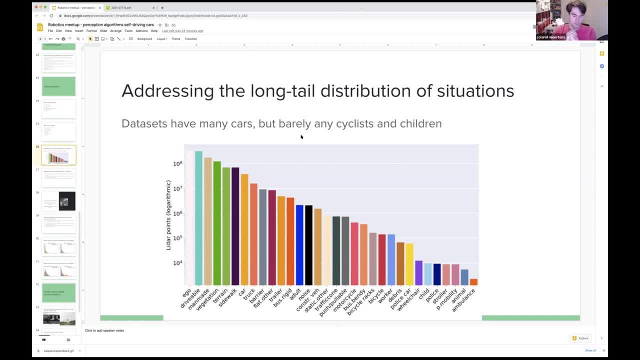 your lidar? what kind of uh your lidar? what kind of uh? what kind of objects do you have a problem? what kind of objects do you have a problem? what kind of objects do you have a problem with um, with um, with um, or what is the effective uh, like what? 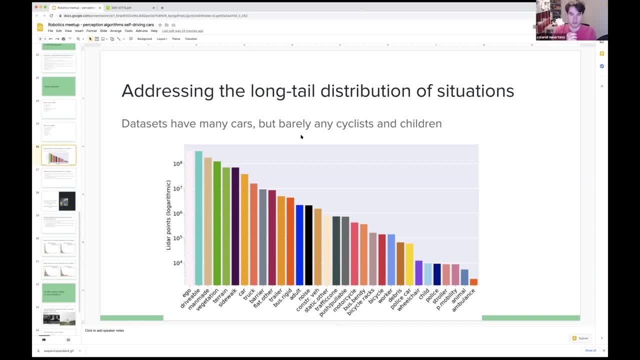 or what is the effective? uh, like what? or what is the effective? uh, like, what are your specific neural network metrics? are your specific neural network metrics? are your specific neural network metrics? you know what's your confusion matrix? uh, you know what's your confusion matrix? uh, you know what's your confusion matrix. uh, what objects do you have a problem with? 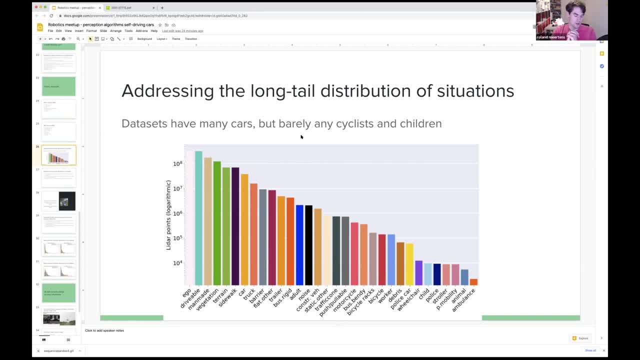 what objects do you have a problem with? what objects do you have a problem with um? what kind of objects can you not um? what kind of objects can you not um? what kind of objects can you not handle? uh, handle, uh, handle, uh. so yeah, in that sense, i totally see what. 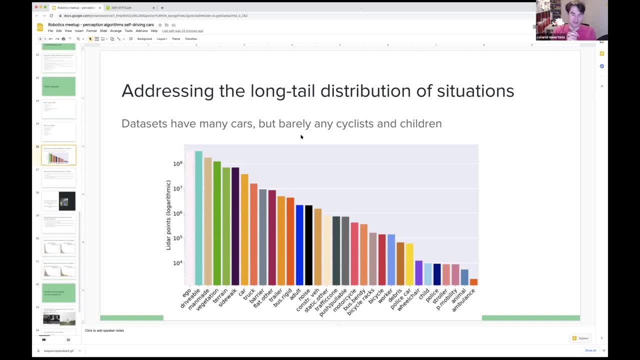 so yeah, in that sense i totally see what. so, yeah, in that sense i totally see what. michael is saying that there. michael is saying that there. michael is saying that there are there might be a need for like a. are there might be a need for like a. 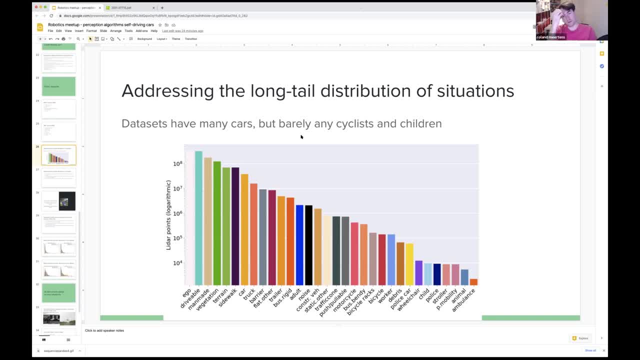 are. there might be a need for, like, a different way of validating things, um different way of validating things, um different way of validating things. um, i don't know exactly what the thing he's. i don't know exactly what the thing he's. i don't know exactly what the thing he's doing with the simulation. i haven't. 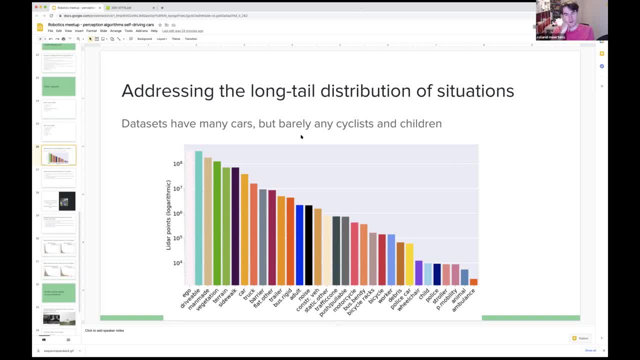 doing with the simulation. i haven't doing with the simulation. i haven't really read into that. so i should maybe really read into that, so i should maybe really read into that. so i should maybe do that, do that, do that, um, but i think he's more for doing. 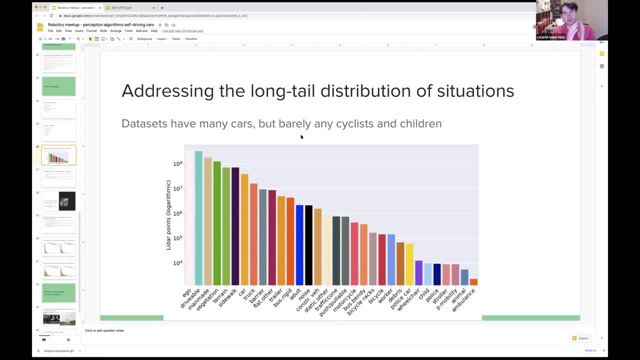 um, but i think he's more for doing um, but i think he's more for doing things, the traditional automotive way things. the traditional automotive way things. the traditional automotive way where you just say, okay, well, these, these. where you just say, okay, well, these, these. where you just say, okay, well, these. these are the specific aspects of my 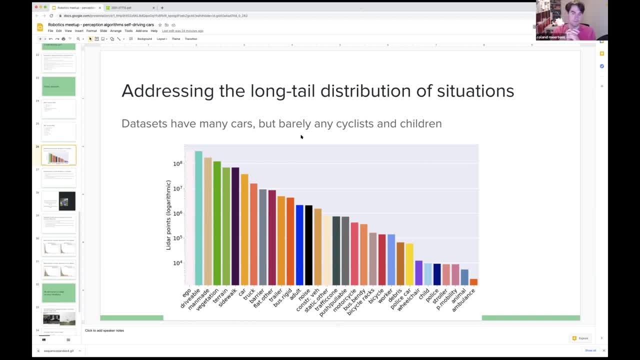 are the specific aspects of my, are the specific aspects of my algorithm. so i can algorithm, so i can algorithm, so i can do. like a formal proof that my algorithm do, like a formal proof that my algorithm do, like a formal proof that my algorithm or my self-driving car planner is always 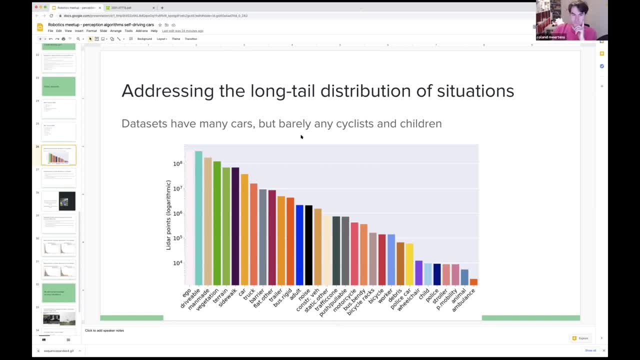 or my self-driving car planner is always- or my self-driving car planner is always- able to react to those able to react to those able to react to those things. yeah, i think it's uh. yeah, i'm really. yeah, i think it's uh. yeah, i'm really. 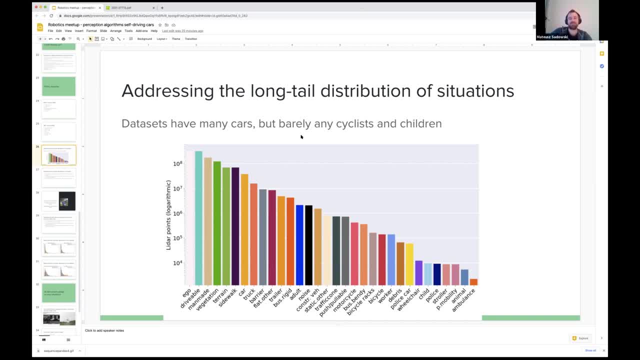 yeah, i think it's. uh, yeah, i'm really curious uh what he can curious, uh, what he can curious, uh what he can, yeah, where he can get with his ideas. yeah, where he can get with his ideas. yeah, where he can get with his ideas. it could be useful, but uh, i'm not in the 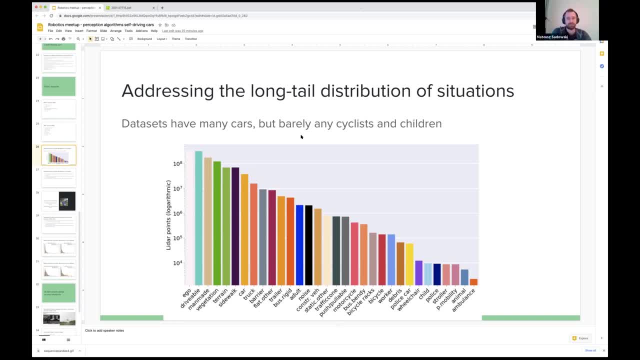 it could be useful, but uh, i'm not in the. it could be useful, but uh, i'm not in the industry at all. so i was wondering what industry at all. so i was wondering what industry at all. so i was wondering what you were thinking about this. 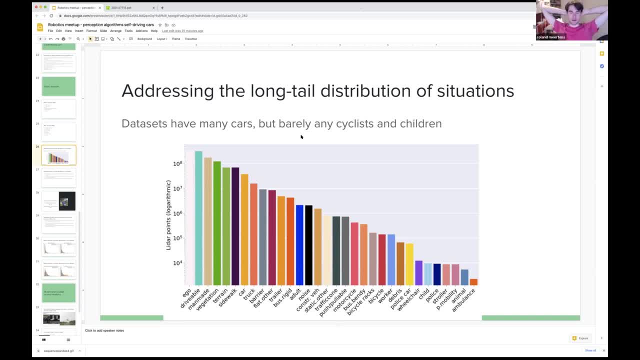 you were thinking about this. you were thinking about this. yeah, i i've read some articles from him. yeah, i, i've read some articles from him. yeah, i, i've read some articles from him and i think he has a, and i think he has a and i think he has a right. uh, right, critique points, um, which? 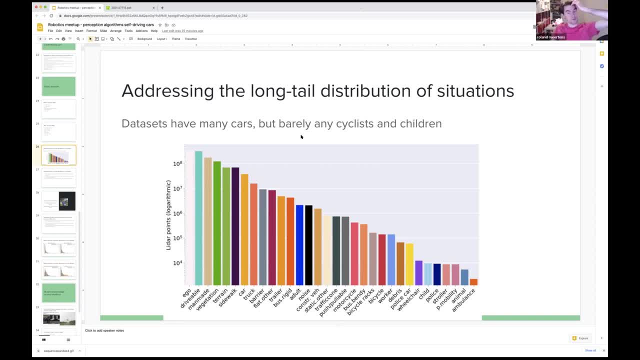 right, uh right, critique points um which right, uh right, critique points um which could be addressed, could be addressed, could be addressed. but yeah, i, i'm personally, i mean i'm, but yeah, i, i'm personally, i mean i'm, but yeah, i, i'm personally, i mean i'm personally trying to 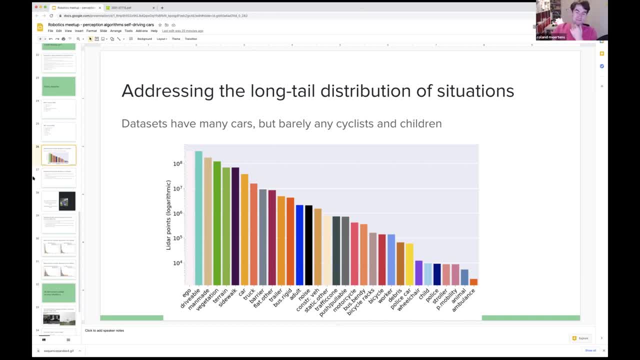 personally trying to, personally trying to get the or make safety cool again. get the or make safety cool again. get the or make safety cool again by just having a discussion like an, by just having a discussion like an, by just having a discussion like an open discussion with people like okay. 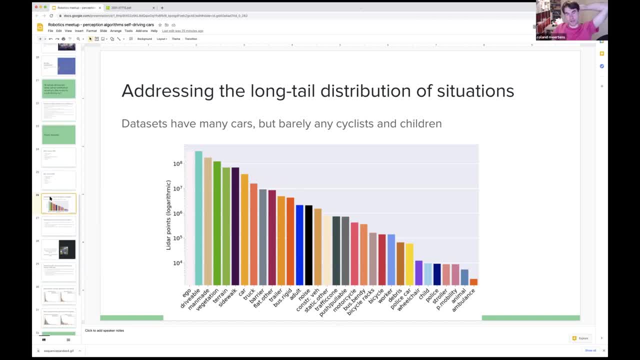 open discussion with people like: okay, open discussion with people like, okay, what's what would you like to see? what's what would you like to see? what's what would you like to see? i always see that people are really. i always see that people are really. i always see that people are really engaged in. 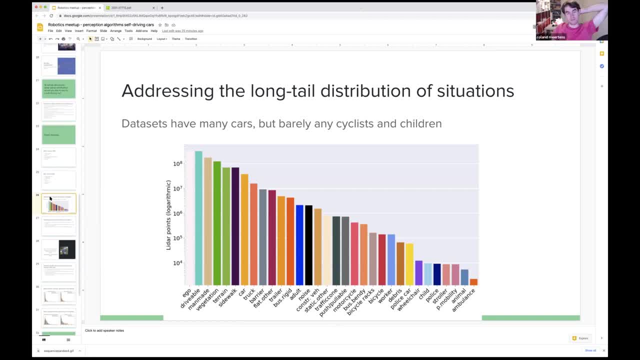 engaged in, engaged in in doing that and have great ideas and in doing that and have great ideas and in doing that and have great ideas and cool or make safety relevant and uh cool. or make safety relevant and uh cool. or make safety relevant and uh yeah, it's always interesting to see what. 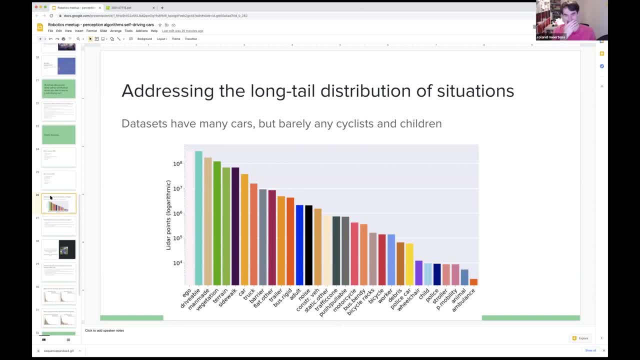 yeah, it's always interesting to see what. yeah, it's always interesting to see what they're doing. are there any more questions? now's the moment. it doesn't. now's the moment. it doesn't. now's the moment. it doesn't seem- yeah, doesn't seem like it. 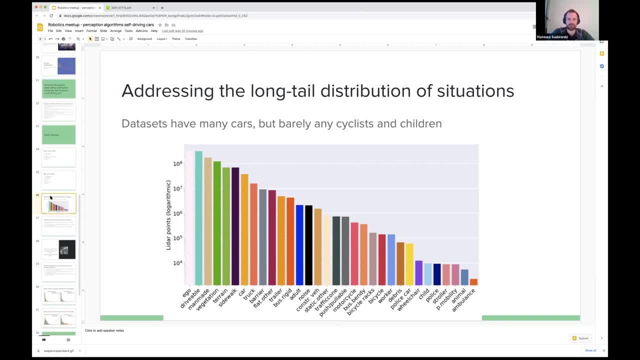 seem, yeah, doesn't seem like it. seem, yeah, doesn't seem like it. um, um, um, okay, then i think, uh, i think we can. okay, then i think, uh, i think we can. okay, then i think, uh, i think we can. oh, oh, oh, vinesh admitted, i saw it. vinesh admitted, i saw it. vinesh admitted, i saw it. yeah, actually, uh. so i just didn't want, yeah, actually, uh. so i just didn't want. yeah, actually, uh. so i just didn't want to push because we are well beyond the to push, because we are well beyond the. 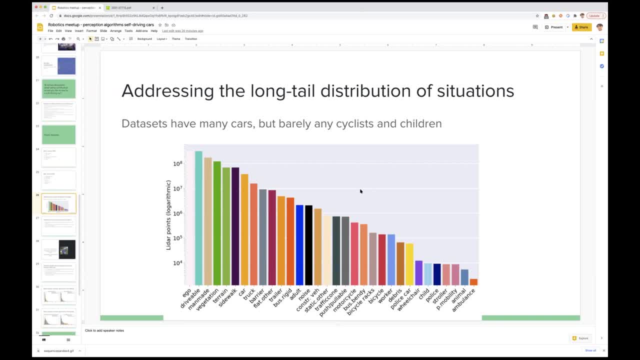 to push because we are well beyond the time limit. uh, on a very general note. uh, time limit? uh, on a very general note, uh, time limit? uh, on a very general note, uh, how? how do you see the um? how? how do you see the um? how? how do you see the um? eu's development towards, or uh? 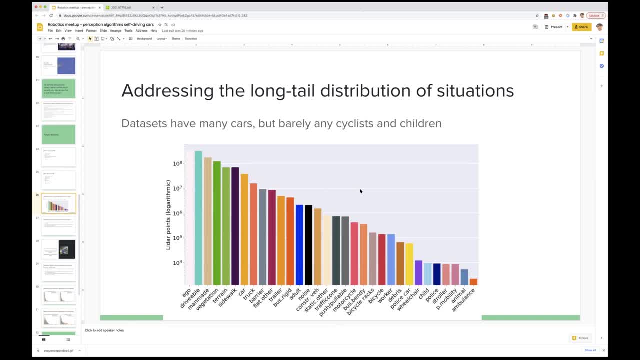 eu's development towards or uh. eu's development towards or uh. i would like to probably put it in a. i would like to probably put it in a fashion that um. fashion that um. fashion that um. the so-called competition between the uh. the so-called competition between the uh. 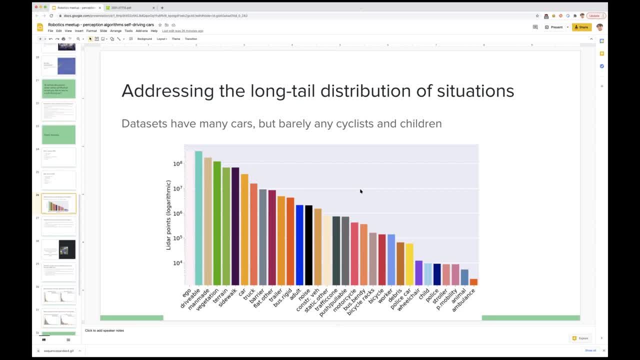 the so-called competition between the uh the american, the american, the american technology development towards technology development, towards technology development towards autonomous driving and the european autonomous driving and the european autonomous driving and the european style of development towards autonomous style of development, towards autonomous style of development, towards autonomous uh driving systems. because right now we 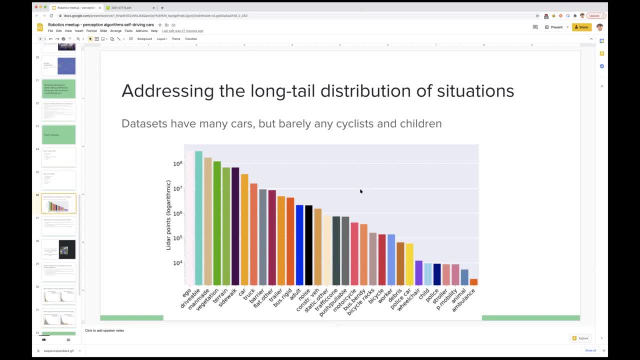 uh driving systems. because right now we uh driving systems, because right now we have have have zooks um and vemo and zooks um and vemo and zooks um and vemo and uh also different other players um uh also different other players um uh also different other players um in in the american market uh, but in the 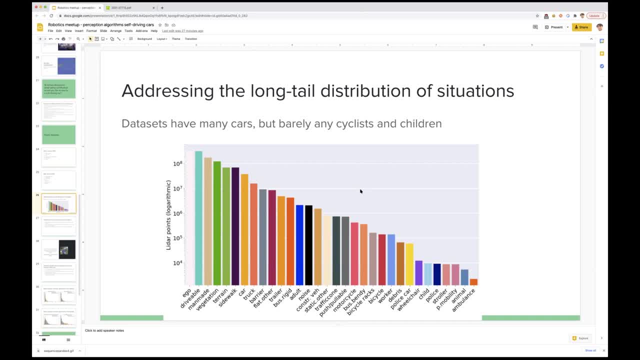 in in the american market, uh, but in the in in the american market, uh, but in the european market. i mean of course tesla european market. i mean of course tesla european market. i mean of course tesla. but on the european market we are in the. 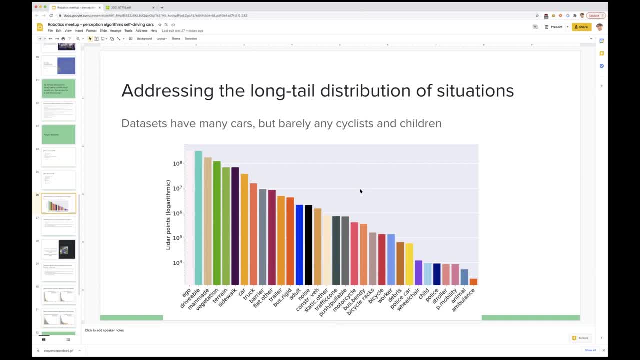 but on the european market. we are in the but on the european market. we are in the verge of verge of verge of uh, i would say still slow, steady, and uh, i would say still slow, steady, and uh, i would say still slow, steady, and also at a standard level, uh, probably. 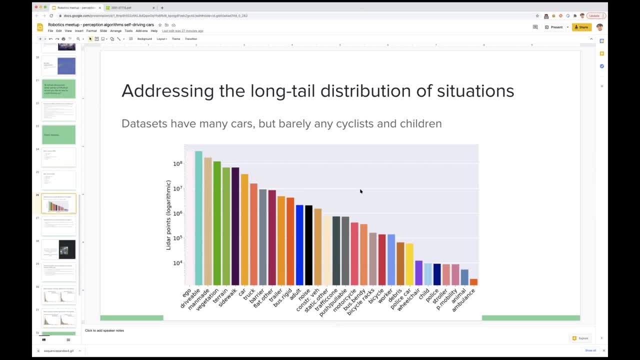 also at a standard level. uh, probably also at a standard level. uh, probably, that's how, that's how, that's how the uh, the cultural waypoint of the uh, the cultural waypoint of the uh, the cultural waypoint of development is at least within european development is at least within european. 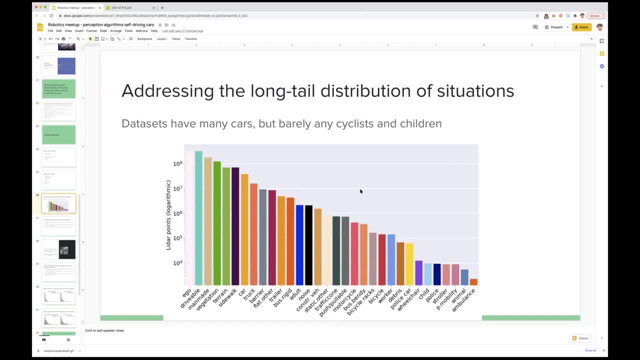 development is, at least within european countries, countries, countries, and um, would it be again a ground up, and um, would it be again a ground up? technology development, or would it be technology development? or would it be technology development or would it be like, like, like, um re-engineering of what the uh, the? 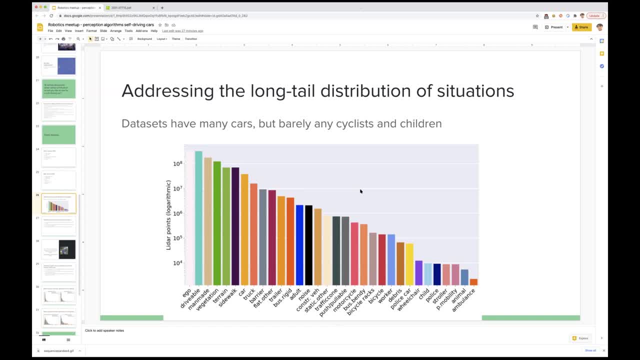 um re-engineering of what the uh, the um re-engineering of what the uh. the technology is going on at uh. technology is going on at uh. technology is going on at uh, for example in america- yeah, i mean in. for example in america, yeah, i mean in. 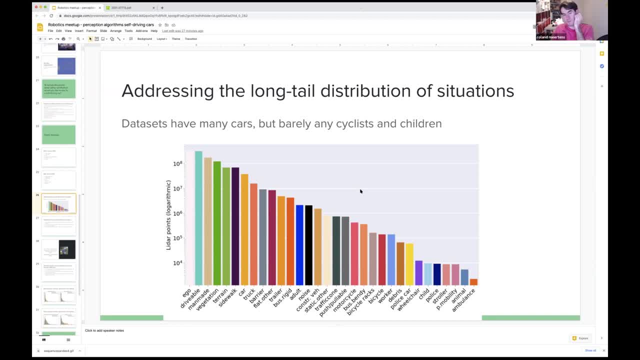 for example, in america. yeah, i mean in terms of terms of terms of uh in terms of geography, uh in munich, we uh in terms of geography, uh in munich, we uh in terms of geography, uh in munich, we had a couple of self-driving car. 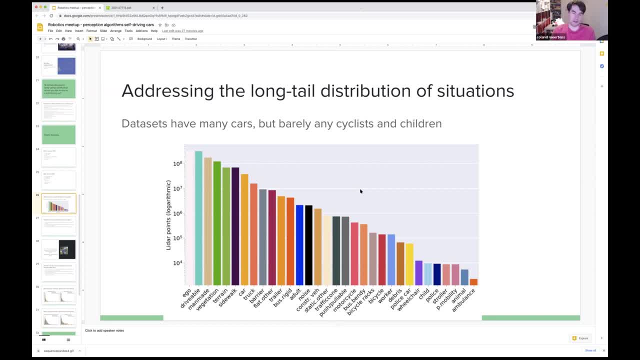 had a couple of self-driving car, had a couple of self-driving car companies, right, so we had uh companies, right, so we had uh companies, right, so we had uh. we had aid, which is now part of argo, so we had aid, which is now part of argo. so 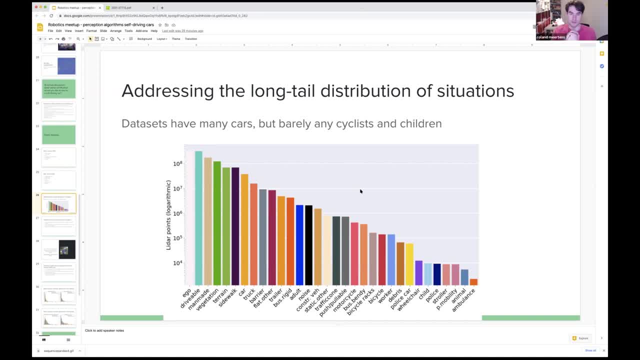 we had aid, which is now part of argo, so argo has a european headquarters, which argo has a european headquarters, which argo has a european headquarters, which is really nice. so at least they are is really nice. so at least they are is really nice. so at least they are going to test uh things here in. 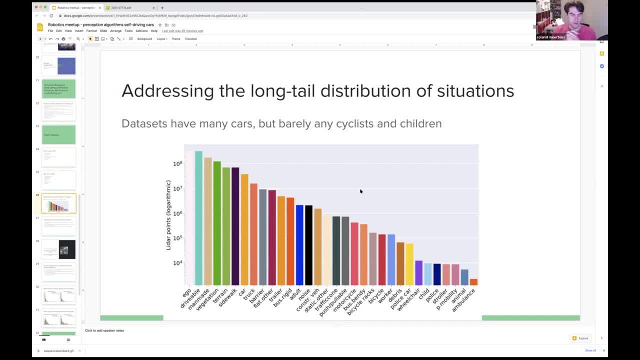 going to test uh things here in. going to test uh things here in munich and hamburg. um so there is munich and hamburg. um so there is munich and hamburg. um so there is. there are some developments towards. there are some developments towards. there are some developments towards also getting cars and roads here. 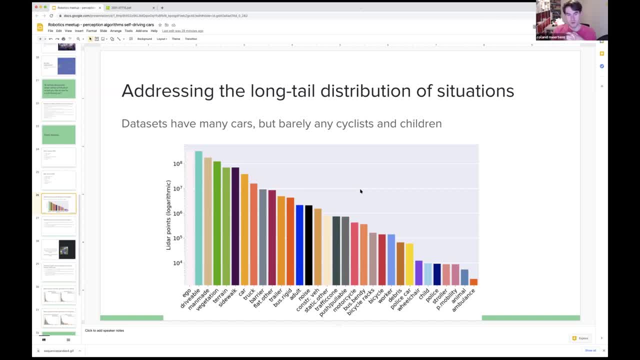 also getting cars and roads here- also getting cars and roads here. um, we also had a lift level five office. um, we also had a lift level five office. um, we also had a lift level five office here in munich a while ago. uh, but i here in munich a while ago, uh, but i. 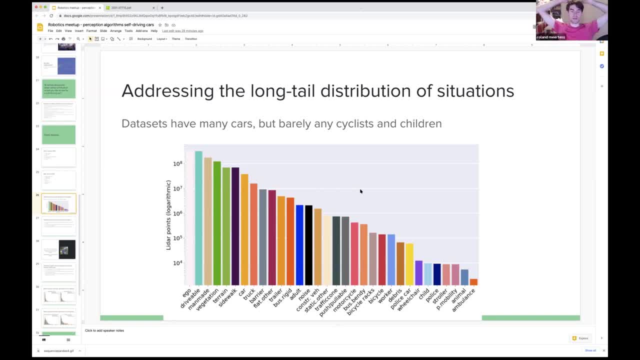 here in munich a while ago, uh, but i think they're not stopped, um, think they're not stopped, um, think they're not stopped um, so there is, there is some development, so there is, there is some development, so there is there is some development. uh, going on in europe, no, no, i, i. uh going on in europe. no, no, i, i uh going on in europe. no, no, i. i completely agree with that. i mean i'm completely agree with that. i mean i'm completely agree with that. i mean i'm not saying that there's no development, not saying that there's no development. 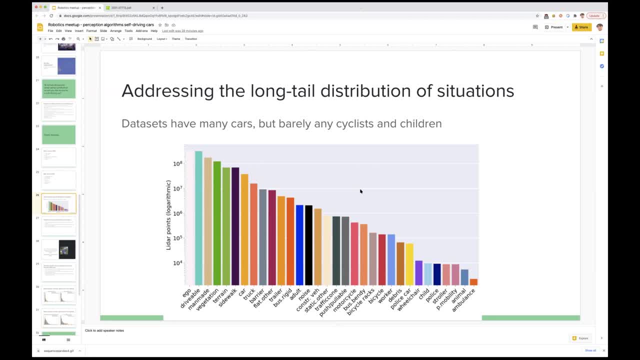 not saying that there's no development, like. i'm just talking about the pace of like. i'm just talking about the pace of like. i'm just talking about the pace of the development, for example. the development, for example, the development, for example. uh, right now we have the shuttles from. 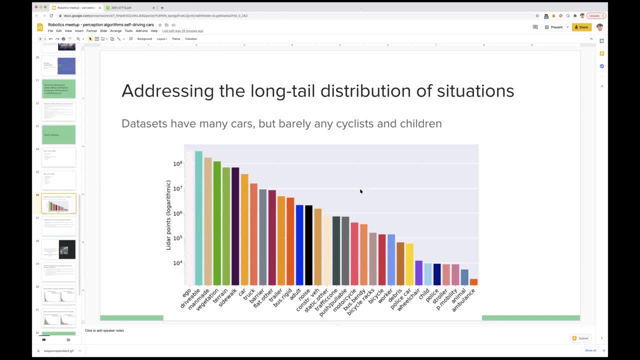 uh, right now we have the shuttles from: uh. right now we have the shuttles from. zed of get to there. uh, in germany, that's zed of get to there. uh, in germany, that's zed of get to there. uh, in germany, that's also. 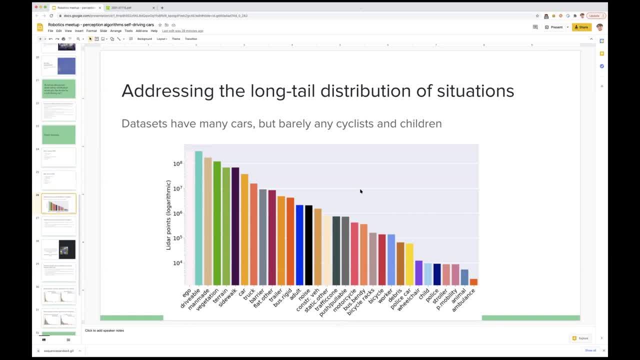 also also uh in pipeline and a lot of um uh in pipeline and a lot of um uh in pipeline and a lot of um taxes, for example, shuttle taxes from taxes. for example, shuttle taxes from taxes. for example, shuttle taxes from different companies. uh uh in berlin, or. 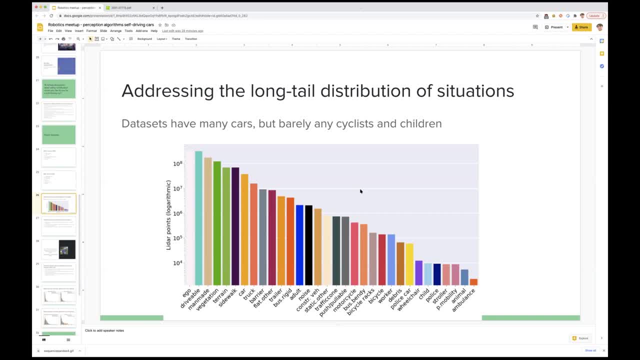 different companies- uh uh, in berlin, or different companies, uh uh, in berlin, or hamburg, for example, hamburg, for example, hamburg, for example. where, yeah, yeah, so i mean i completely where, yeah, yeah, so i mean i completely where, yeah, yeah. so i mean i completely agree to the development on that point. 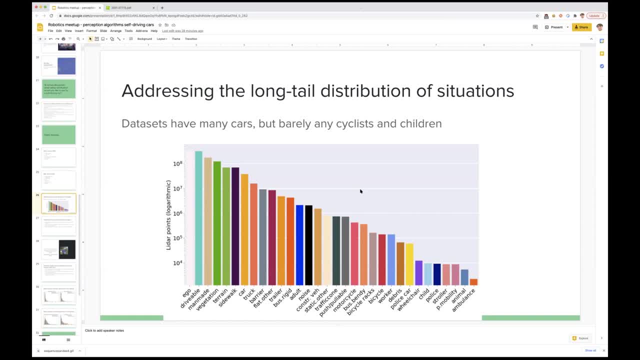 agree to the development on that point. agree to the development on that point, something like that, or would it be like something like that. or would it be like something like that. or would it be like uh, uh, uh, more of uh cooperational development, more of uh cooperational development. 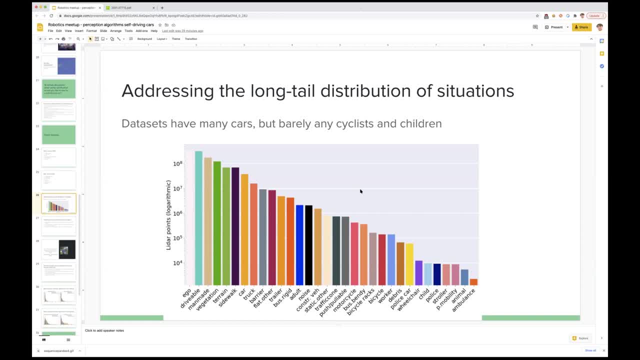 more of uh cooperational development. that would happen. that would happen. that would happen. like i said, it was our general point and, like i said, it was our general point and, like i said, it was our general point and not uh, not uh, not uh specific on the topic that we're. 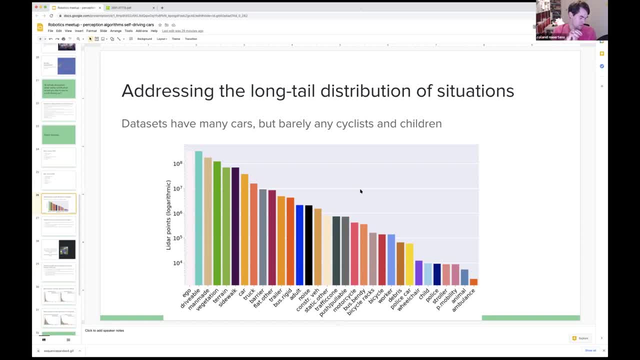 specific on the topic that we're specific on the topic that we're discussing, discussing, discussing- yeah, maybe one uh one other uh. i mean, yeah, maybe one uh, one other uh. i mean, yeah, maybe one uh, one other uh. i mean, i'm now just going to get loads of. 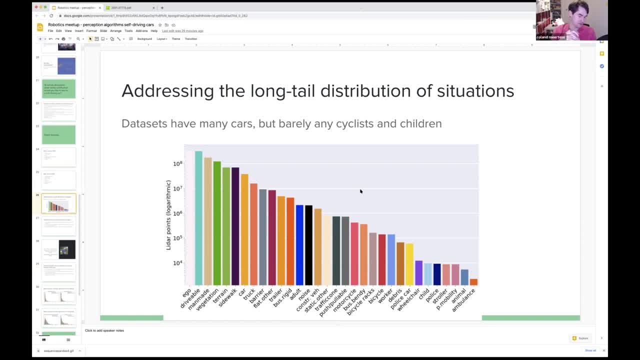 i'm now just going to get loads of. i'm now just going to get loads of opinions on things, right, but uh, so, opinions on things, right, but uh, so, maybe one other thing which might play, maybe one other thing which might play, maybe one other thing which might play. play a bit of a role, is that? 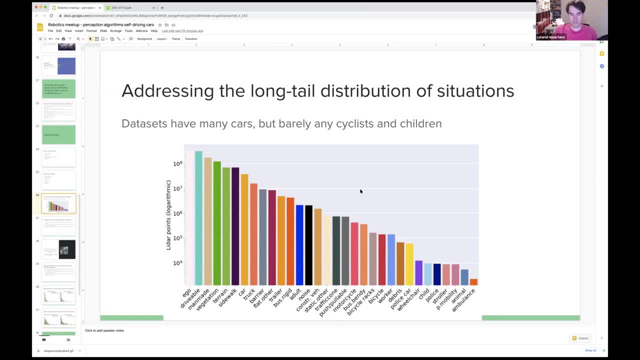 play a bit of a role. is that play a bit of a role? is that in america you can self-certify. in america, you can self-certify. in america, you can self-certify vehicles, vehicles, vehicles. so you can basically deploy something, and so you can basically deploy something, and 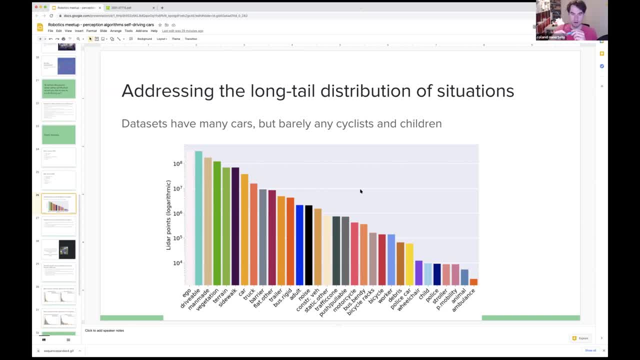 so you can basically deploy something and then you're responsible for whatever. then you're responsible for whatever. then you're responsible for whatever happens to it. happens to it, happens to it, but you don't have to show up front. but you don't have to show up front. 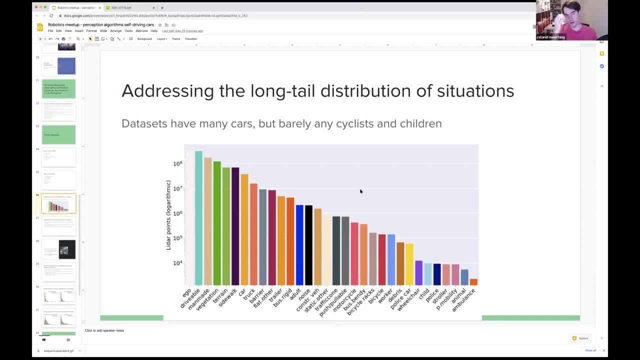 but you don't have to show up front. what's uh that your vehicle is safe to what's uh that your vehicle is safe to what's uh that your vehicle is safe to go on the road? go on the road, go on the road. whereas in europe, 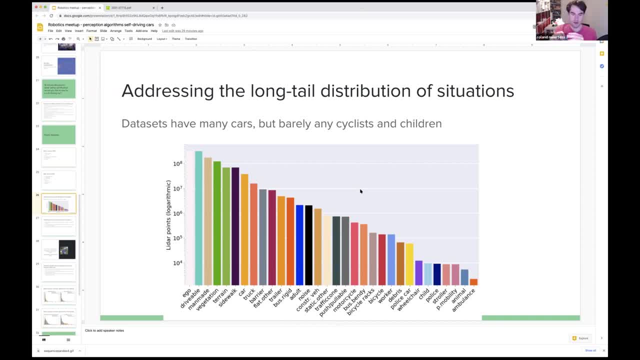 whereas in europe. whereas in europe, we have the tough uh germany and the. we have the tough uh germany and the we have the tough uh germany and the la way, la way, la way. in the netherlands, who are all assessing. in the netherlands, who are all assessing. 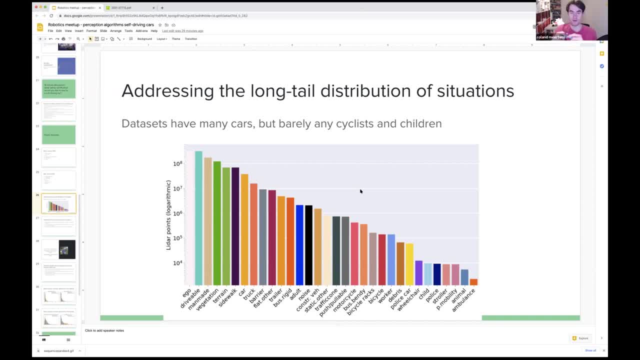 in the netherlands, who are all assessing uh vehicles before they uh vehicles, before they uh vehicles, before they are allowed to go onto the road. so that's are allowed to go onto the road. so that's are allowed to go onto the road. so that's also different. 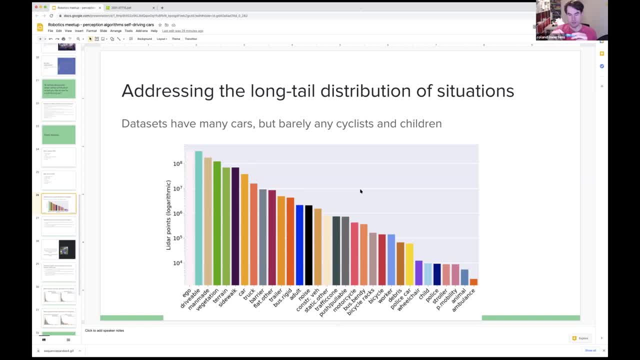 also different, also different. so you see that in london, for example. so you see that in london, for example. so you see that in london, for example, there's already a bit more self-driving, there's already a bit more self-driving, there's already a bit more self-driving car companies, because there you can just 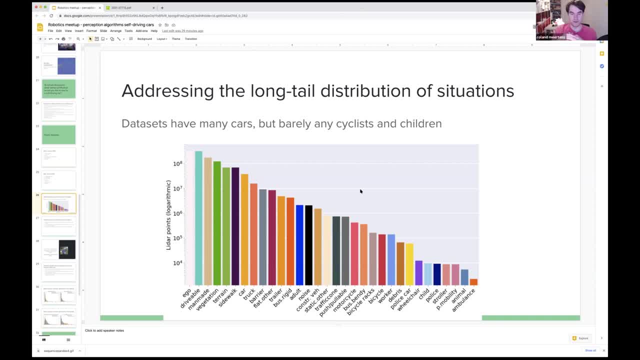 car companies, because there you can. just car companies, because there you can, just as long as you're in the driver's seat, as long as you're in the driver's seat, as long as you're in the driver's seat, and safety driver, and safety driver and safety driver, you're, uh, you're responsible um. 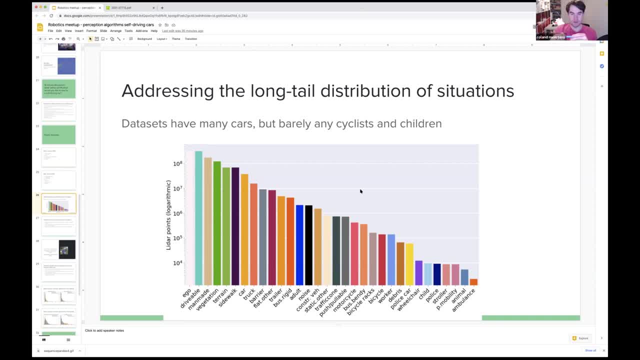 you're, uh, you're responsible, um, you're, uh, you're responsible, um, whereas with ad, we always had, we had to. whereas with ad, we always had, we had to. whereas with ad, we always had, we had to spend a lot of time to spend a lot of time to. 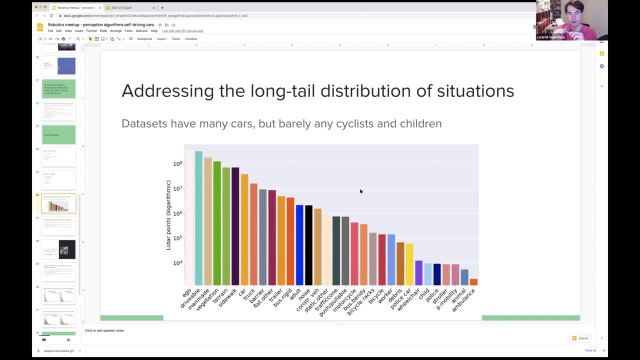 spend a lot of time to get our car approved to go on the road. get our car approved to go on the road. get our car approved to go on the road with a safety driver, with a safety driver, with a safety driver. so in america it might be easier to start. 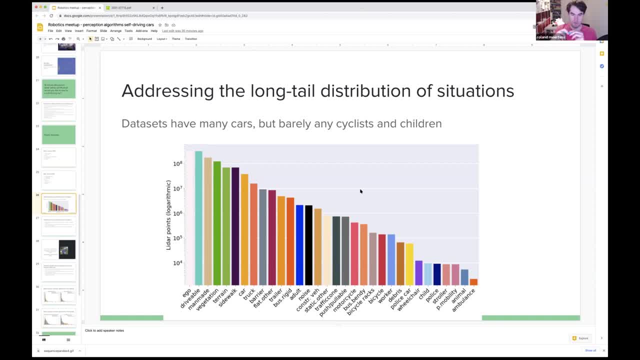 so in america it might be easier to start. so in america it might be easier to start a self-driving car company, a self-driving car company, a self-driving car company. and then there's of course also loads of, and then there's of course also loads of. 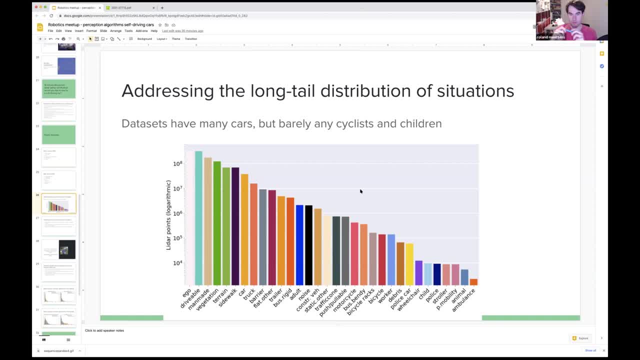 and then there's of course also loads of um knowledge already in uh in america, um knowledge already in uh in america, um knowledge already in uh in america. loads of, loads of, loads of. maybe more money, uh, which could play a. maybe more money, uh, which could play a. 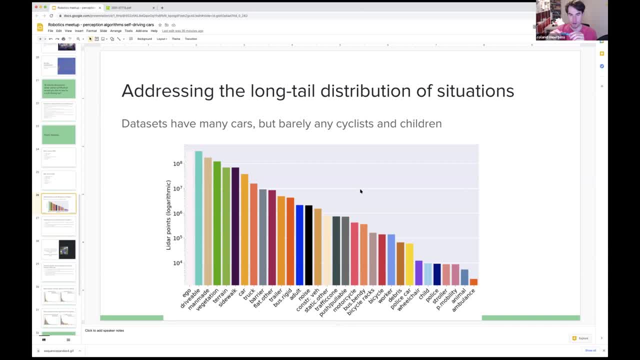 maybe more money, uh, which could play a role, um, role, um, role, um. but yeah, there's definitely some, but yeah, there's definitely some, but yeah, there's definitely some interesting european players, uh, interesting european players, uh, interesting european players, uh, um, but those, those might be um, but those, those might be. 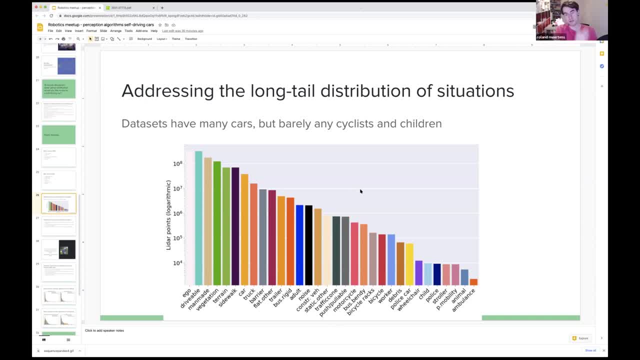 um, but those, those might be, those might be a couple of reasons that, uh, those might be a couple of reasons that, uh, those might be a couple of reasons that, uh, maybe the other thing is the maybe the other thing is the maybe the other thing is the traditional automotive world. 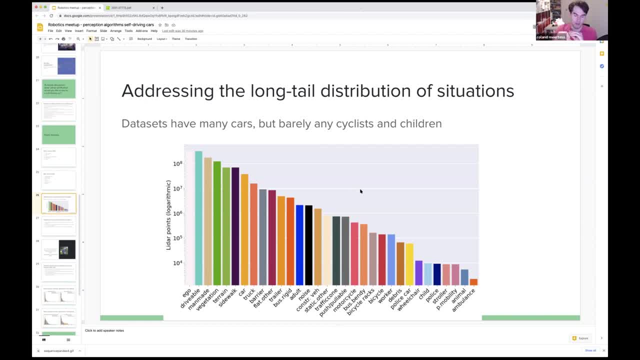 traditional automotive world, traditional automotive world they are often relying on. they are often relying on, they are often relying on, traditionally relying on third-party, traditionally relying on third-party, traditionally relying on third-party vendors. so now vendors, so now vendors, so now volkswagen did make a good start by 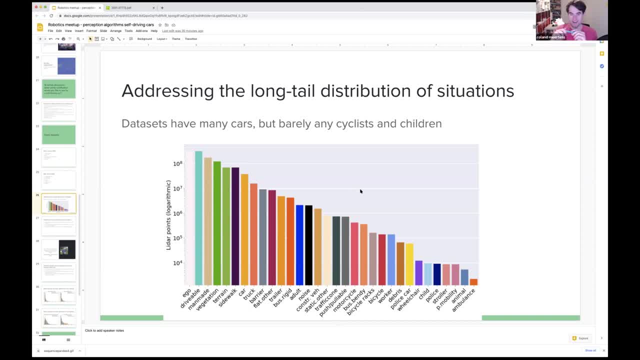 volkswagen did make a good start by. volkswagen did make a good start by having uh carry ads. that's their new having uh carry ads. that's their new having uh carry ads. that's their new car software organization, car software organization, car software organization. so they are, they are trying to uh. 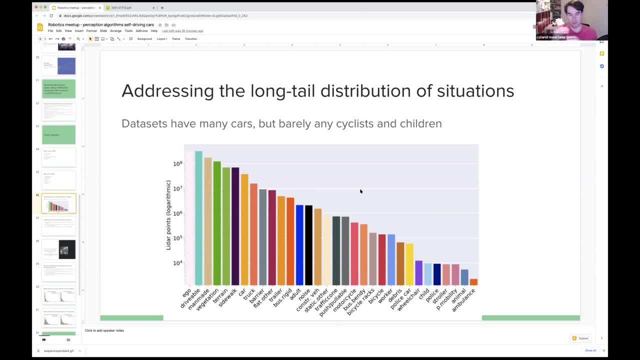 so they are. they are trying to uh start this right. so they are now start this right. so they are now start this right. so they are now setting up their own internal software. setting up their own internal software, setting up their own internal software, development for uh, for um. 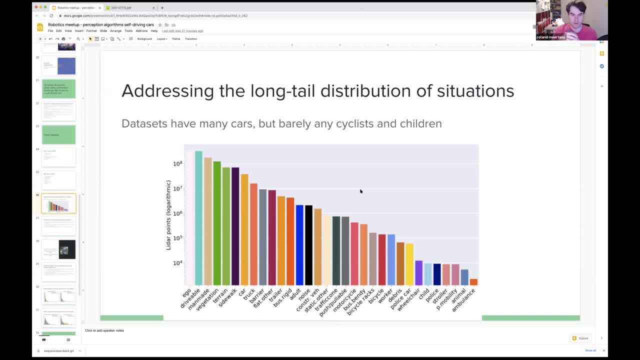 development for uh for um development for uh for um self-driving functionality: uh or self-driving functionality: uh or self-driving functionality, uh, or overall the software functionality: uh, overall the software functionality, uh, overall the software functionality: uh. so it is catching up or it is. it is uh. 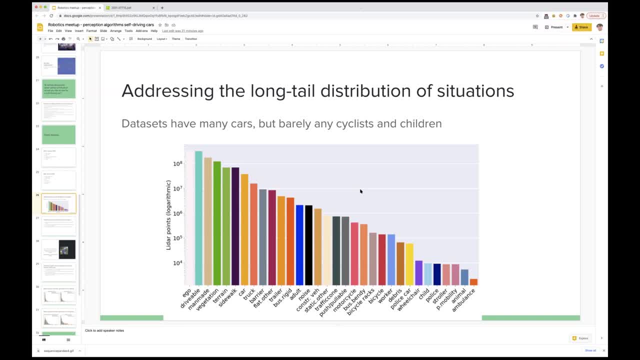 so it is catching up, or it is. it is uh, so it is catching up, or it is. it is uh, now joining the game um. but yeah, now joining the game um. but yeah, now joining the game um. but yeah, perfect, thank you. other questions? other questions? other questions? um, yeah, hi roger. 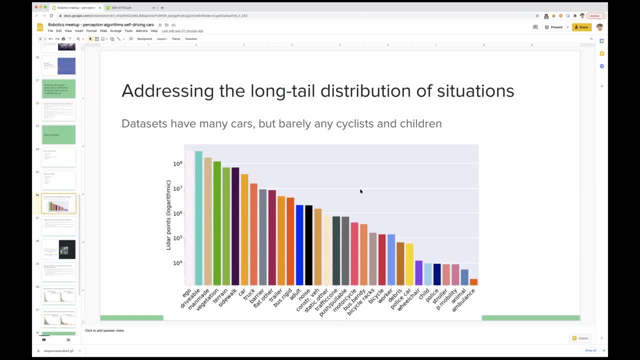 um, yeah, hi roger. um yeah, hi roger. i wanted to brief about like any more. i wanted to brief about like any more. i wanted to brief about like any more. open source software developments like open source software developments, like open source software developments like, which could help all of them. so there, 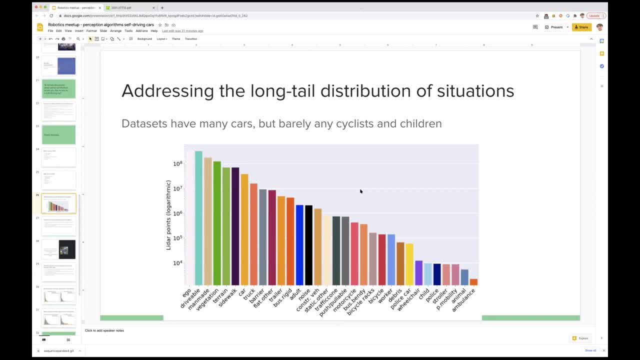 which could help all of them. so there which could help all of them. so there are a few of them. are a few of them. are a few of them currently right now, uh, any currently right now, uh, any currently right now, uh any like i've uh seen apollo and 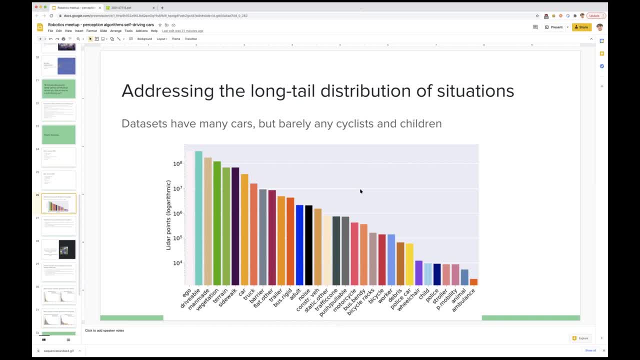 like i've uh seen apollo and like i've uh seen apollo and autoware. but any more autoware, but any more autoware, but any more of them like uh, which could really be of them, like uh, which could really be of them like uh, which could really be worth looking into, or anything like 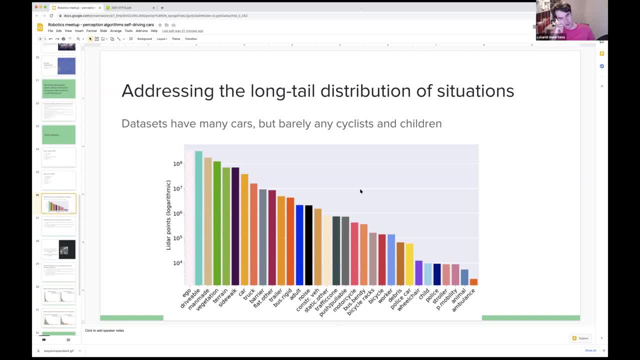 worth looking into or anything like worth looking into or anything like: yeah, in terms of the open source, yeah, in terms of the open source, yeah, in terms of the open source projects. i think apollo is really projects. i think apollo is really projects. i think apollo is really interesting because it's really a 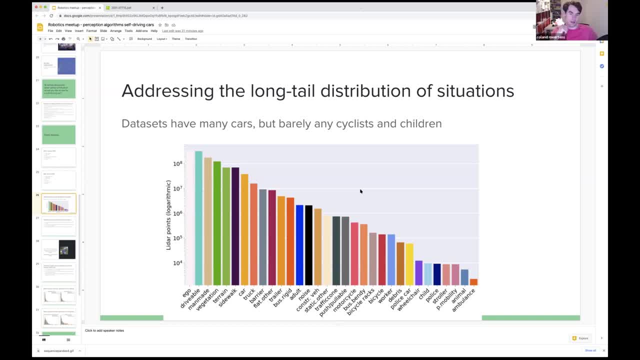 interesting because it's really a interesting because it's really a self-driving car like a complete stack, self-driving car, like a complete stack, self-driving car, like a complete stack and has lots of high level algorithms and has lots of high level algorithms and has lots of high level algorithms. so if you look at their approaches, they 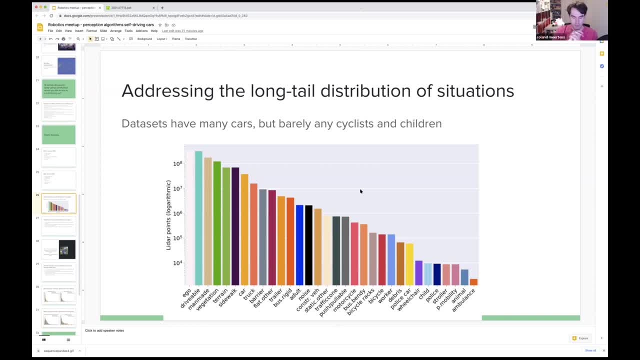 so if you look at their approaches, they. so if you look at their approaches, they, they all make lots of sense and they're they all make lots of sense and they're they all make lots of sense and they're really interesting, really interesting, really interesting. um, and that's really to bootstrap a 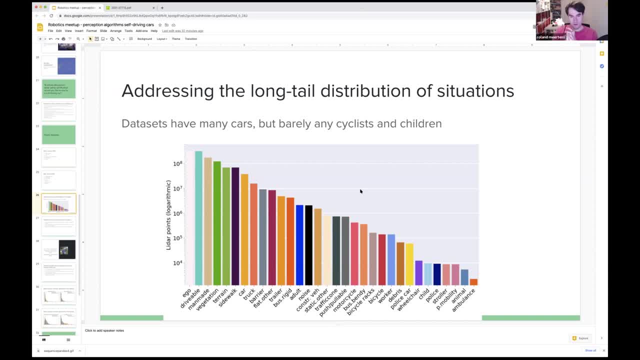 um, and that's really to bootstrap a um, and that's really to bootstrap a whole uh, surviving car taxi service. what i really like about outerwear is what i really like about outerwear is. what i really like about outerwear is that they are, that they are. 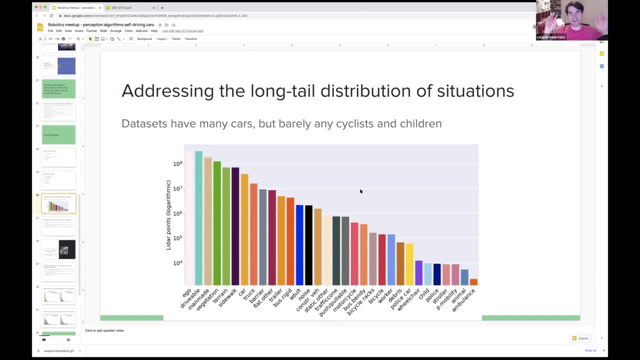 that they are starting from the safety case. so starting from the safety case, so starting from the safety case, so basically, basically, basically, uh, apollo is approaching it from let's uh apollo is approaching it from. let's uh apollo is approaching it from. let's just add some functionality and then we 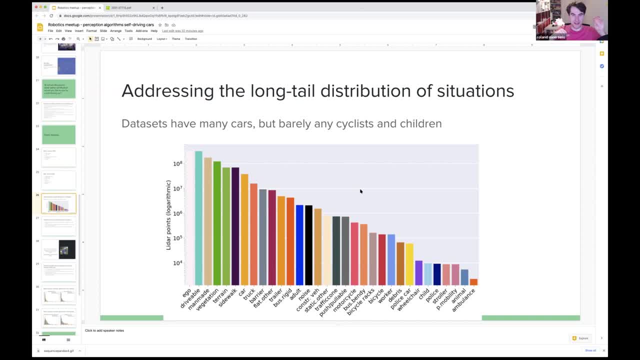 just add some functionality, and then we just add some functionality, and then we can later see how we can certify it, and can later see how we can certify it, and can later see how we can certify it. and outerwear seems to go from okay well. outerwear seems to go from okay, well. 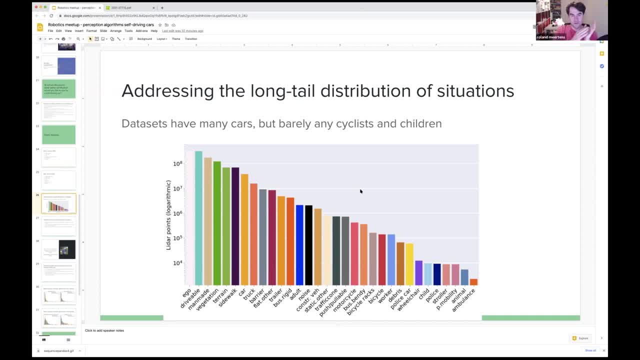 outerwear seems to go from okay. well, let's start with the basis we can. let's start with the basis we can. let's start with the basis we can certify, certify: uh to put in every car, and then we can. uh to put in every car, and then we can. 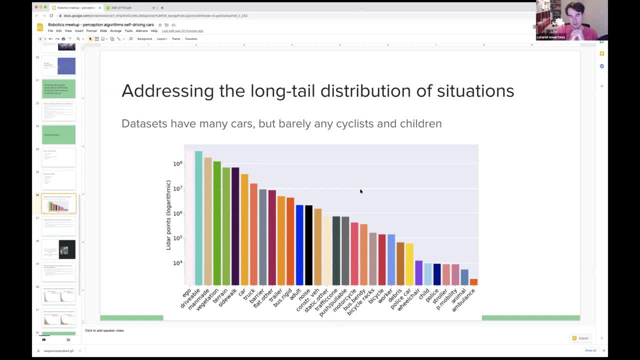 uh, to put in every car, and then we can see what, see what, see what kind of functions we can add later on kind of functions we can add later on, kind of functions we can add later on top of that of the already certified, top of that of the already certified. 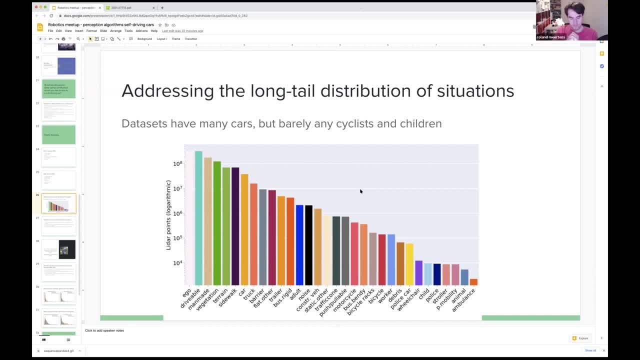 top of that of the already certified stack, stack, stack. so that's that's a big difference. um, so, that's, that's a big difference. um, so that's that's a big difference. um, but yeah, i don't know, uh, but yeah, i don't know uh. 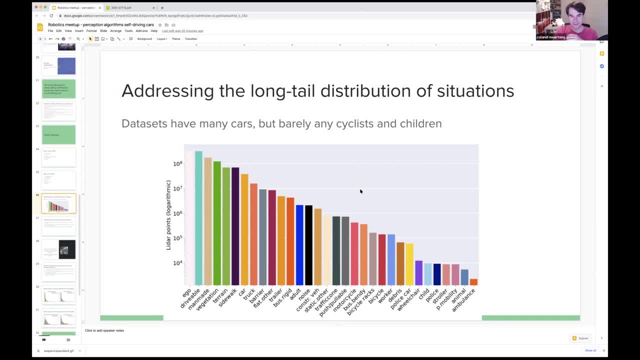 but yeah, i don't know, uh, i don't have any other. i mean those are my, i don't have any other. i mean those are my, i don't have any other. i mean those are my opinions on the on the two projects. opinions on the on the two projects. 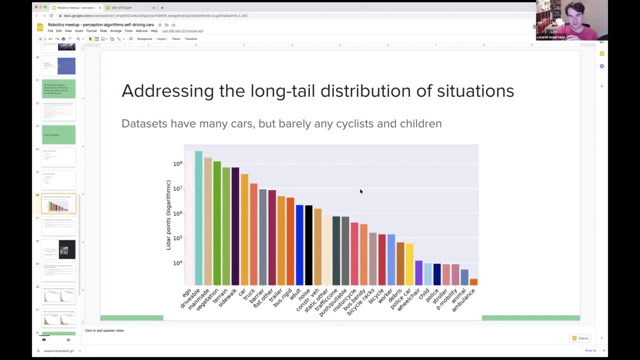 opinions on the on the two projects you just mentioned. uh, you just mentioned. uh, you just mentioned: uh, comma ai is also open source, right, uh, comma ai is also open source, right, uh, comma ai is also open source, right, uh. so there you can see what they are. 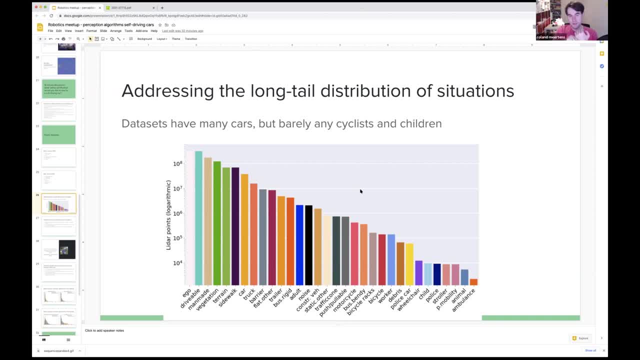 so there you can see what they are. so there you can see what they are using, i think um, using, i think um, using, i think um, but that's of course again level two, but that's of course again level two, but that's of course again level two system um. 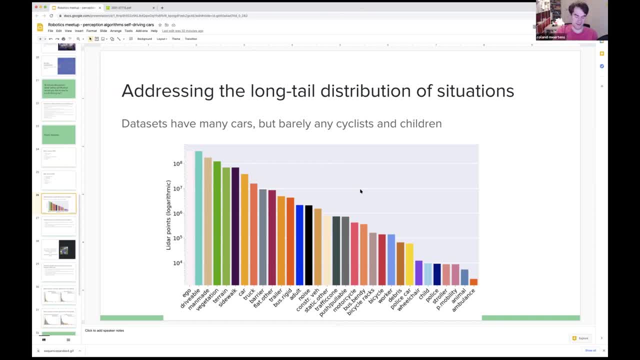 system, um, system, um, and there are the safety certifications and there are the safety certifications and there are the safety certifications also, also, also, i don't know, it's mostly, mostly unit tests. i don't know it's mostly, mostly unit tests. i don't know, it's mostly mostly unit tests. and, uh, you as a driver are always 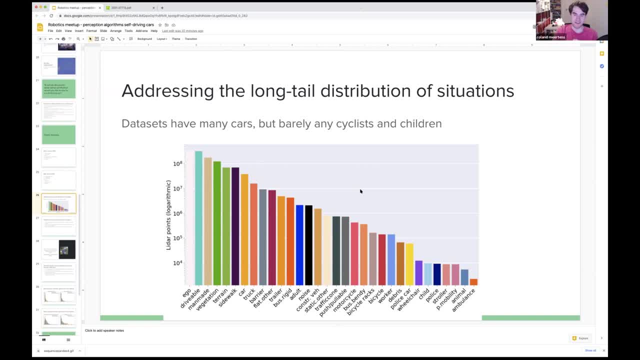 and uh, you, as a driver, are always, and uh, you, as a driver, are always responsible. that's uh responsible, that's uh responsible. that's uh. that's the message. they are a safety. uh, that's the message. they are a safety. uh, that's the message. they are a safety, uh. document is literally a readmetxt. 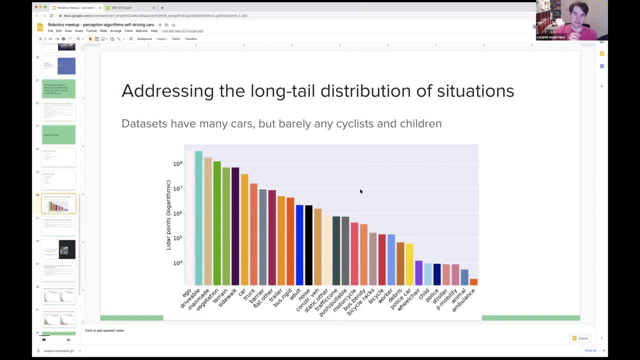 document is literally a readmetxt. document is literally a readmetxt. which is interesting, which is interesting, which is interesting, um, but yeah, so there's a. there's a um, but yeah, so there's a. there's a um, but yeah, so there's a. there's a couple of open source projects, um. 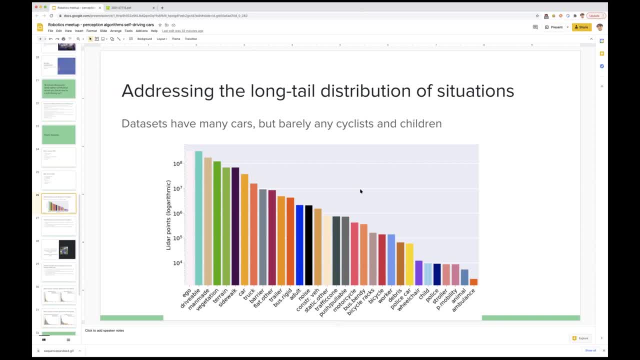 thanks, it wouldn't fire you like that's thanks. it wouldn't fire you like that's thanks. it wouldn't fire you like that's very important, very important, very important. thank you, no more questions. thank you, no more questions. thank you, no more questions. let me add one more, uh, one more. 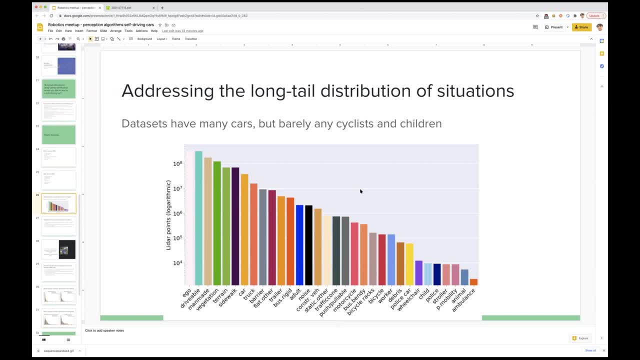 let me add one more, uh, one more. let me add one more, uh, one more question, uh, but first, uh, thanks for the question, uh, but first, uh, thanks for the question, uh, but first, uh, thanks for the presentation. was presentation was presentation, was that was nice to see, um, so, but then let. 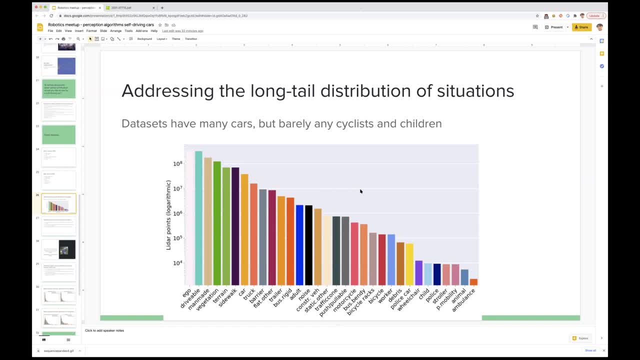 that was nice to see, um so, but then let. that was nice to see, um so, but then let me ask the hardest questions. i guess me ask the hardest questions. i guess me ask the hardest questions. i guess uh, and that is when, uh, and that is when. 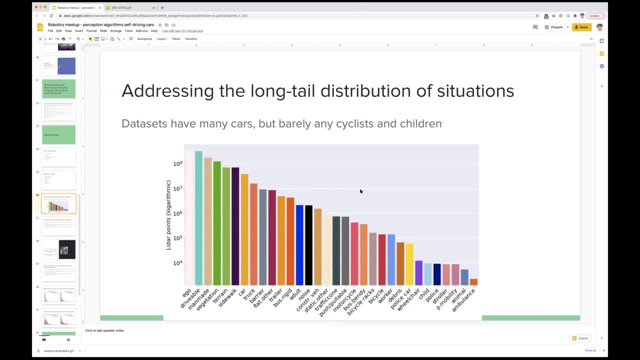 uh, and that is when: yeah, good question. so, yeah, good question. so, yeah, good question. so is there an answer? is there an answer? is there an answer? i think the biggest question is how to. i think the biggest question is how to. i think the biggest question is how to scale uh. 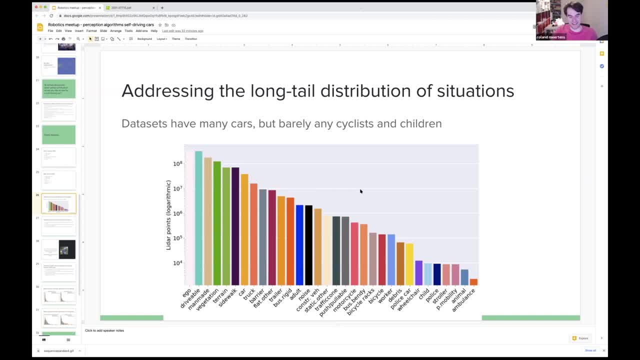 scale, uh, scale, uh. maybe then because uh, when is already now. maybe then because, uh, when is already now. maybe then because, uh, when is already now, because you can already uh, because you can already uh, because you can already uh, you can already book uh rights with waymo. 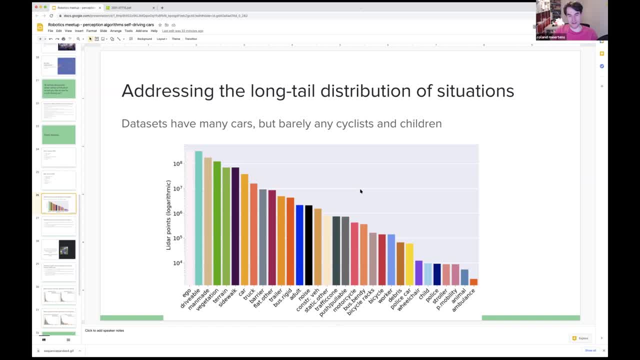 you can already book uh rights with waymo. you can already book uh rights with waymo, right? so there's already level four. right, so there's already level four. right, so there's already level four. driving driving: driving in a very limited area- uh, i can in a very limited area, uh, i can. 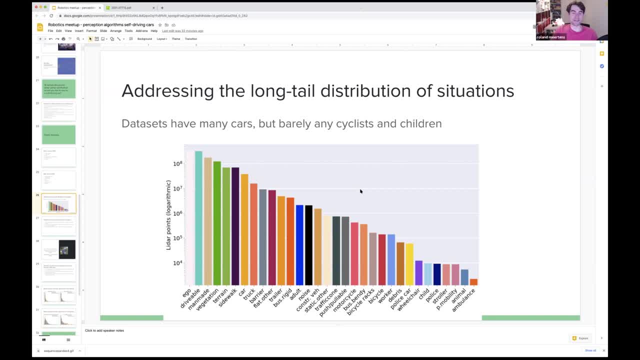 in a very limited area. uh, i can actually recommend, actually recommend, actually recommend the. i i really like watching, uh watching the. i i really like watching, uh watching the. i i really like watching, uh watching videos of several cars, videos of several cars, videos of several cars. it's my, it's my hobby. 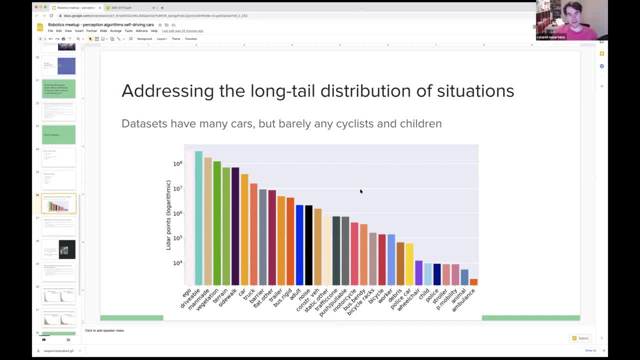 but there's, uh, there's loads of, but there's uh, there's loads of, but there's, uh, there's loads of interesting videos from jj wright, who is interesting videos from jj wright, who is riding a lot with waymo. he also has a riding a lot with waymo. he also has a. 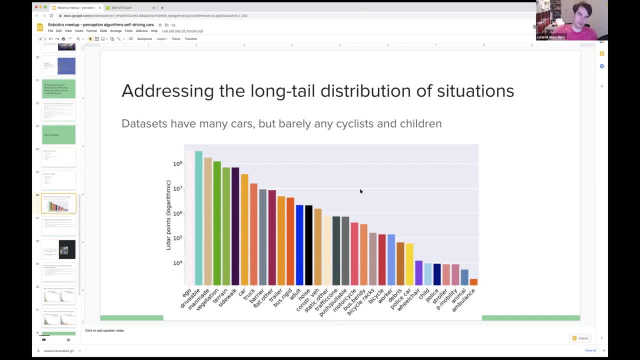 riding a lot with waymo. he also has a spreadsheet where you can see that spreadsheet, where you can see that spreadsheet, where you can see that, over the years that he has written with, over the years that he has written with, over the years that he has written with waymo, they are more and more completely. 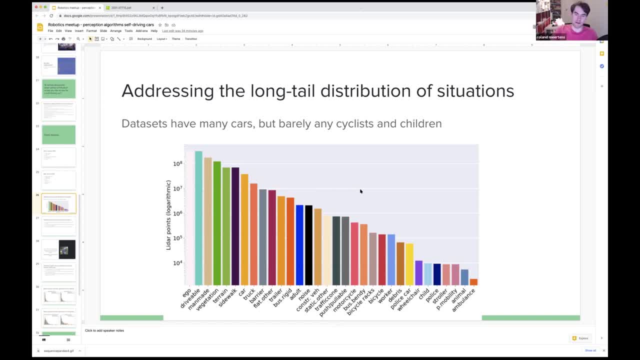 waymo. they are more and more completely waymo. they are more and more completely driverless, driverless, driverless. um. i think this morning he actually had um. i think this morning he actually had um. i think this morning he actually had a really terrible video where he 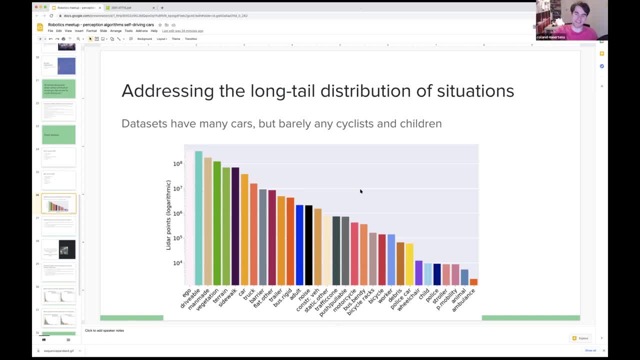 a really terrible video where he a really terrible video where he actually had a big problem, where the car actually had a big problem, where the car actually had a big problem, where the car like couldn't handle a construction zone, like couldn't handle a construction zone, but then they are quick to fix it. so now 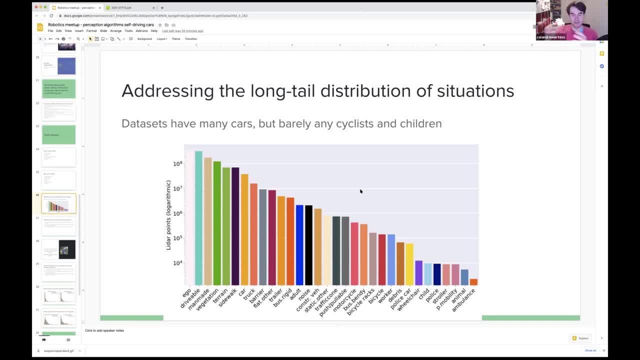 but then they are quick to fix it. so now, but then they are quick to fix it, so now. the question is: how can waymo scale this? the question is: how can waymo scale this? the question is: how can waymo scale this to multiple cities? um, how can they add? 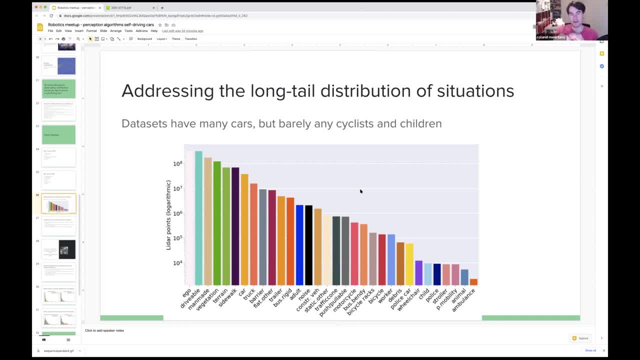 to multiple cities? um, how can they add to multiple cities? um, how can they add more uh streets or their odd? how can more uh streets or their odd? how can more uh streets or their odd? how can they, they, they, uh, make this a worldwide thing? um, so. 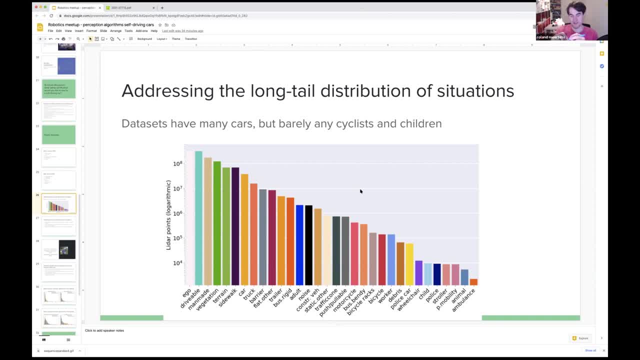 uh, make this a worldwide thing. um so, uh, make this a worldwide thing. um so, things are already possible now. uh, the things are already possible now. uh, the things are already possible now. uh, the question is: how can you question? is how can you question? is how can you expand your, uh, your number of streets? 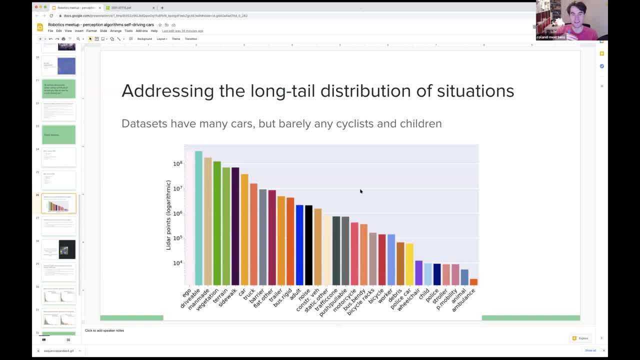 expand your, uh, your number of streets. you're driving and they say, maybe you're driving. and they say, maybe you're driving and they say, maybe, overfit to one area, overfit to one area, overfit to one area, or it's a problem really hard, we don't. 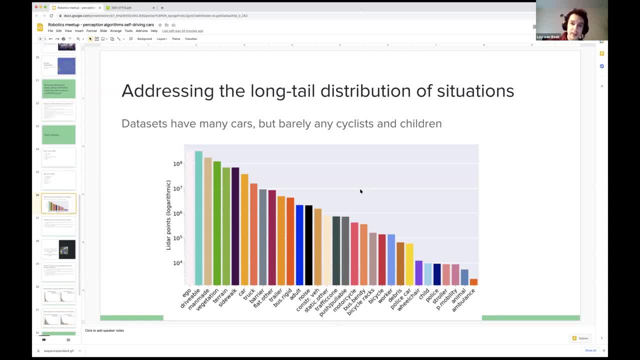 or it's a problem really hard, we don't, or it's a problem really hard we don't know, know, know, thanks, yeah, very interesting. yeah, super thanks. yeah very interesting. yeah, super thanks. yeah, very interesting. yeah, super interesting stuff, cool, all right. so if there are no more, 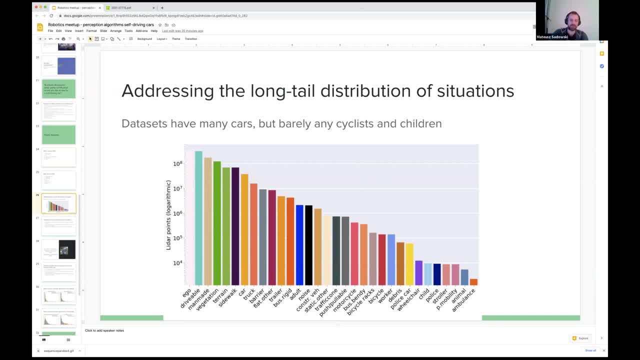 cool, all right. so if there are no more cool, all right. so if there are no more questions, questions, questions, uh, then i think, uh, we can finish. uh, uh, then i think, uh, we can finish. uh, uh, then, i think, uh, we can finish, uh. thanks a lot for the presentation was. 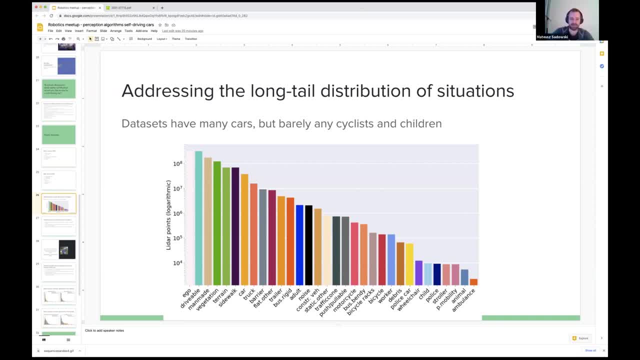 thanks a lot for the presentation was. thanks a lot for the presentation was really good, really good, really good, and uh, it was nice to have that and uh, it was nice to have that and uh, it was nice to have that discussion. i think it changed that in. 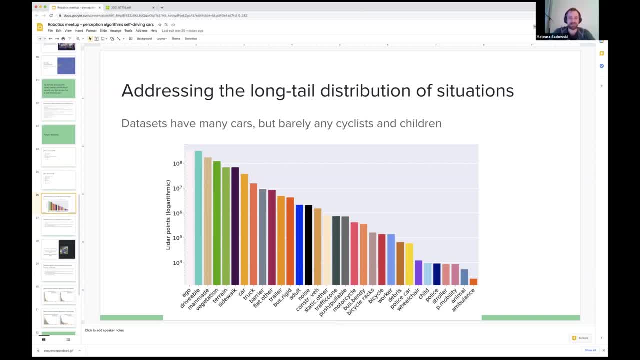 discussion. i think it changed that in discussion. i think it changed that in dynamics, dynamics, dynamics. i want to have more of this in the. i want to have more of this in the. i want to have more of this in the future meetups, future meetups, future meetups. yeah, hopefully, now people uh know each. 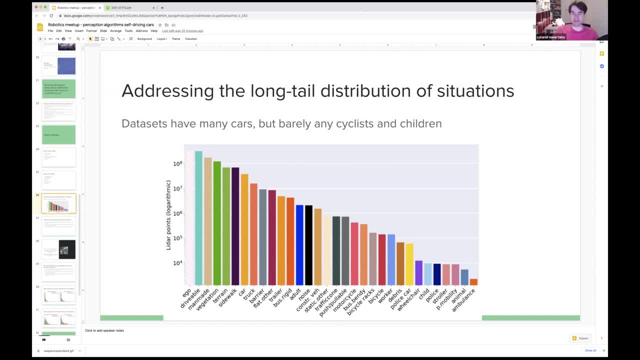 yeah, hopefully now people uh know each. yeah, hopefully now people uh know each other from the surviving car meetup or other, from the surviving car meetup or other, from the surviving car meetup or the robotics meetup. yeah, i think it's possible. yeah, i think it's possible. yeah, i think it's possible. um, yeah, 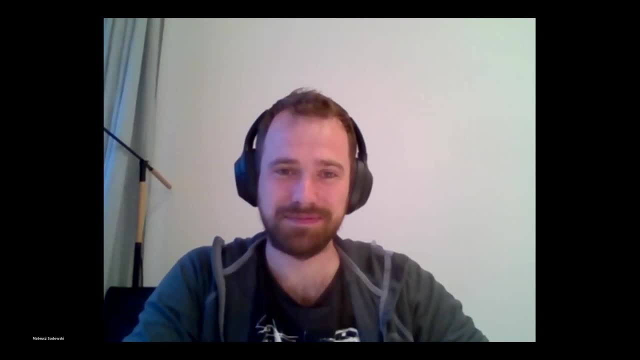 um, yeah, um, yeah, all right. so, uh, let's close, all right. so, uh, let's close all right. so, uh, let's close. thanks a lot and see you next time. thanks a lot and see you next time. thanks a lot and see you next time. thank you all for joining the discussion.